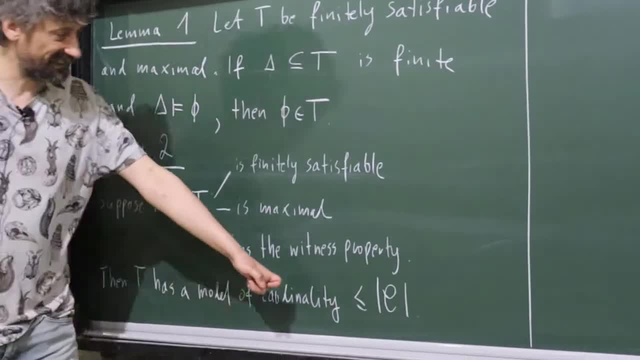 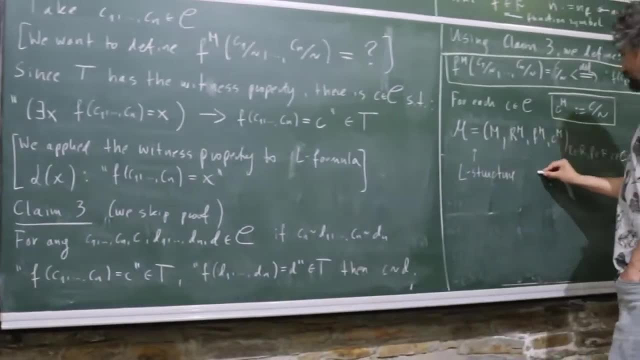 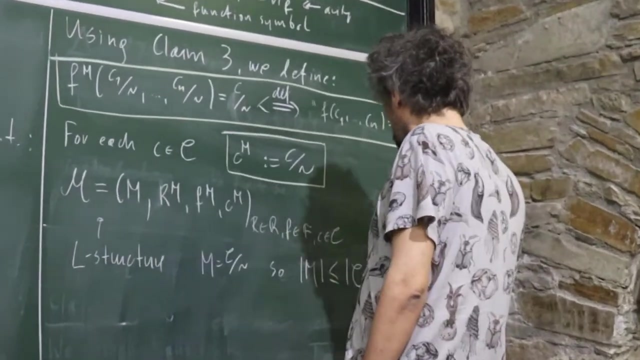 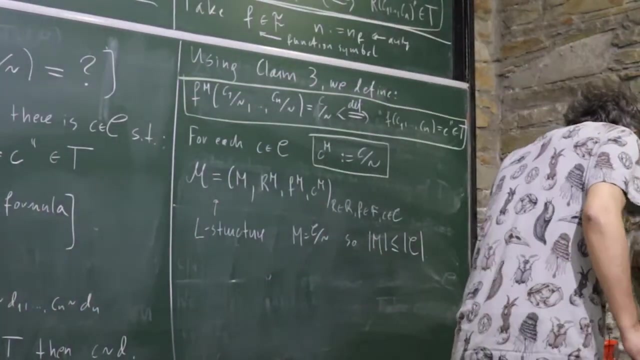 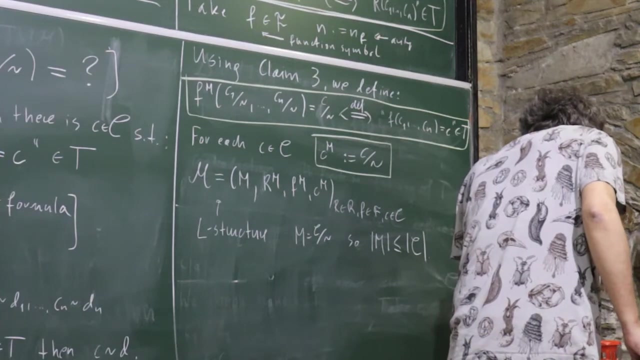 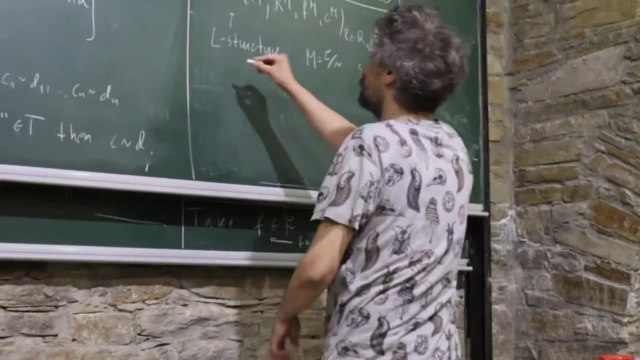 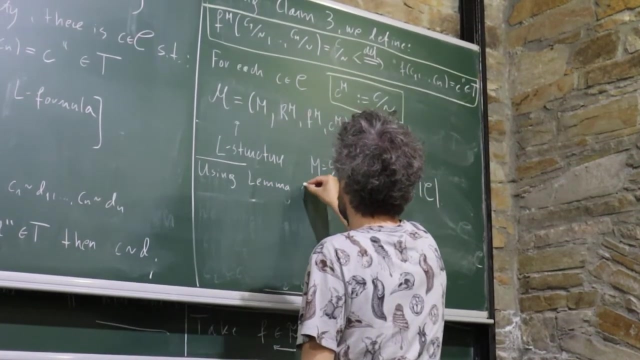 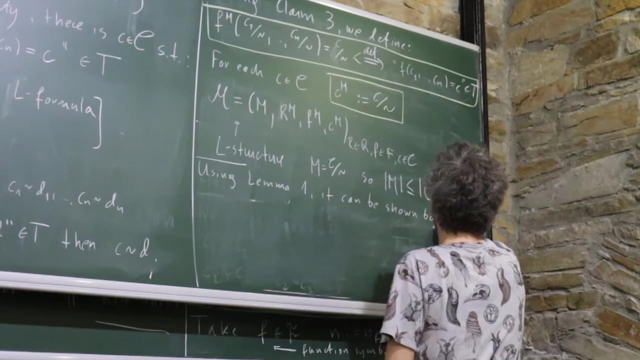 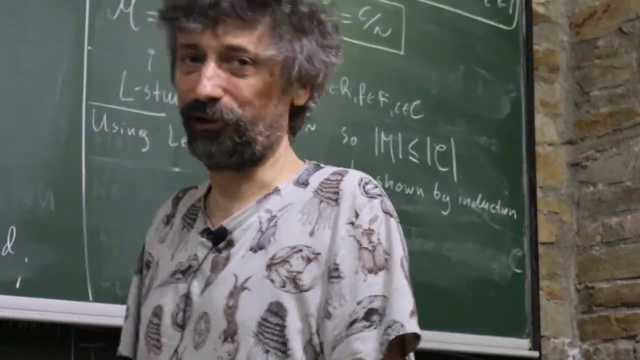 And now we want to say: obviously it has cardinality, at most this: it's a quotient, so M, so Okay, and now something I will not show, that it is Okay. So now this is a Glamour: 1 can be shown, but to do that by induction of complexity of formulas. but I 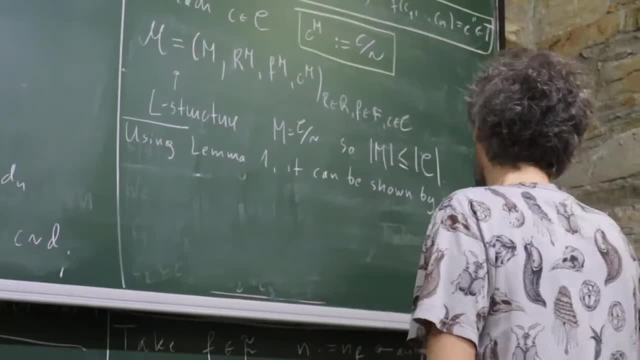 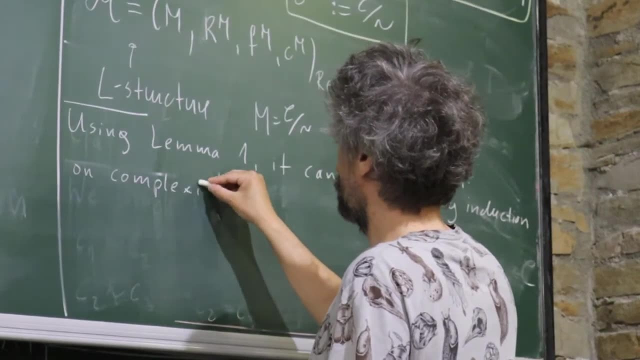 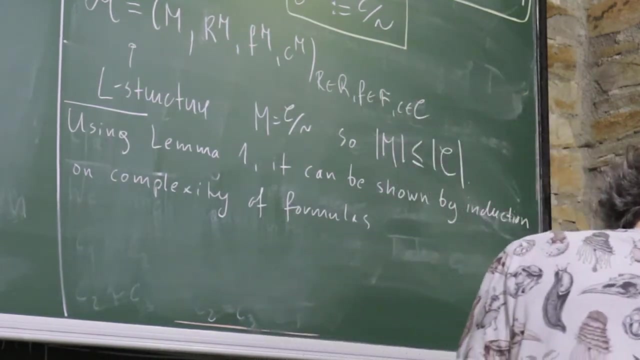 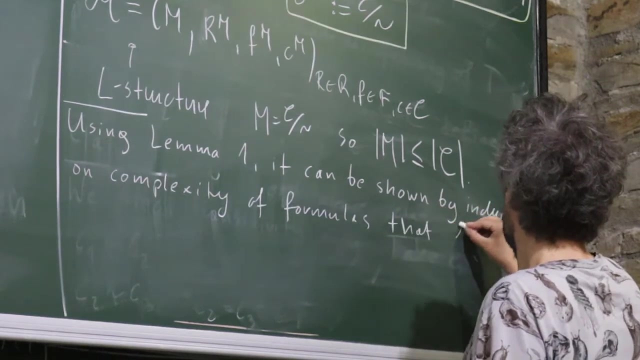 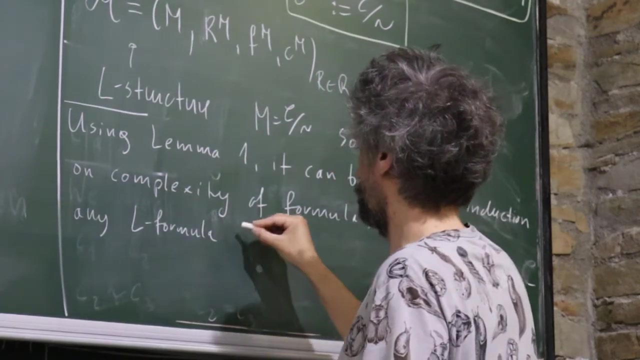 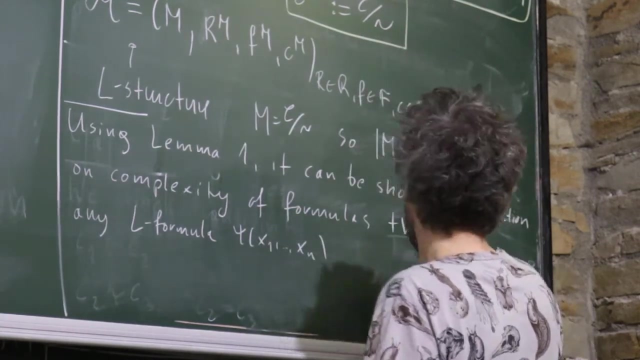 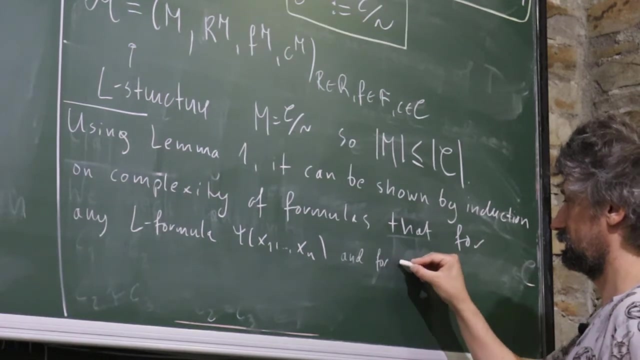 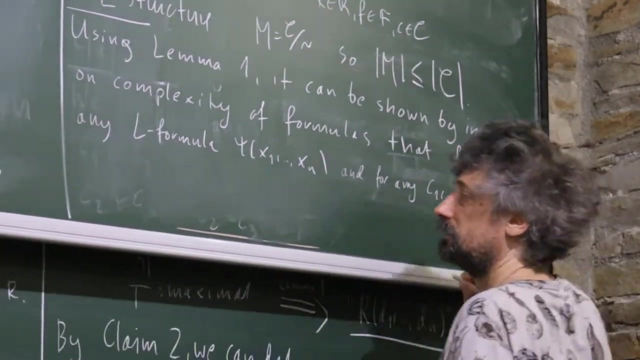 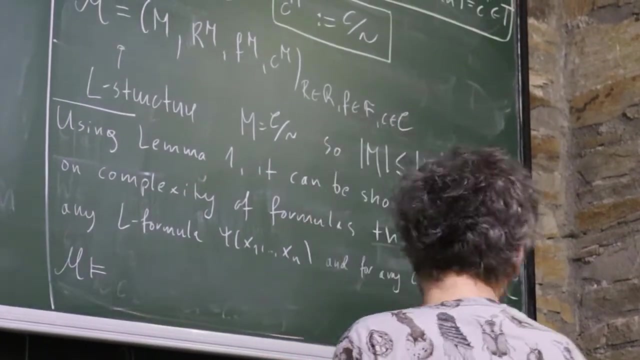 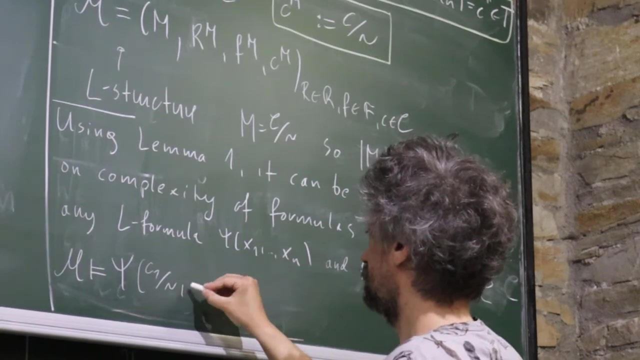 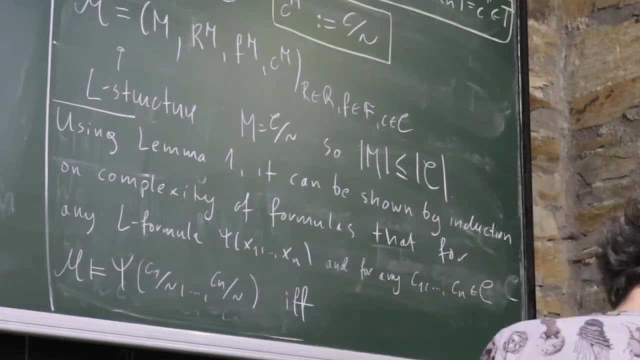 didn't define normally what is a formula, never. so I cannot do that induction on complexity of formulas. that for any L formula, let's say psi, x1, xn, and for any constant symbols c1 and cn, if we plug it it becomes true in this model if, and only if, this formula 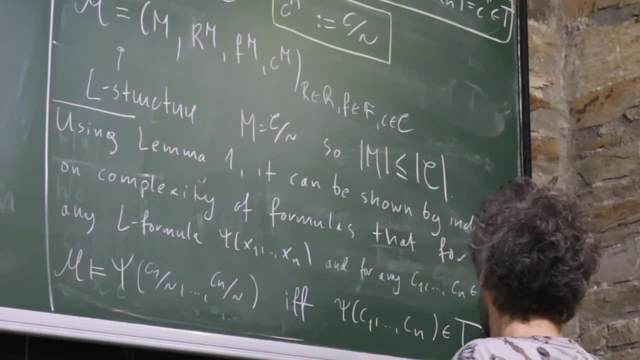 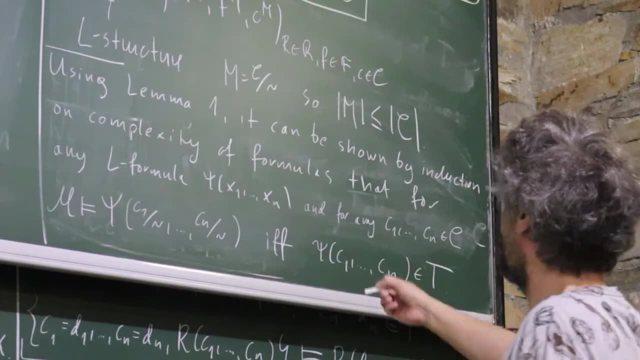 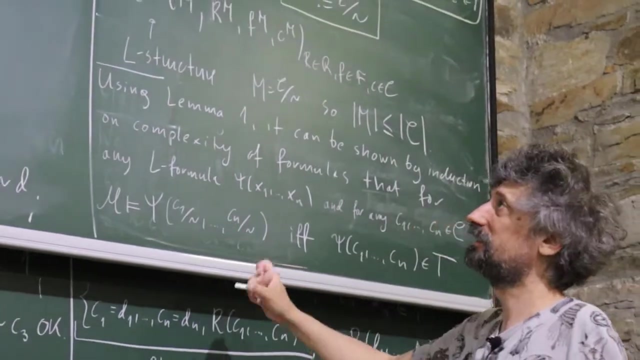 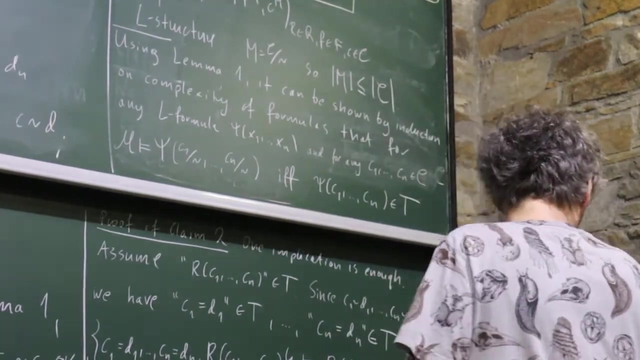 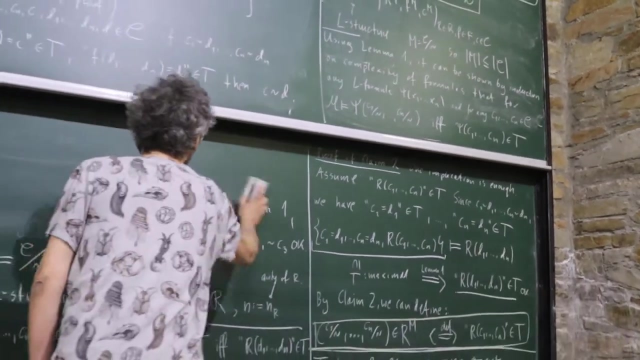 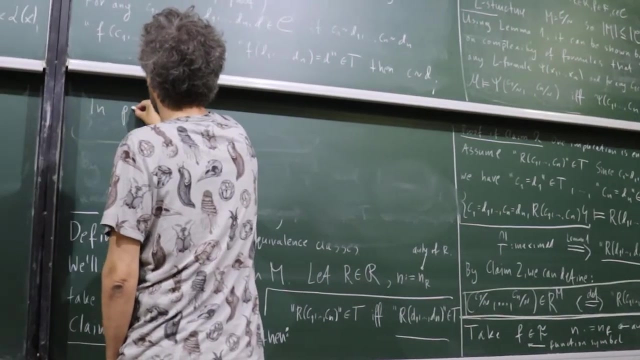 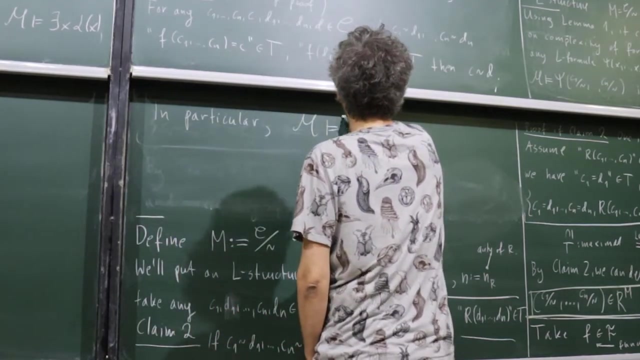 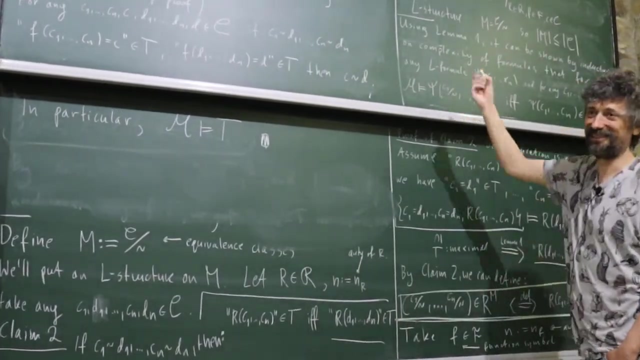 this sentence is in t. okay. so this: if we knew how to formally define formulas from less complicated to more complicated, then similar arguments as in claims one, two, three would show such a thing. but this in particular implies- and now the proof will be finished, okay so because kind of, if phi is in t, then already it is true here. 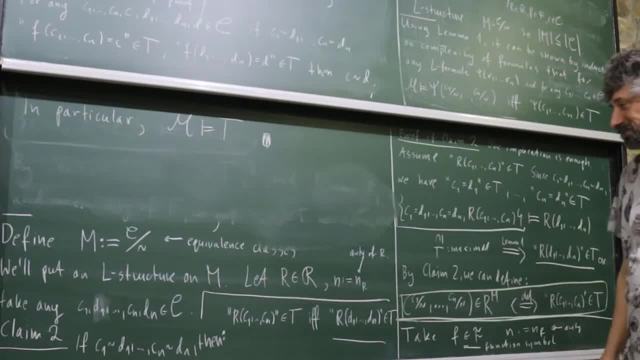 so kind of this part is skipped, so it may look at the end. so what I do on it, What I did honestly, was constructing the structure. but I didn't do the last part because that would, as I said, require formalizing all of this concept. what really is a formula? how? 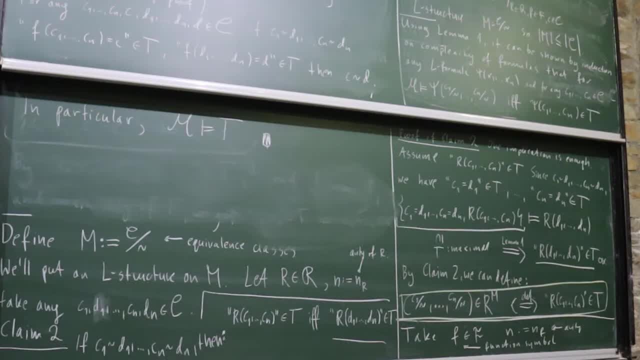 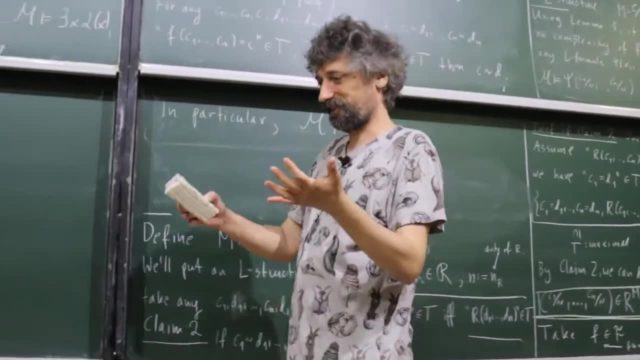 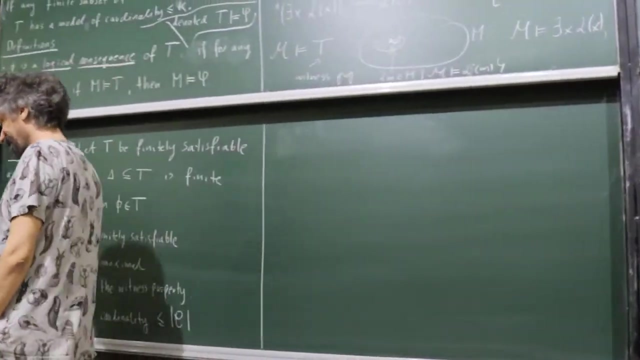 it is constructed from simpler formulas and in each level of construction we would have to show such an if and only if, which would be always kind of trivial but it would take lots of time. So here it is funny, but as I was discussing with Oslem in the break, here actually finiteness. 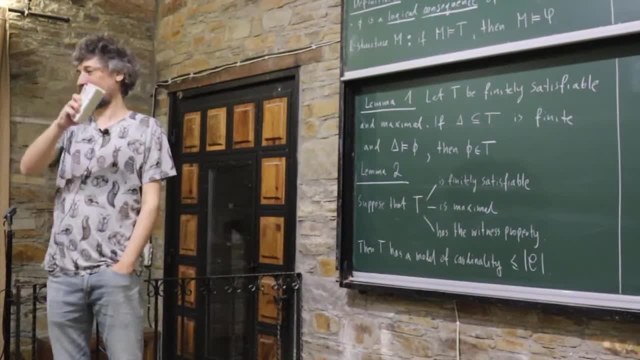 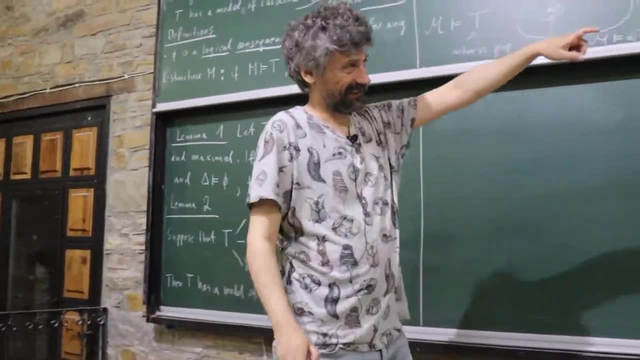 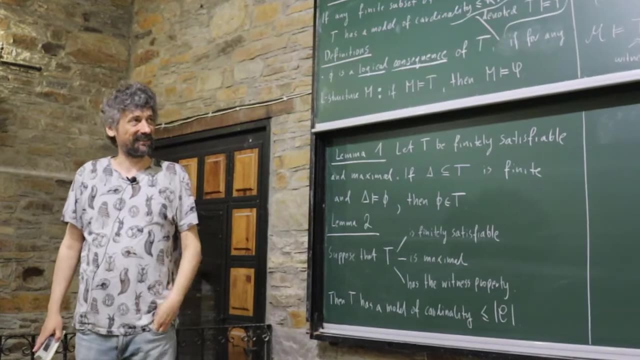 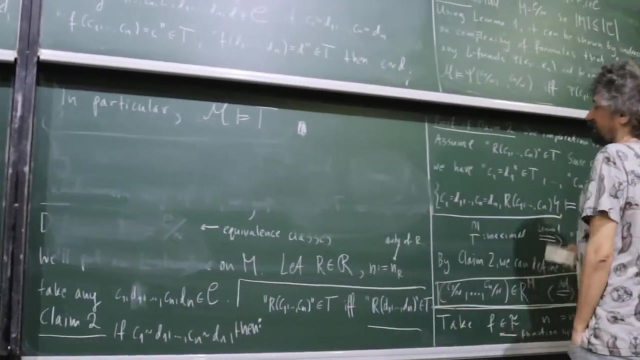 of formulas matters. if we would allow infinitely many, like disjunction or conjunction, we would need transfinite induction and this would break on the limit step. So kind of this is the reason. the finiteness here, or the compactness, works, And I'm fortunately okay, we may discuss a bit later. how would it break perhaps if we 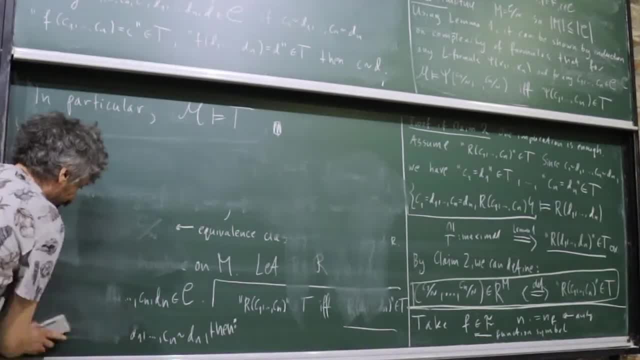 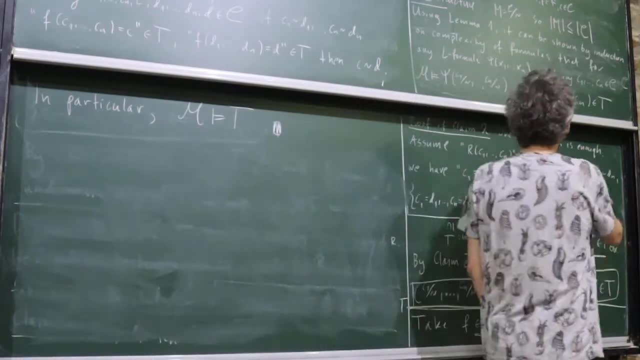 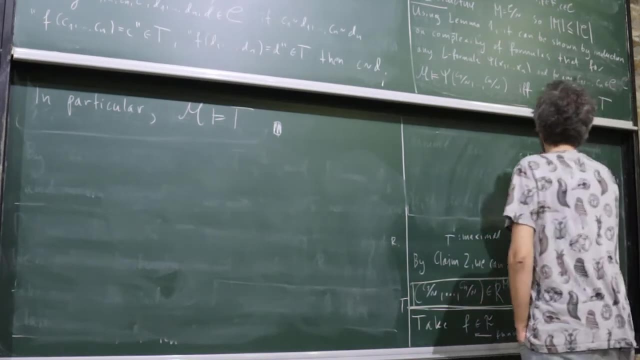 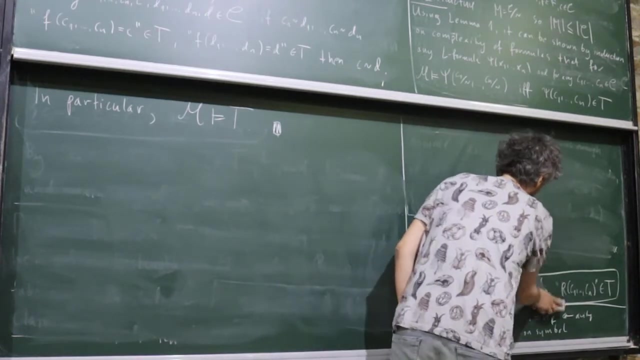 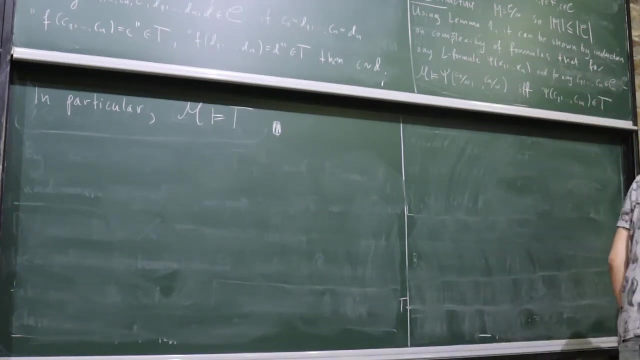 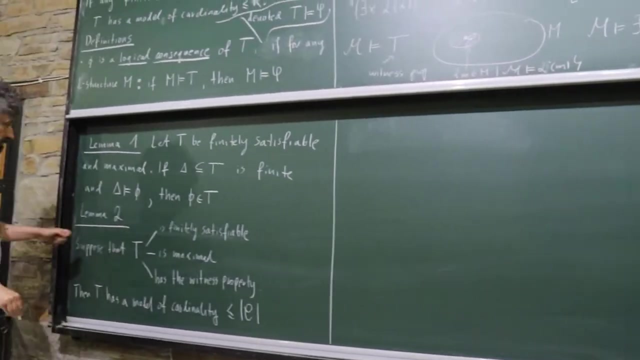 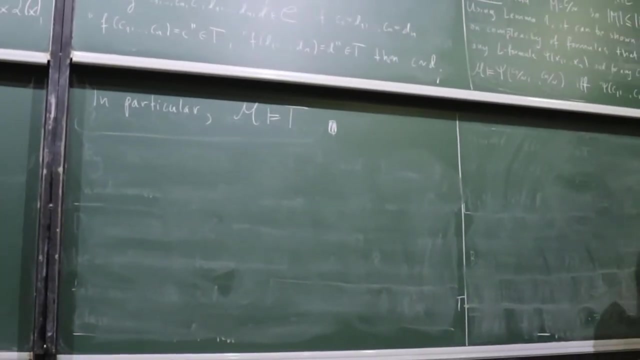 allowed infinite conjunctions, if you are interested. So now Lemattu is proved. Okay, so now from any theory, like in compactness theorem, we have to make it like this, so the whole proof is not finished. So Lemma 3.. So Lemma 3.. 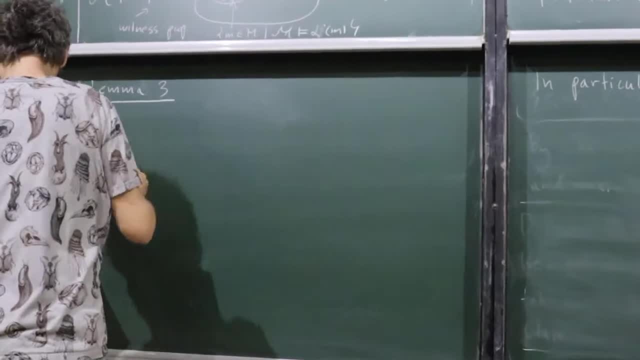 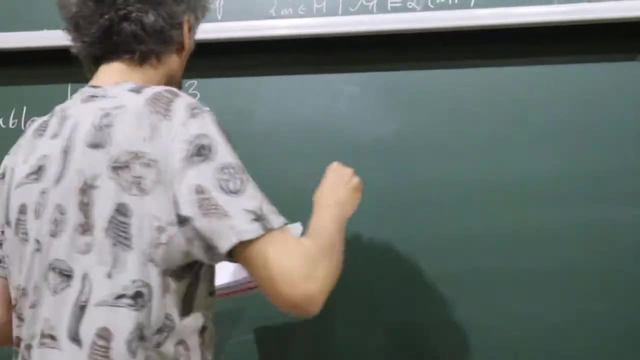 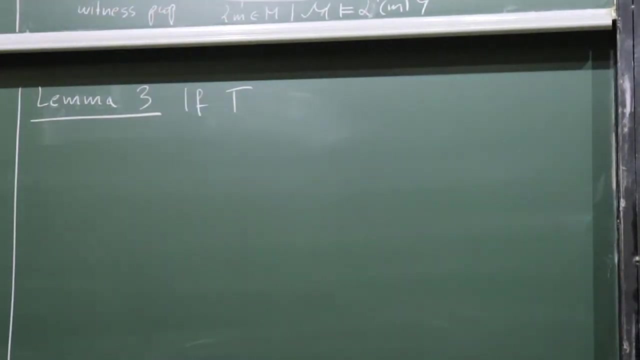 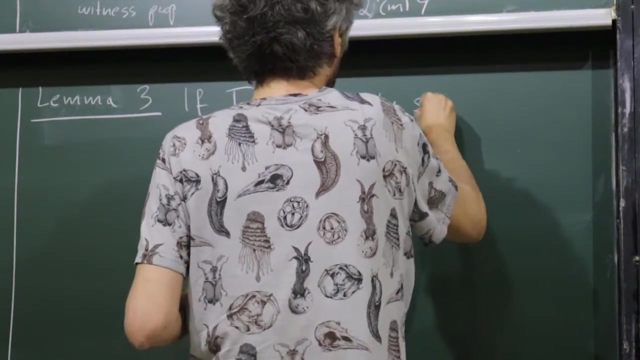 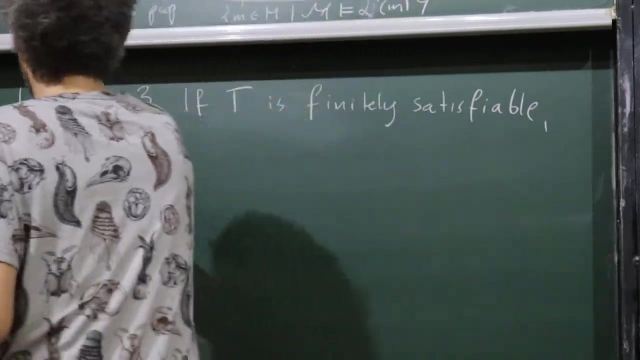 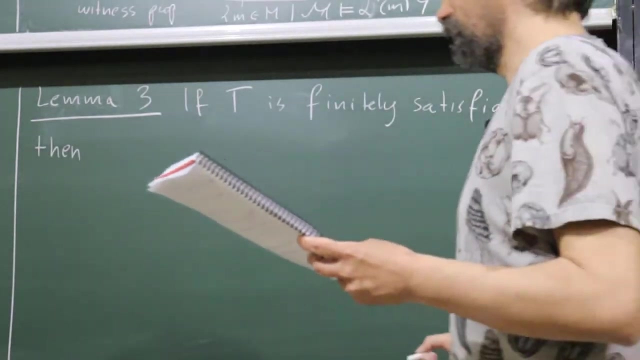 So Lemma 3. So now we force this witness property. So you see how to get this strange theory which has a witness property. So if t is finitely satisfiable, Okay, Okay, Yes, but to get this constants, we have to enlarge our language to allow space for this. 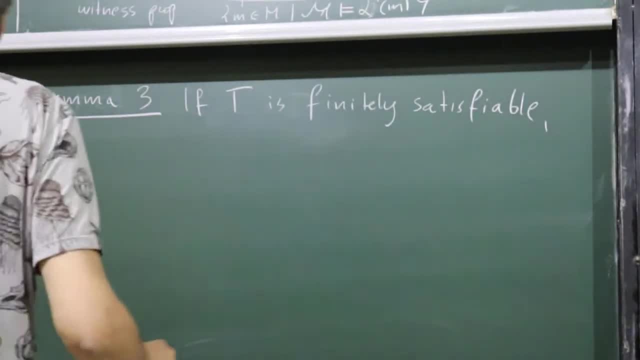 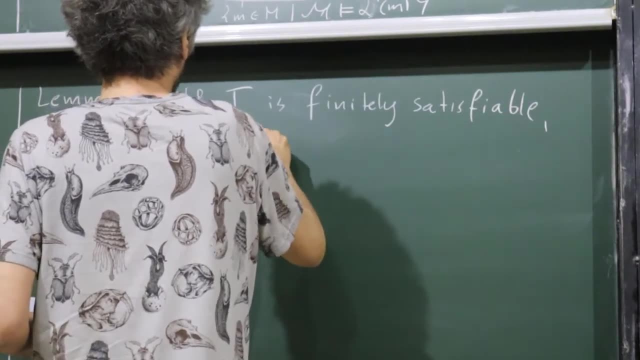 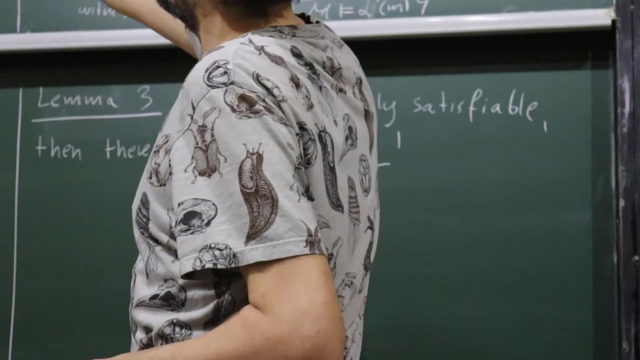 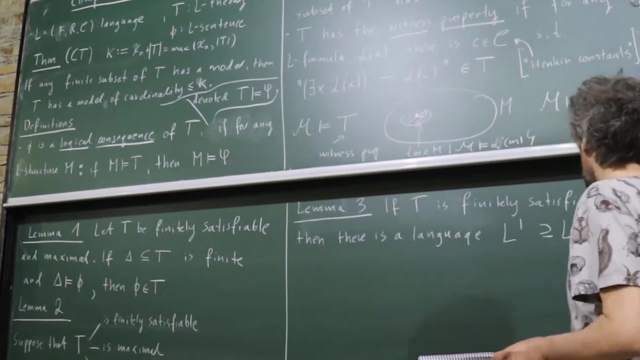 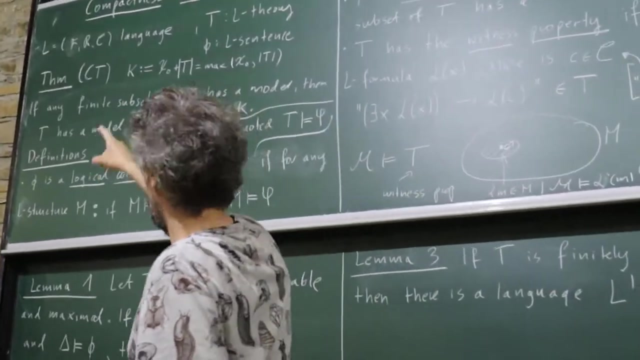 constants- it's like language of rings- would not be enough. Then there is a bigger language. so like f prime, r, prime, c, prime, everything is bigger. Actually, only constant symbols will be bigger. So this doesn't really formally means this. It means that all of the sets frc are bigger, are not smaller. 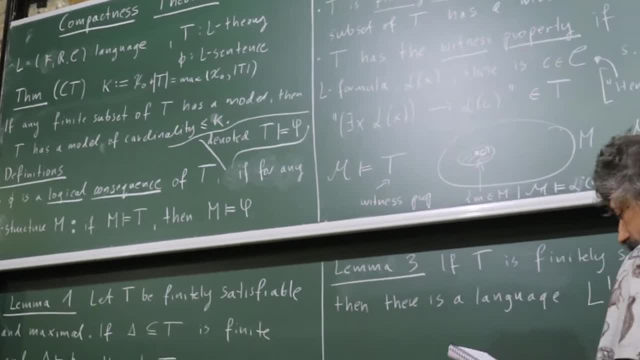 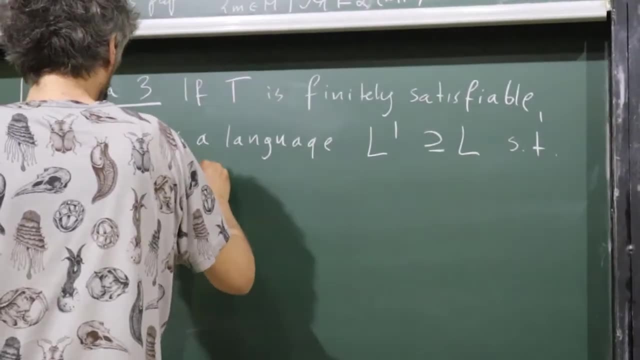 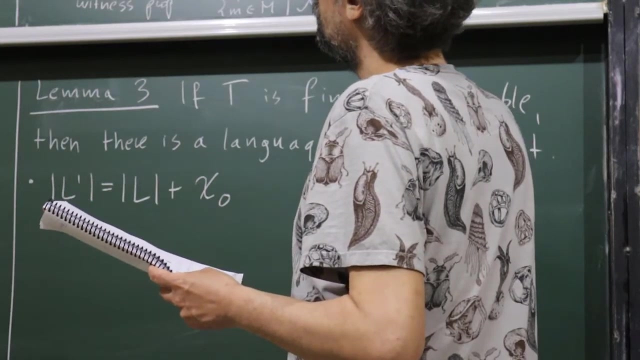 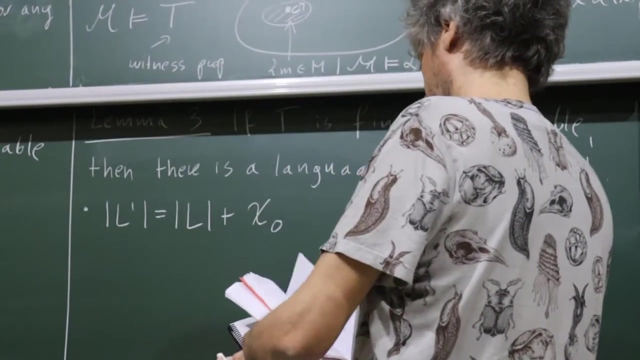 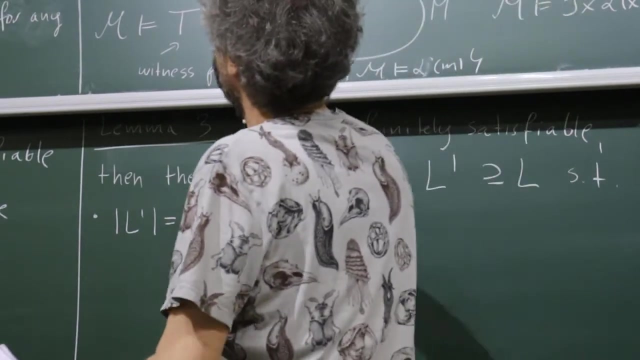 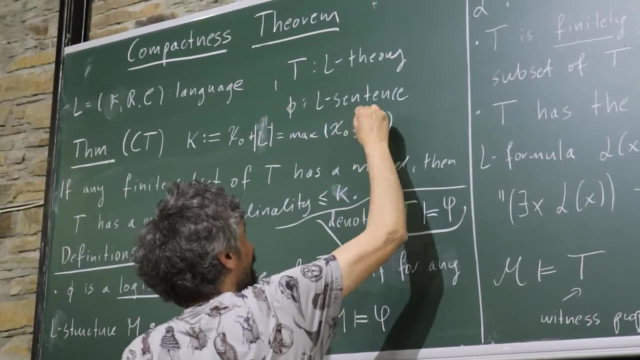 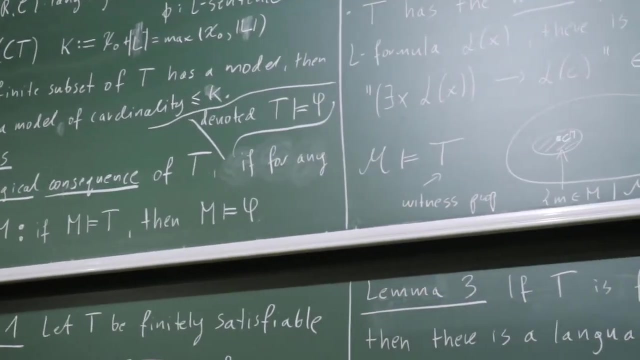 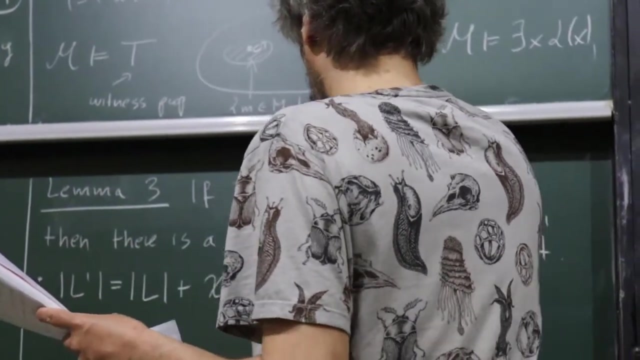 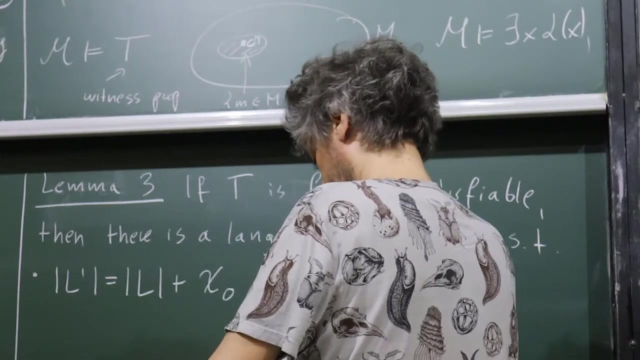 Such that Now cardinality is The cardinality Is: ah, actually sorry, I did not make much. still I think it should be L here, just maybe not. so here the language, especially since it comes like this here. so this is this kappa. so there is the speaker's language, and 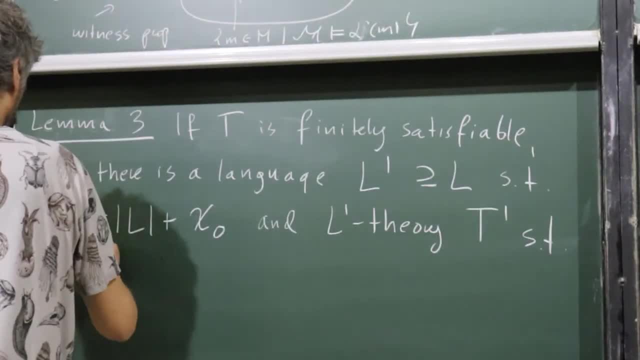 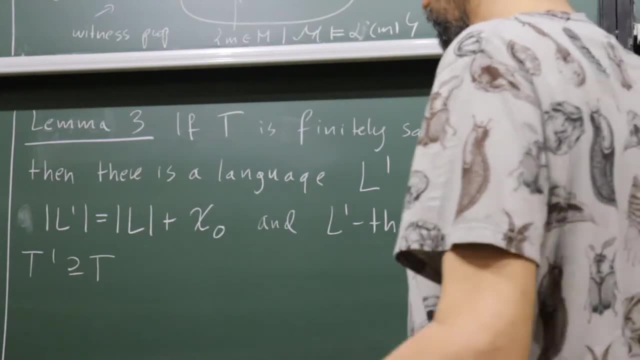 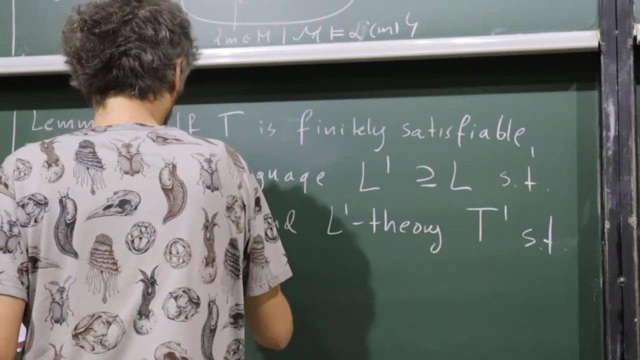 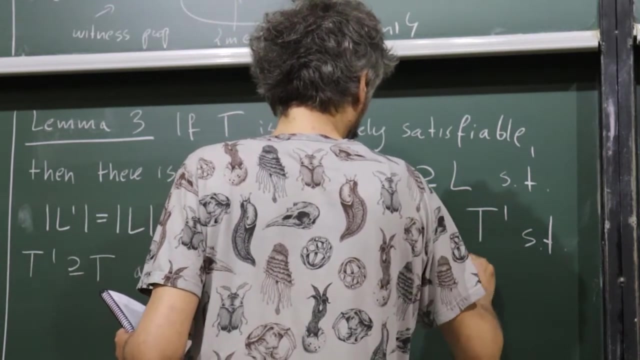 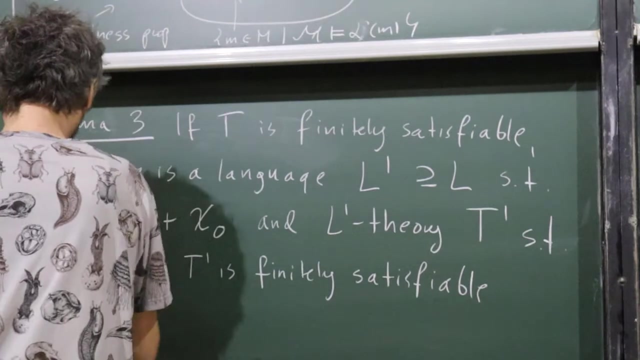 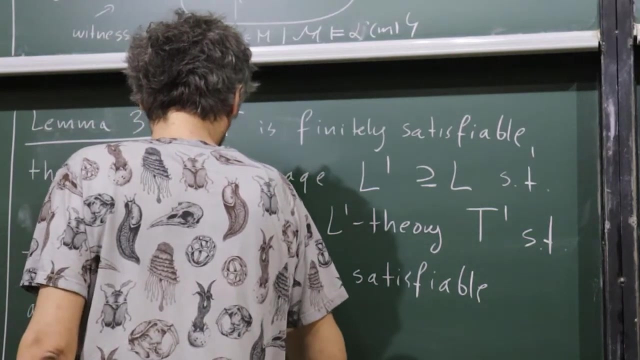 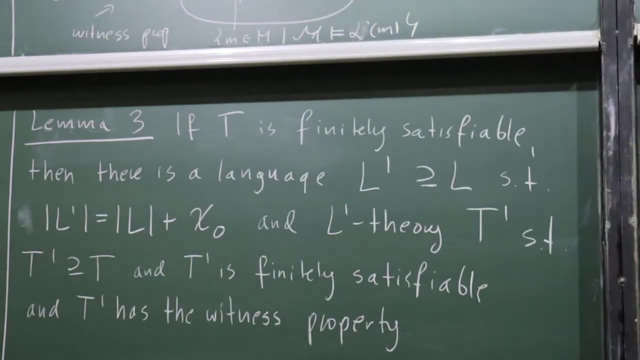 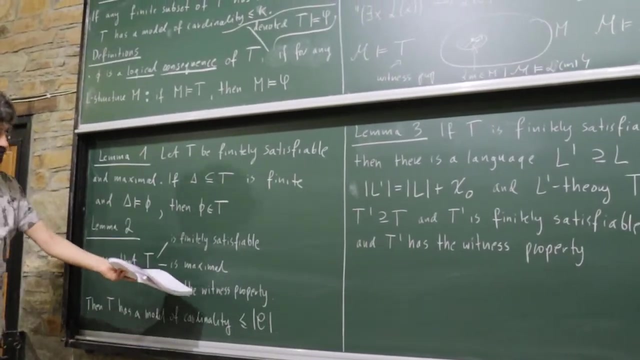 such that t prime contains the previous theory. so kind of each model of t prime can be understood as model of t and still t prime is finitely satisfiable but also has the witness property. ok now double t prime actually actually okay. so at the cost of enlarging the language we make a bigger theory from. 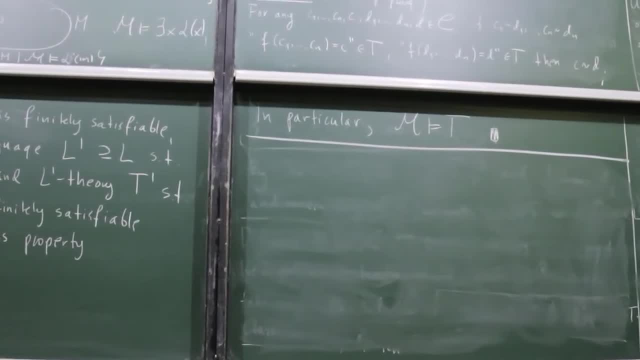 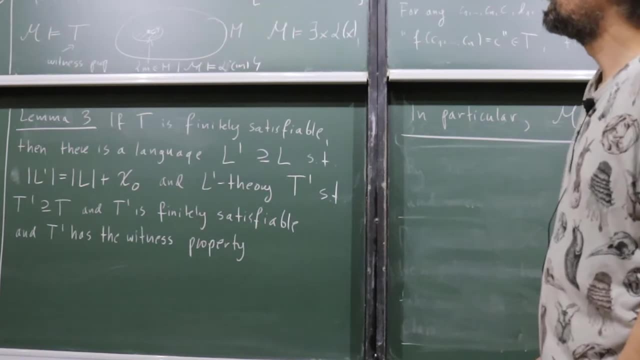 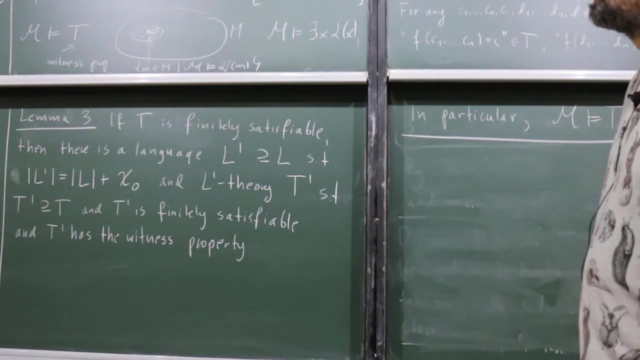 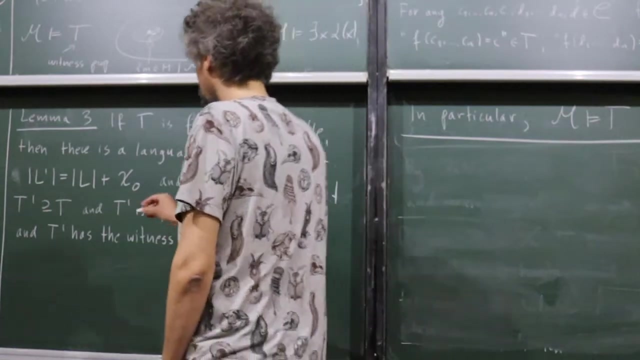 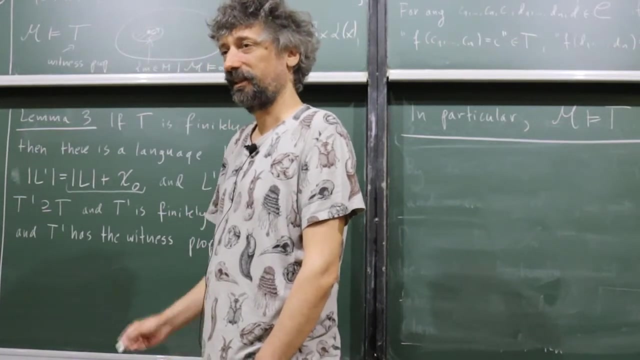 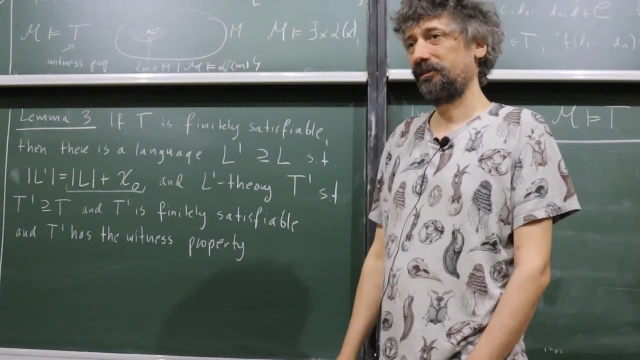 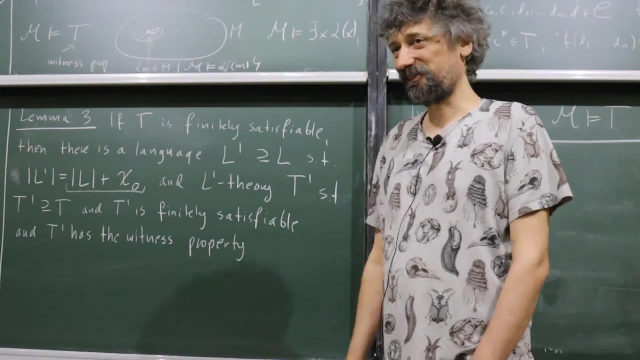 this original one which has the witness property. Now, actually I'm a bit confused, but at the end it should be like this: so okay, so this is definitely. this is the cardinality of set of formulas, as was actually mentioned before. so I think this is the right: all the possible formulas in the language, not necessarily if L. 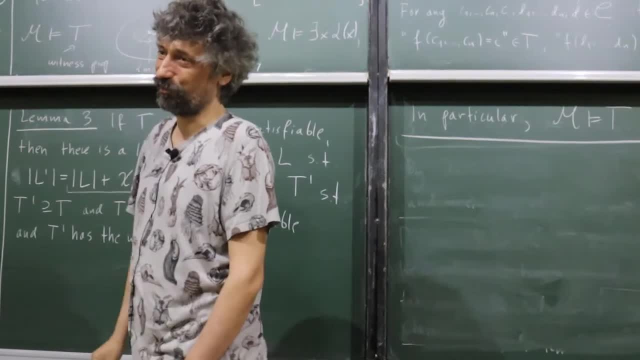 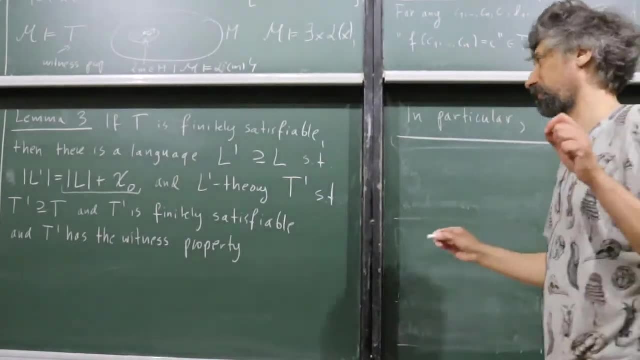 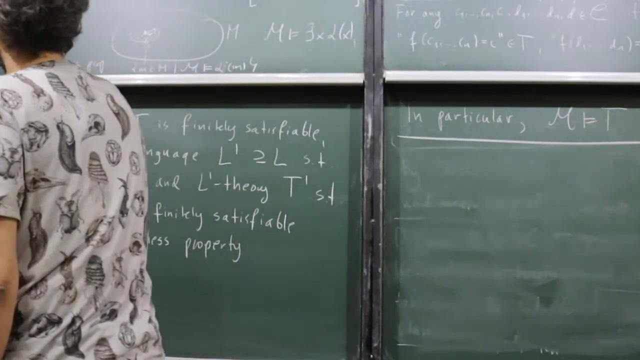 is uncountable and T is very, very small, then not. so this is a safe answer. This is a safer choice and I think this is this is the right choice, because we really wanted to say: really a number of formulas in the language, that's just a number. so I made here: yes again. 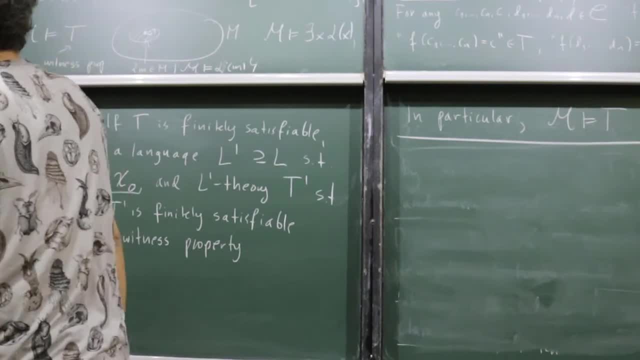 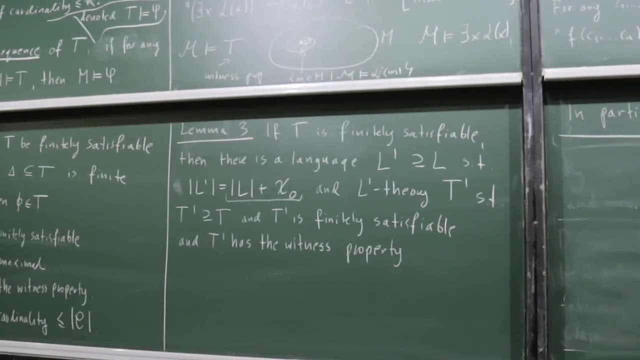 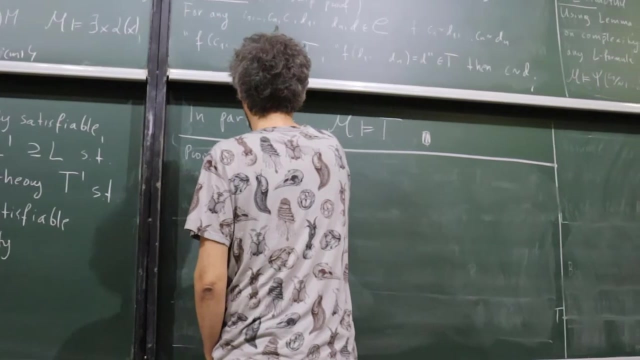 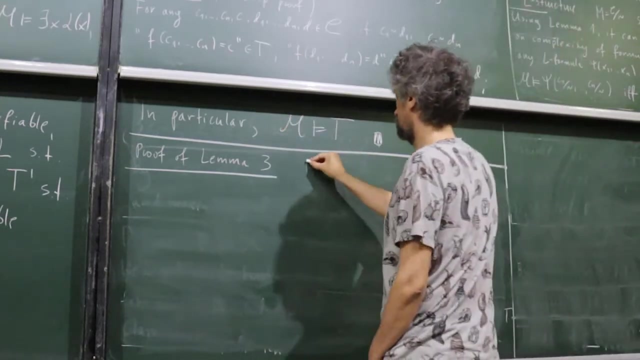 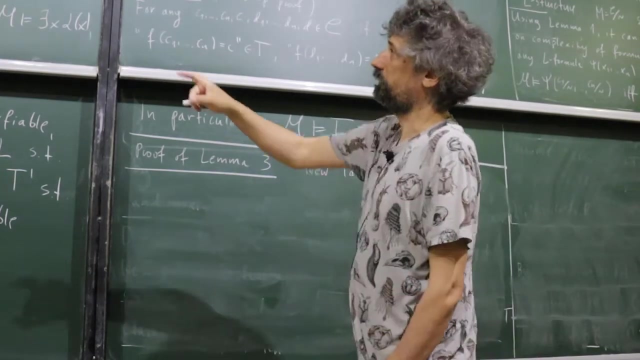 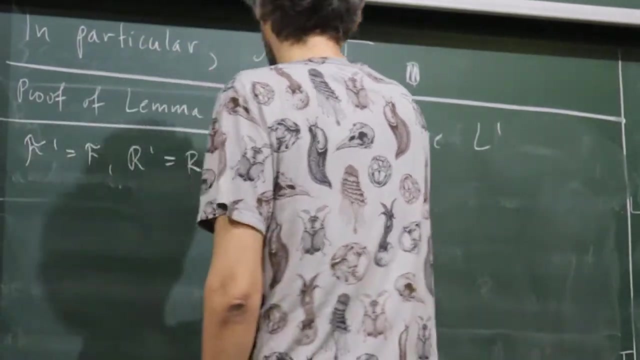 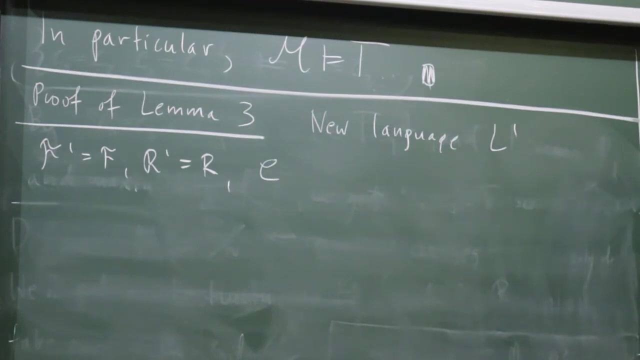 I mistake this. so doesn't depend on T. this number does not depend on T, depends only on the language. okay, so now proof of lemma 3. so what is this new language? so we don't change F and R, but C prime we do. ah, okay, it's not L prime, sorry, it's an L1. it will be L1 and L1 is the same as L1, so it's an L1, and L1 is the same as L1, so it's an L1 and L1 is the same as L1. so it's an L1 and L1 is the same as L1. 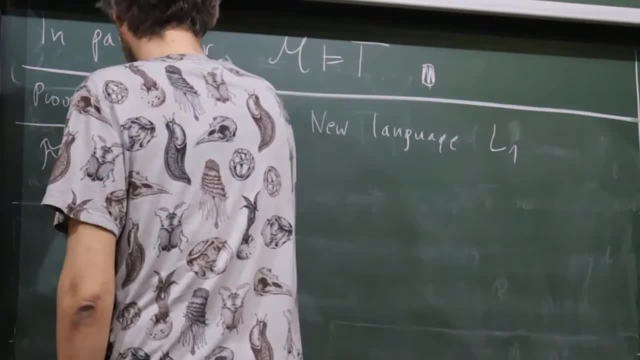 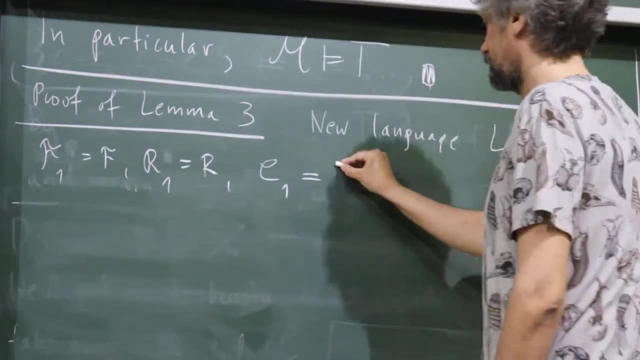 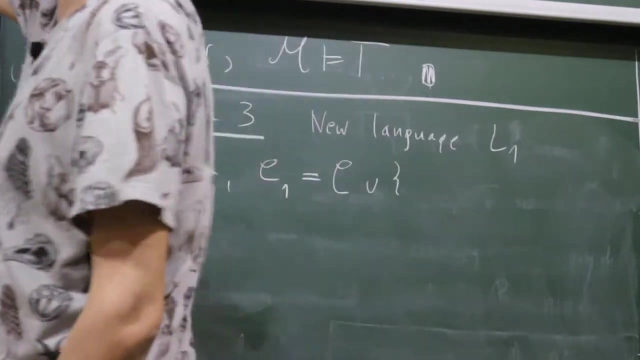 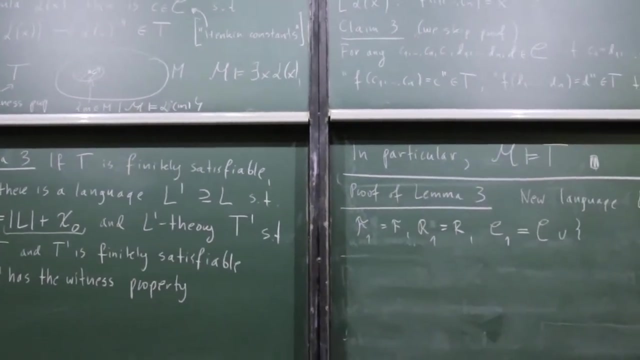 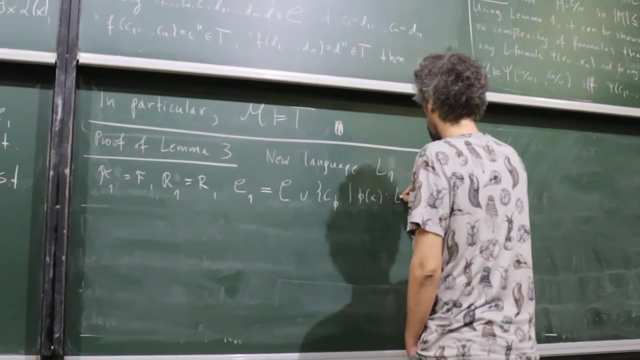 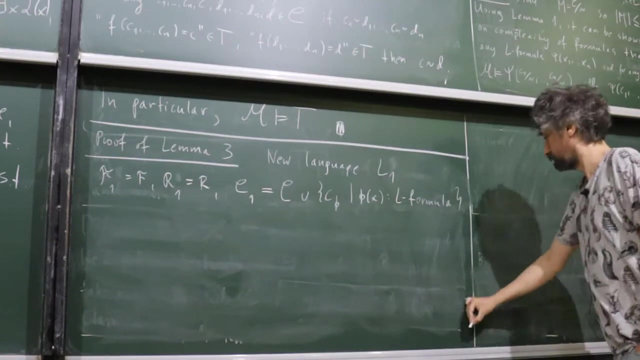 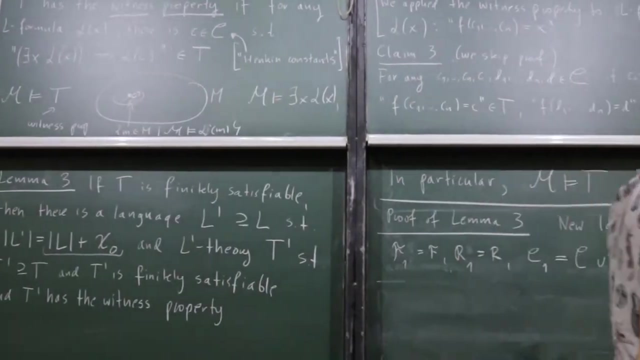 infinite process of new languages. so this is how it happens: we take all constants and for each formula like this, we add a new constant symbol. so it's a formula with one free variable. so now, this was this moment that for all formulas we artificially added constant symbols. so 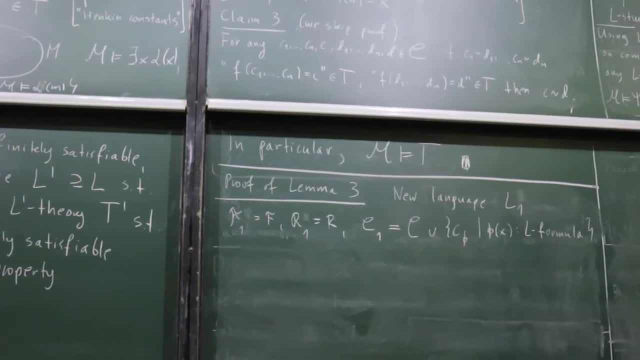 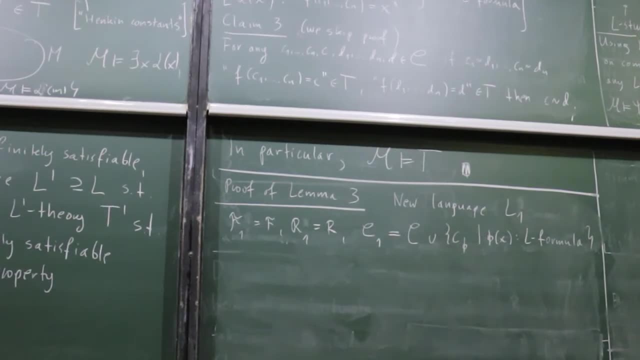 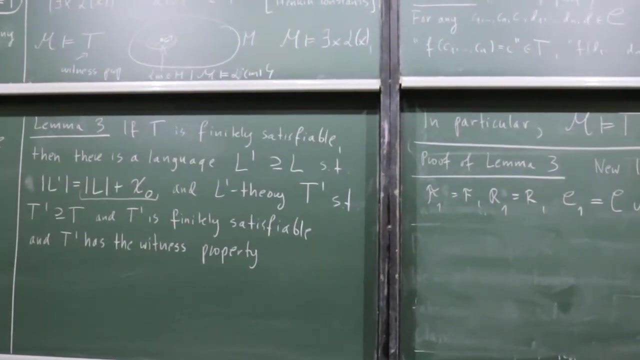 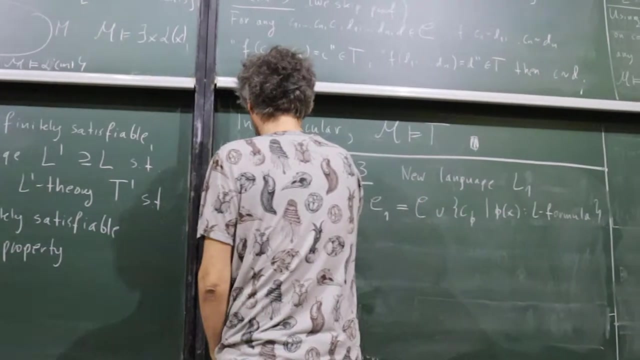 we add a new formula, but still we have to define this theory and we have to make sure it is still finite, satisfiable. so t1, and this is just what it should say. so t1 is t. t1 is t plus all the. 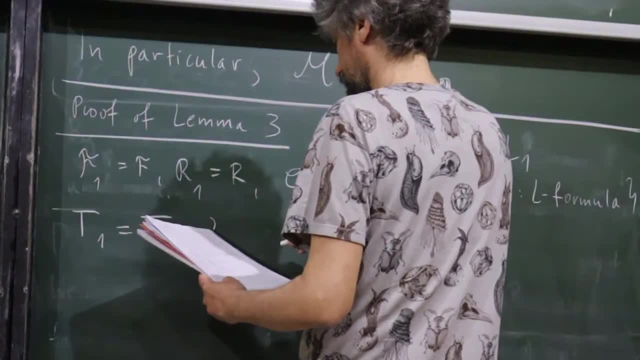 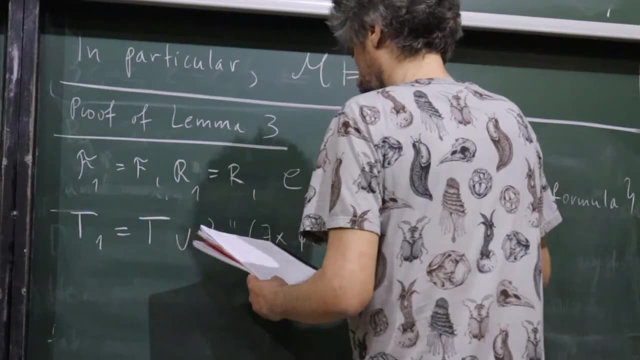 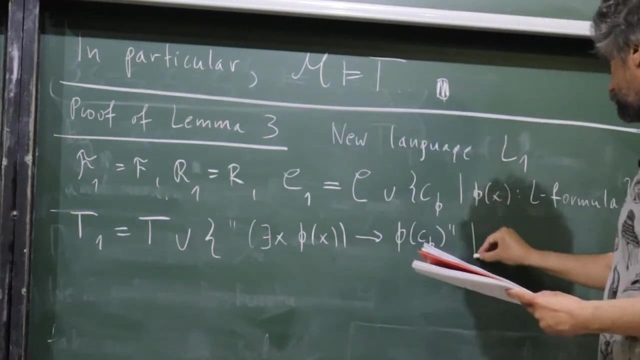 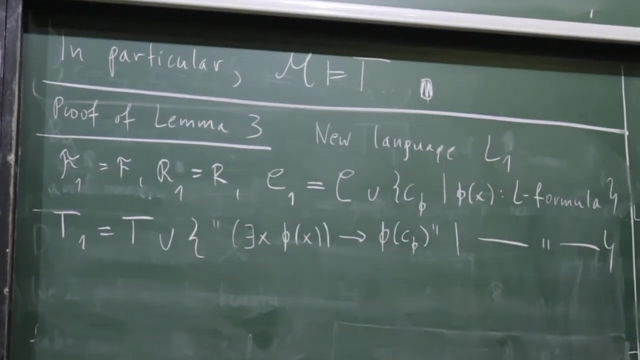 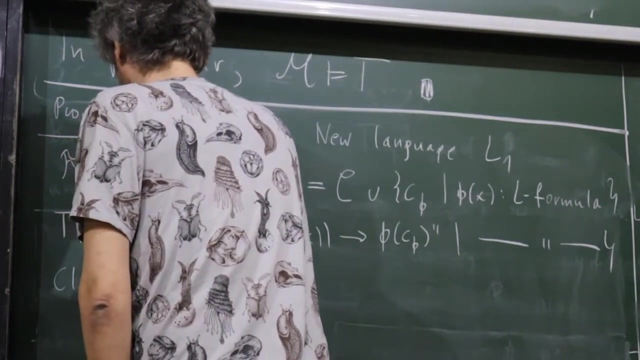 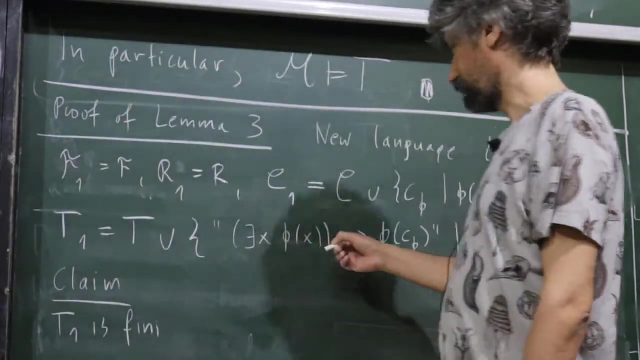 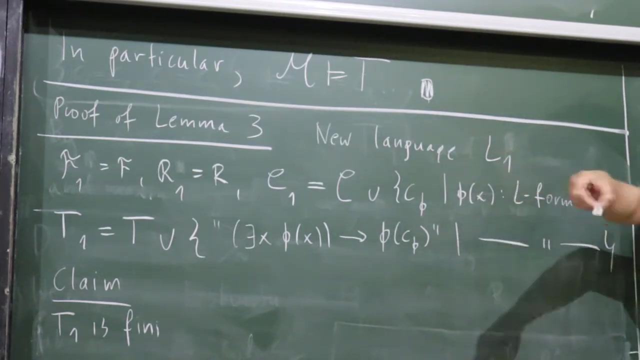 t1 is t plus all the from the witness property. so phi, c, phi. So now we should check it is really finitely satisfiable And note: this does not have witness property. it has witness property with respect to formulas from old language. that's why we would have to repeat the process. 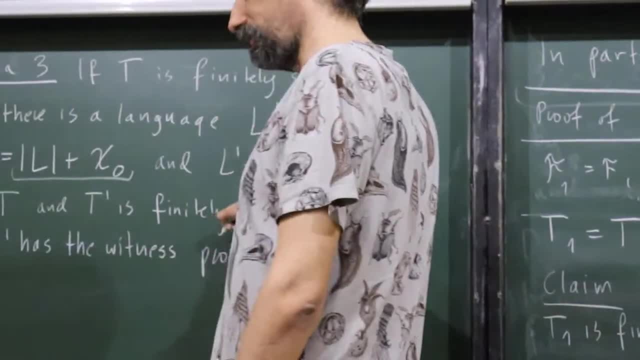 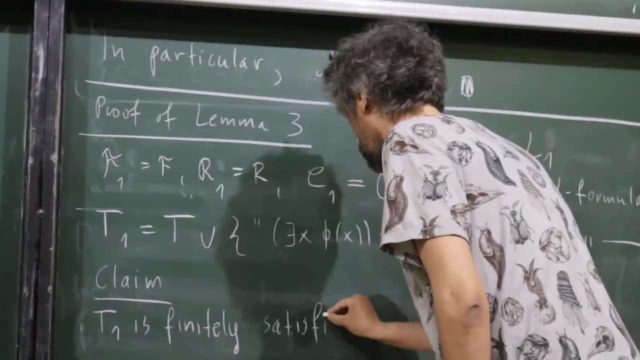 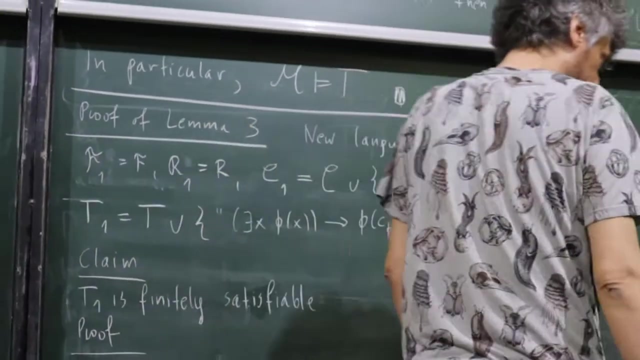 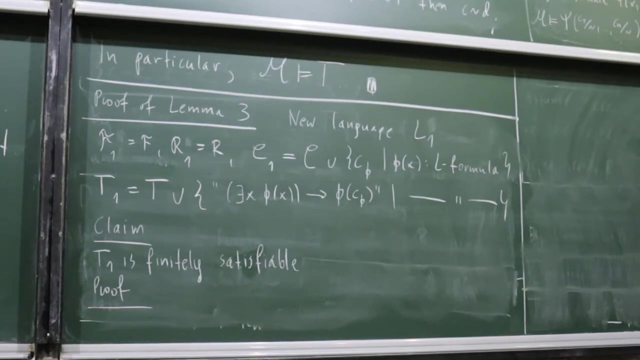 But of course we will be totally dead If we lose finite satisfiability on the way. so this has to be checked. so proof of claim. So now again, we would have to find some model. So take, So now again, we would have to find some model. 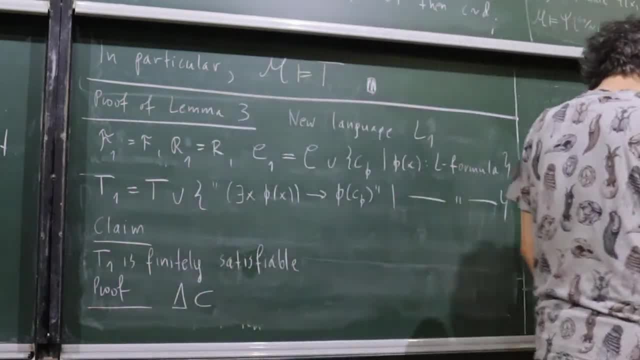 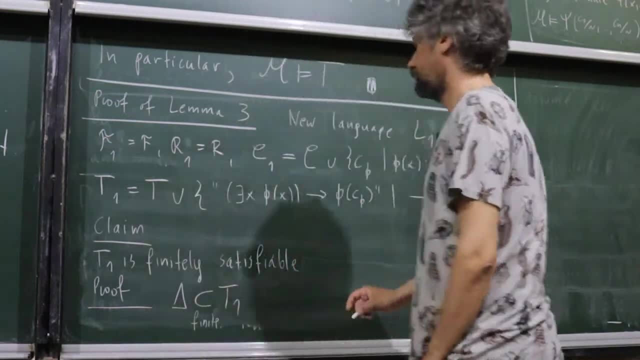 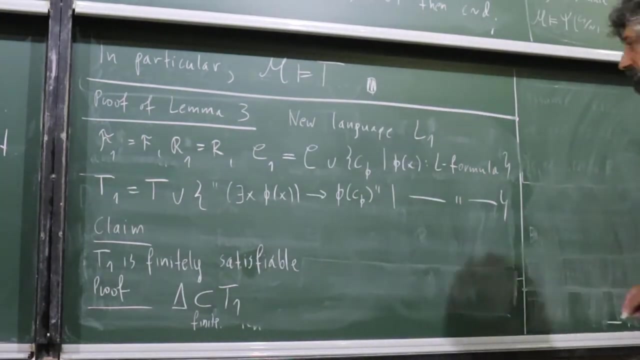 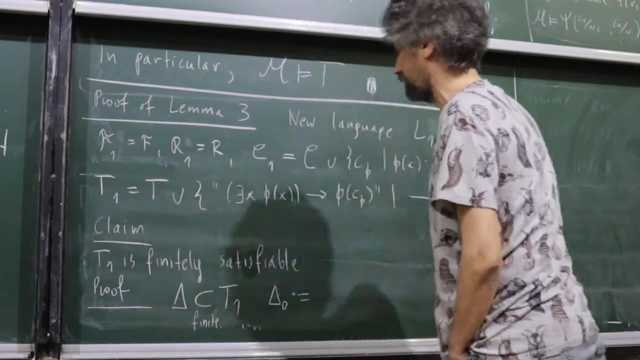 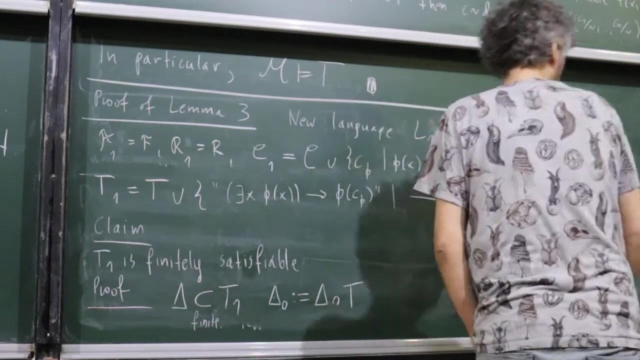 So take. So take this partial, okay, partial, in T1 finite. So T1 comes from T and it has this: new sentences. So let delta 0 be the part coming from capital T, maybe empty, maybe not, Okay, Okay. 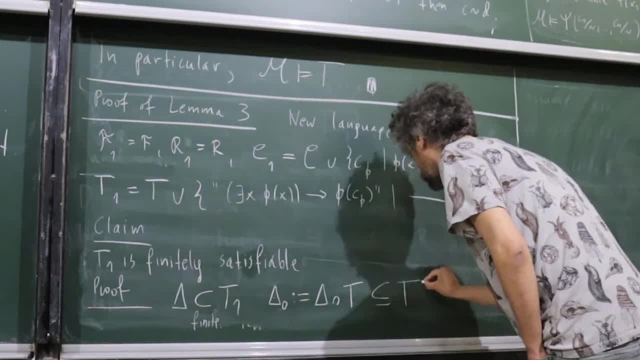 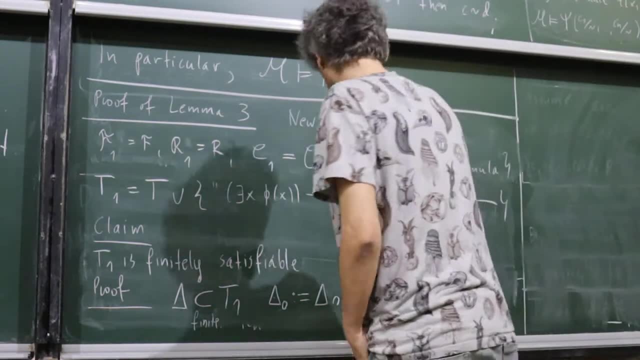 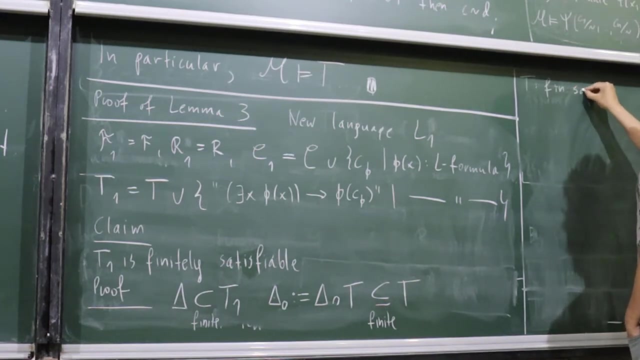 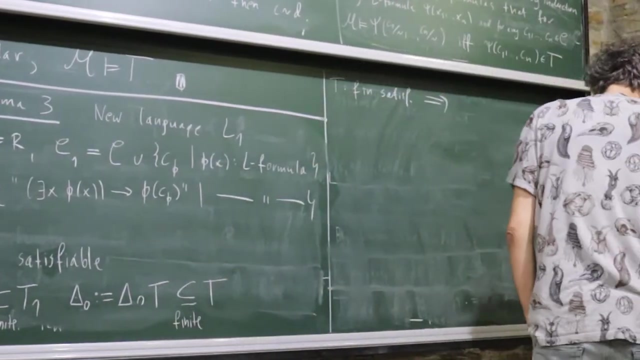 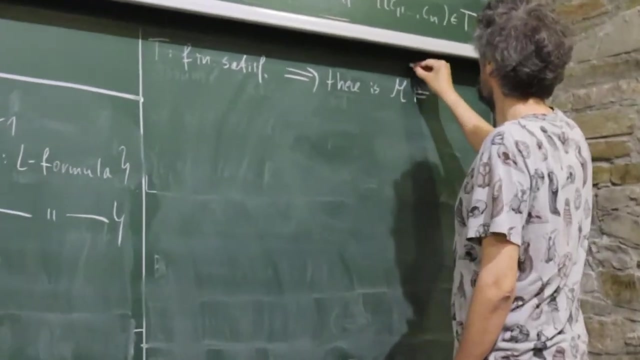 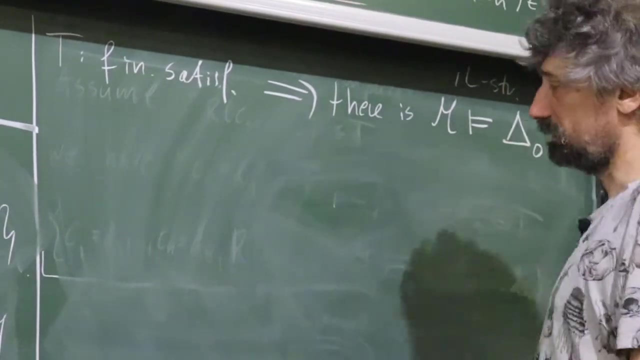 Okay, So delta 0 from T is definitely finite because it's a subset of something finite, So this has a model. T is finitely satisfiable, So this finite subset of T has a model. Okay, Okay, L structure M, which is a model of this delta 0, and we want to expand it to make it a model. 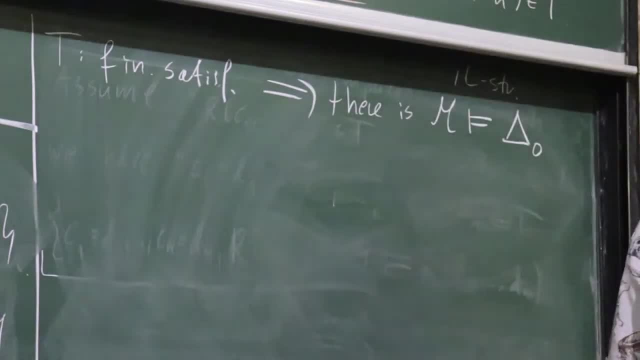 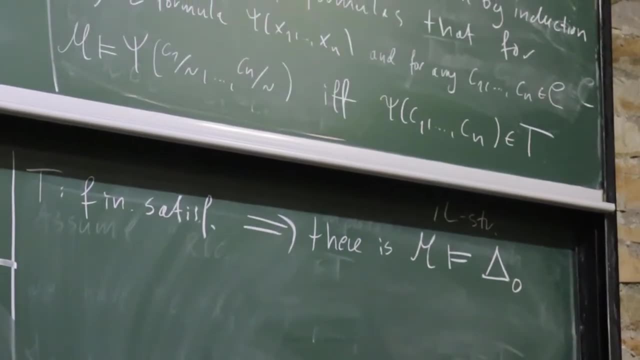 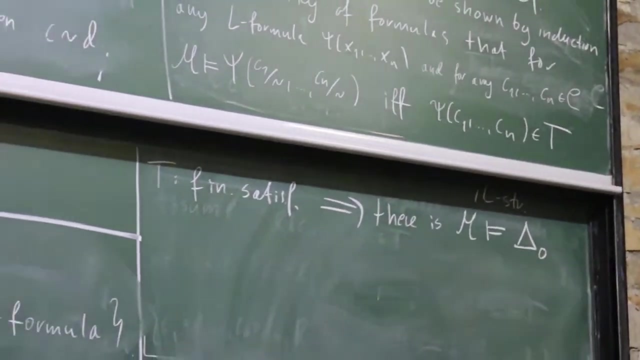 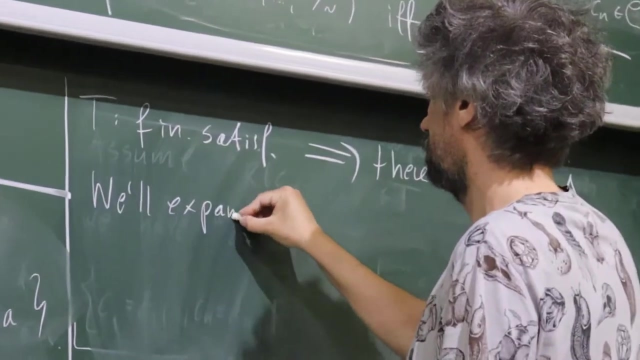 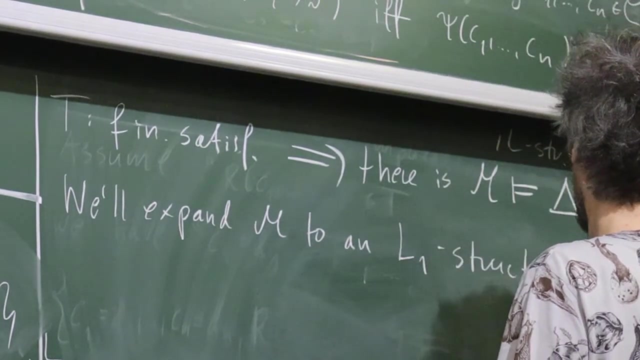 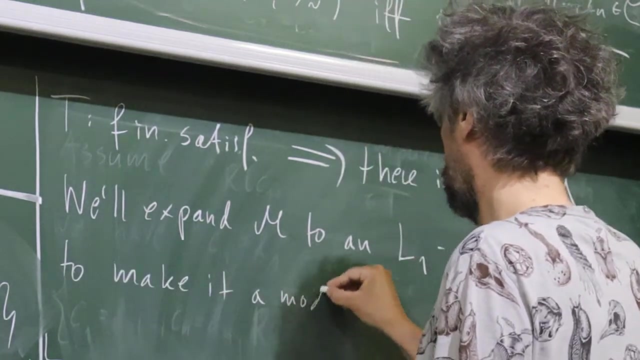 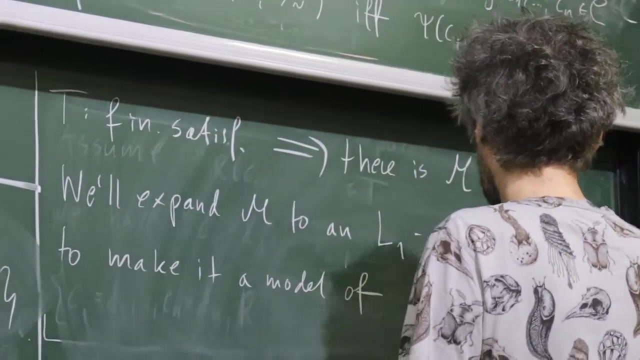 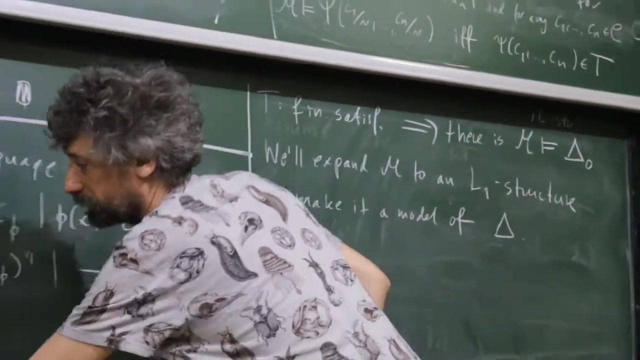 of delta. so now, what? so? actually, we will even, I think, make it model of delta 0 and all the sentences so for any, okay. so we will expand M to N L1 structure to make it a model of this. okay, but as I'm saying, I think already it will be model of delta 0 and all of this in particular. 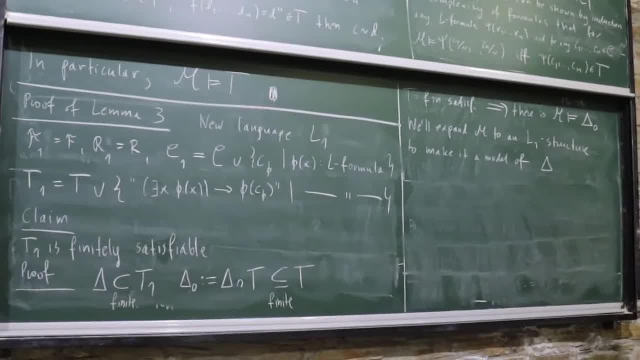 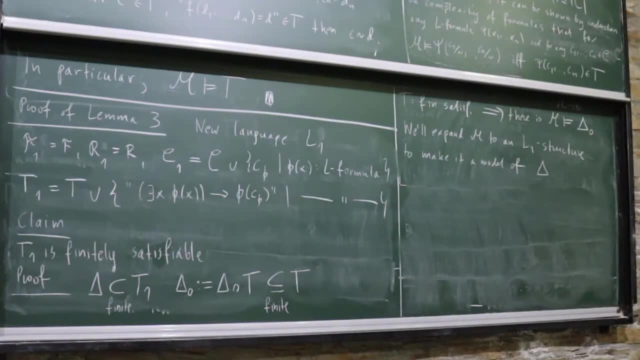 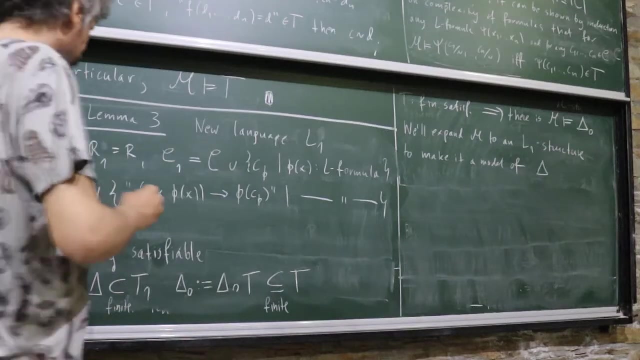 of this. so to expand it, we have to find interpretations of all these new constant symbols. sorry, in the definition of delta 0 you say delta composition T. what is the meaning of delta composition T words interesting. No intersection. this circle didn't become a circle, it's. 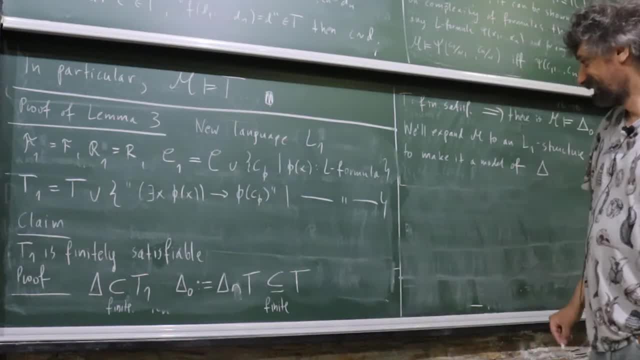 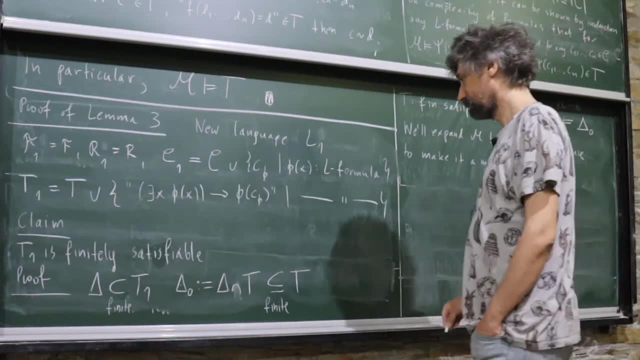 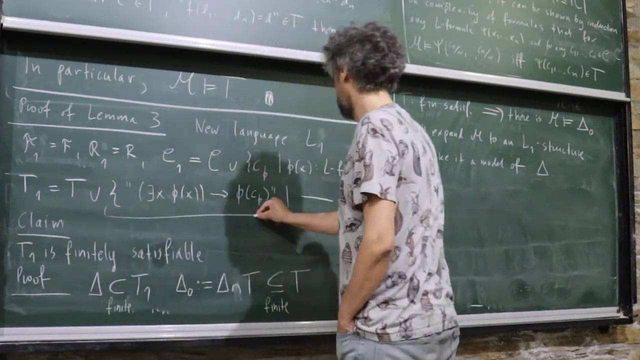 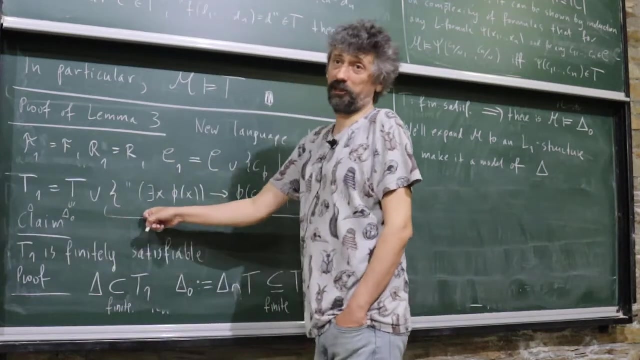 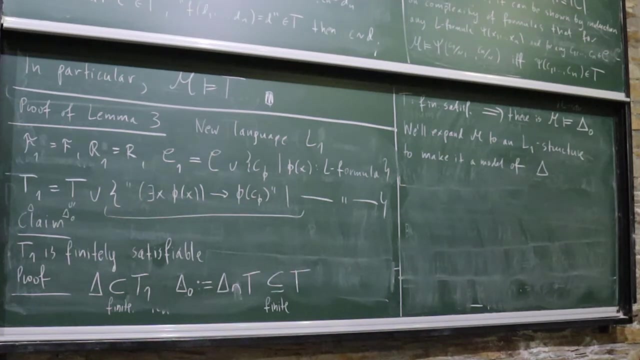 this is a circle intersection. intersection just a part of, as I was saying, a part of this. delta is here, So it's delta 0. So this delta 0.. so delta zero is here and maybe there is some rest here. okay, okay, expand it. 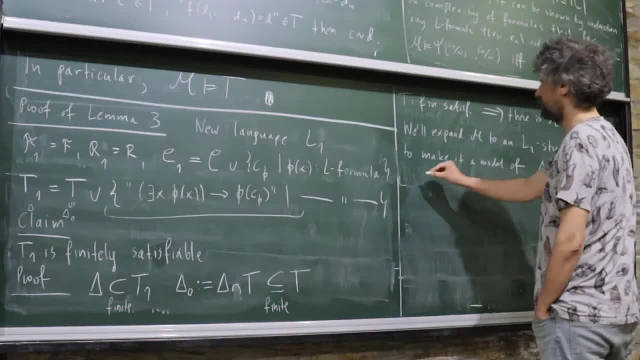 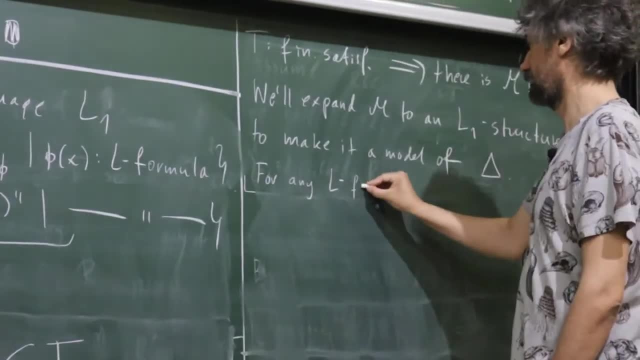 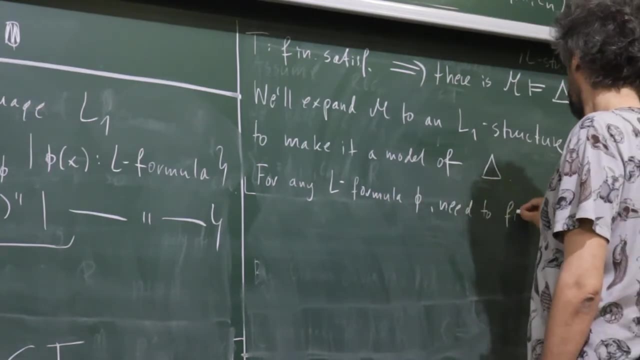 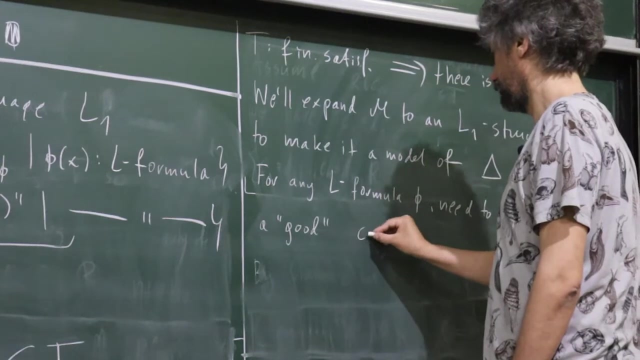 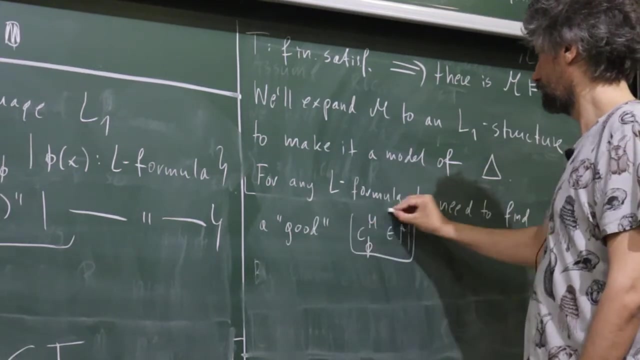 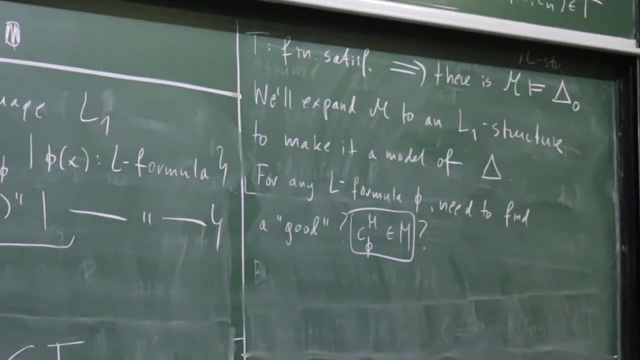 so for any l-formulapsy like this, we need to find good c phi interpreted in m in m. so what will it be? so we just look, there are two, there are two options, so if it may happen. so now we really give a meaning to. 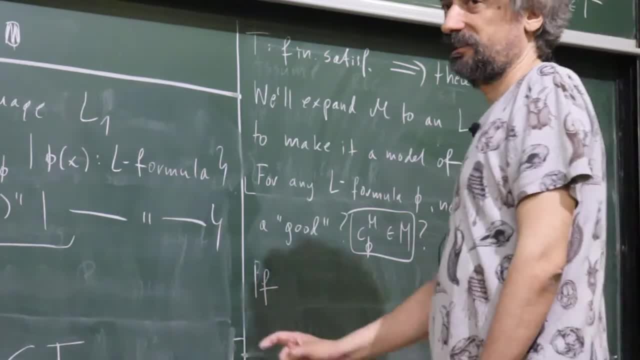 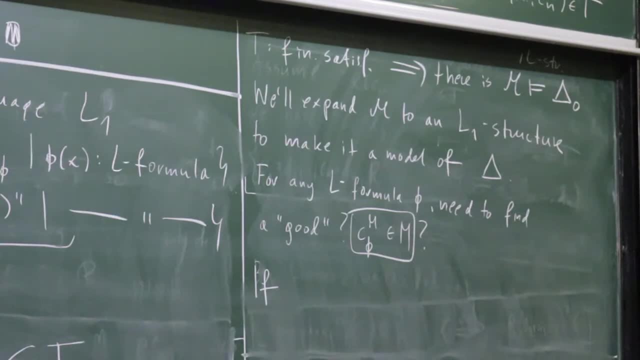 it. so we just look, there are two, there are two options, so if it may happen, so now we really give a meaning to it, we give a meaning to this witness property. if there is something to witness, then we pick a witness. if there is nothing to witness, we pick anything. 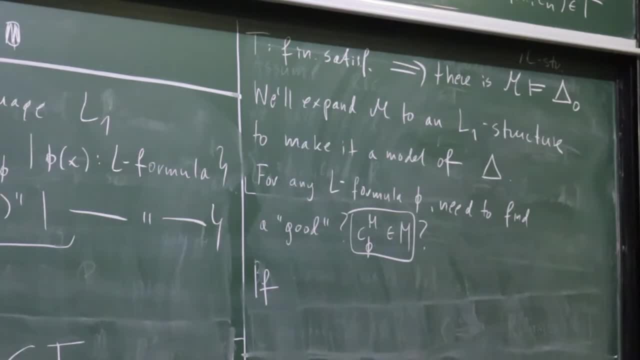 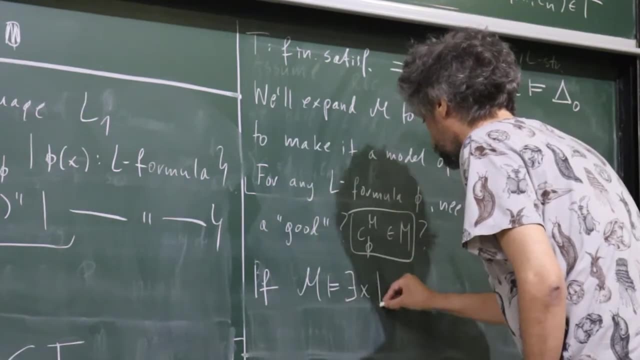 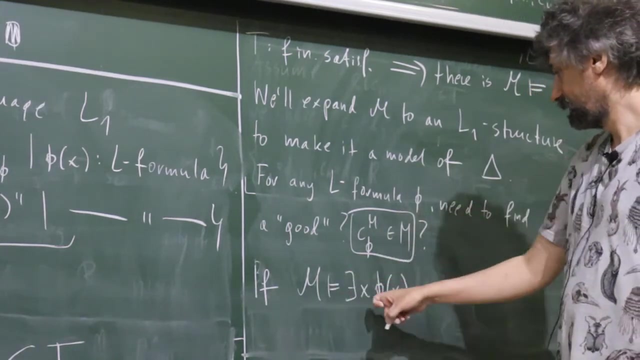 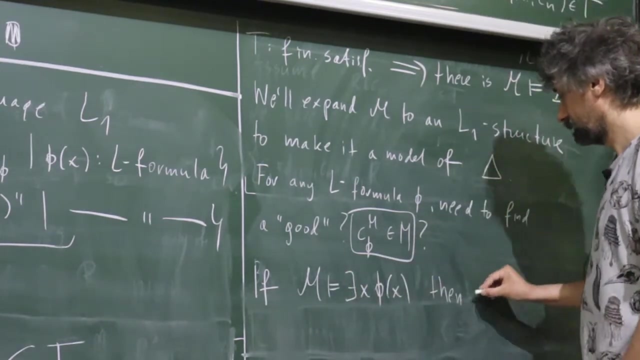 just nothing very deep, but a little. we cannot do it totally randomly. so if it is true that in m this holds, it means there is some element in m such that there is some element in m such that the c of this element is true in them. then 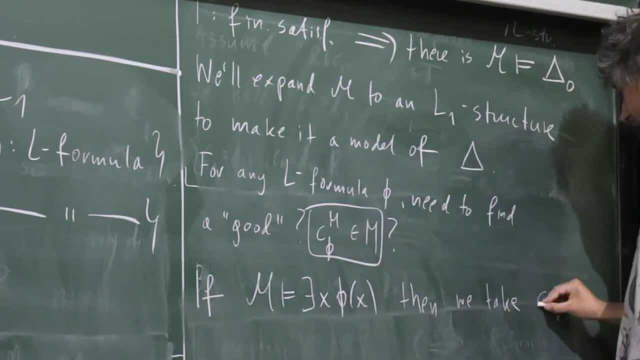 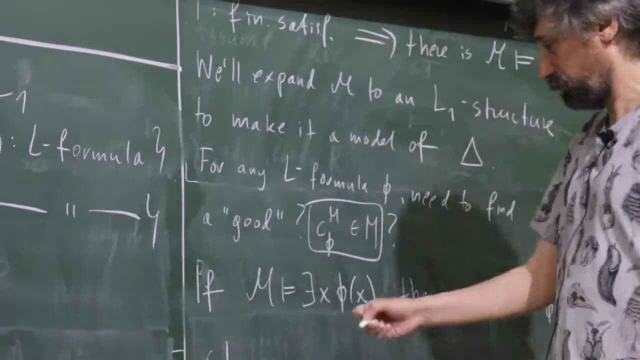 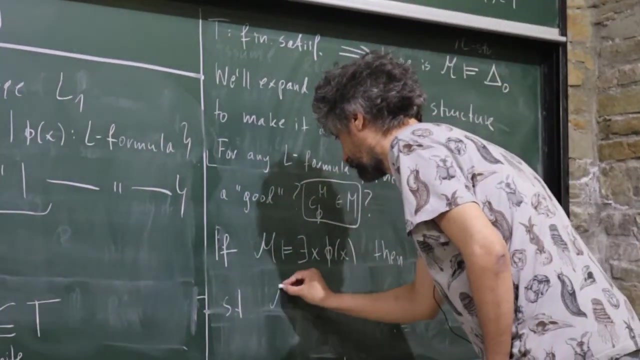 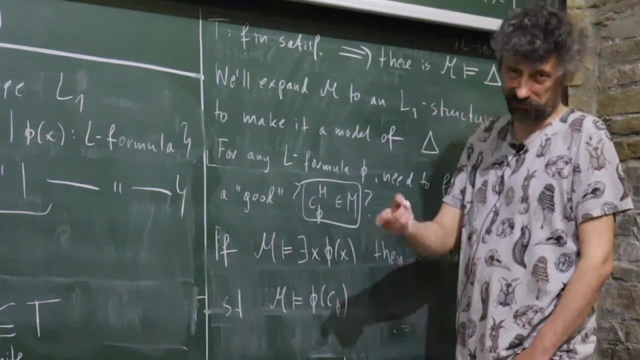 we take cpm such that it is a witness, it really witnesses the truth of this sentence. so finally, this witness becomes really a witness. so finally, this witness becomes really a witness, becomes really a witness. okay, if this is true, such a thing exists. okay, if this is true, such a thing exists. 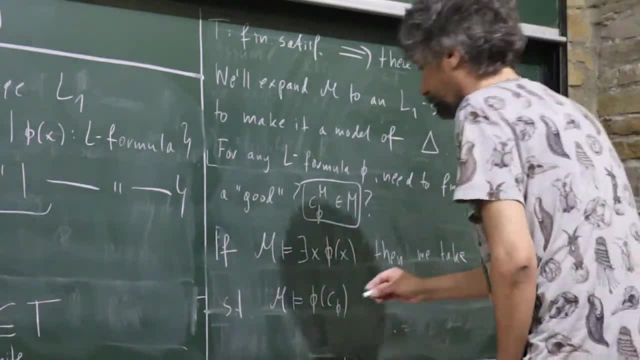 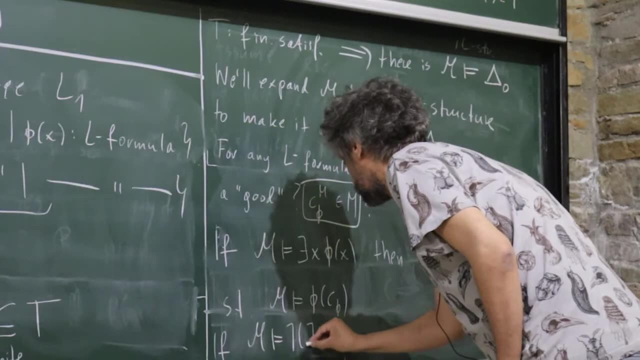 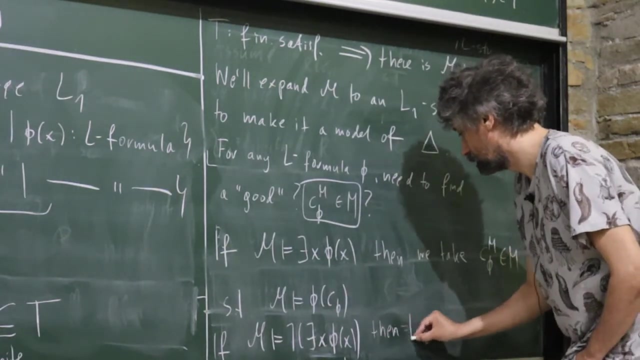 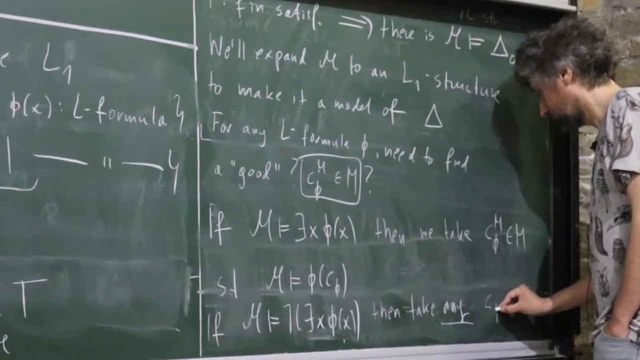 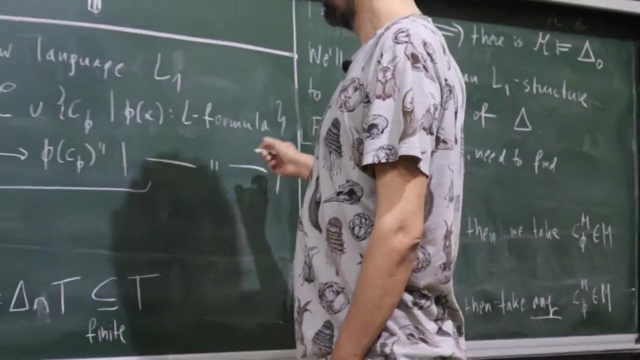 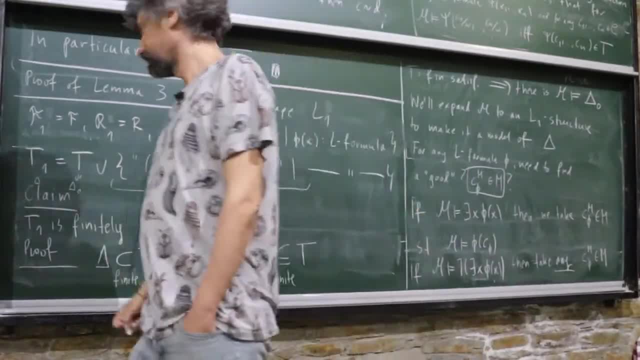 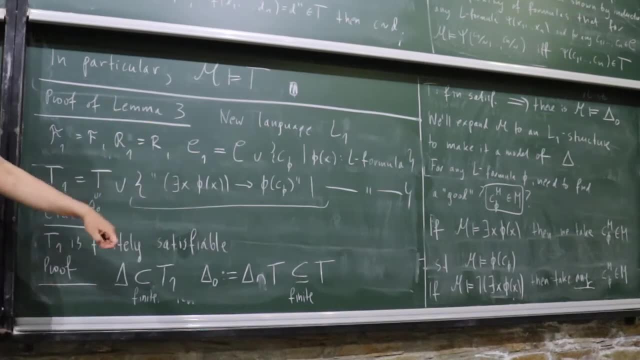 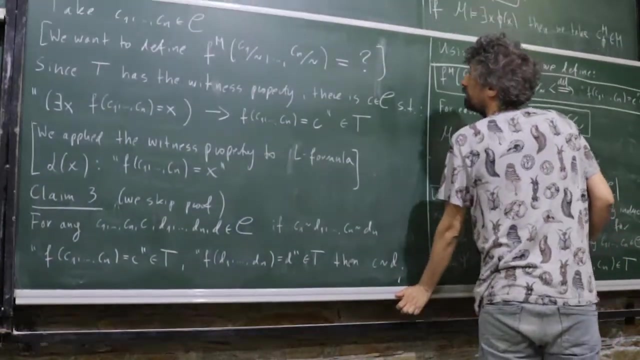 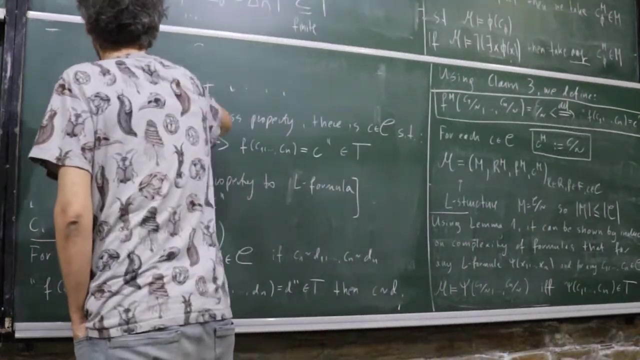 all of the sentences are true, because if this was not true, then this doesn't matter, because already the whole sentence is true. if it was true, then we choose the right one. because if this was not true, then this doesn't matter, because we are doing track and test. 광idk department. 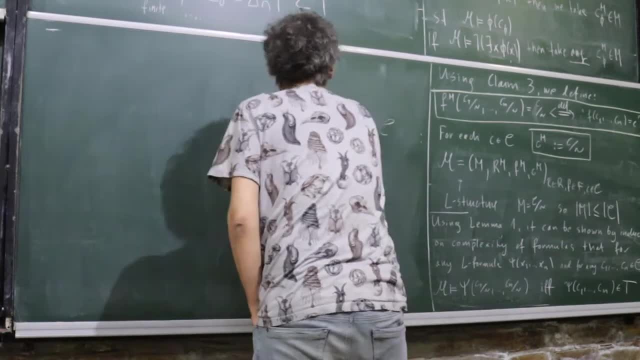 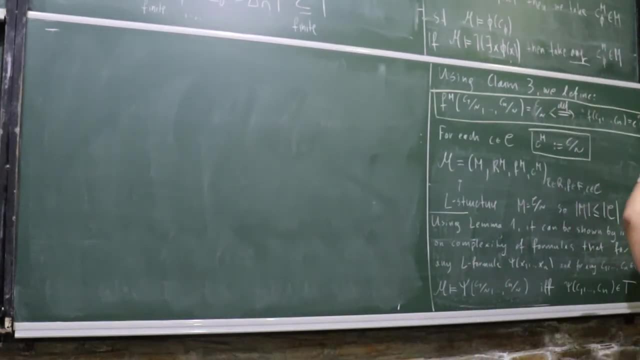 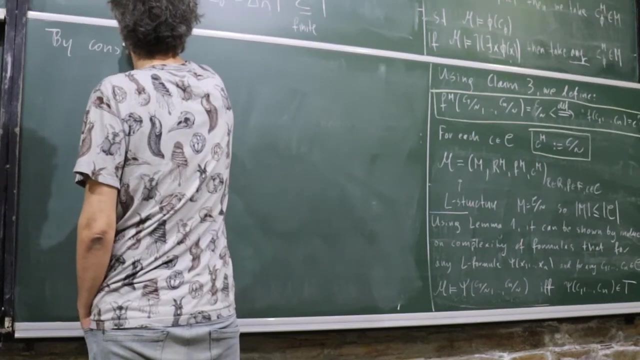 of course grandeur barresining- mirror image- stronger norm. and of course grand reading- mirror image- stronger norm and mirror image stronger norm. and when you are lucky and present, the choice of small will do the work, all with string on prepared, okay, so why construction? so this a the like old thing is brand new. 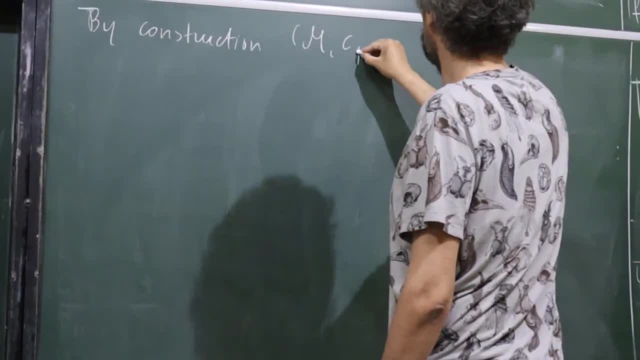 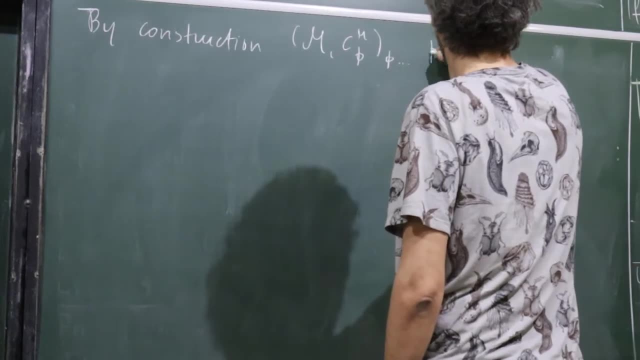 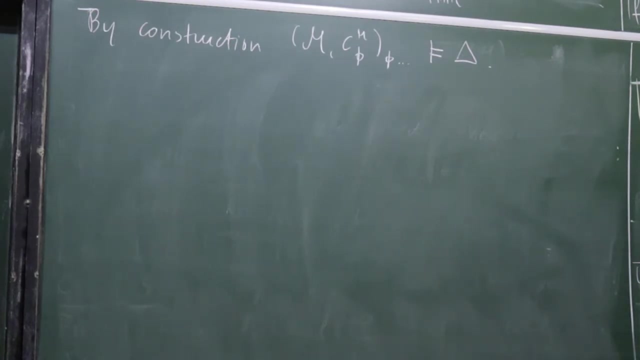 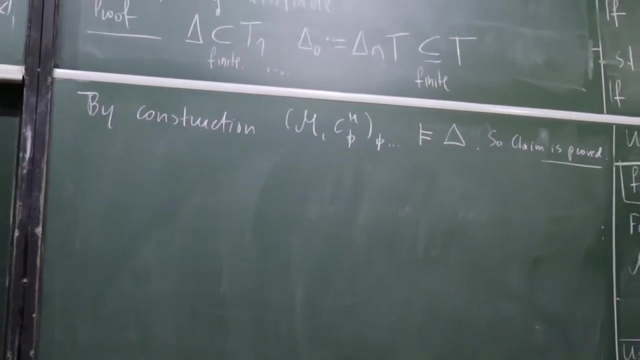 so this a, the like old thing is brand new. this m with all this c phi m, there's all these other possible sentences, so claim is proved for any finite subset of this new theory. we found the model by founding model of this old part and interpreting this constant. it should be interpreted by the actual, by the. 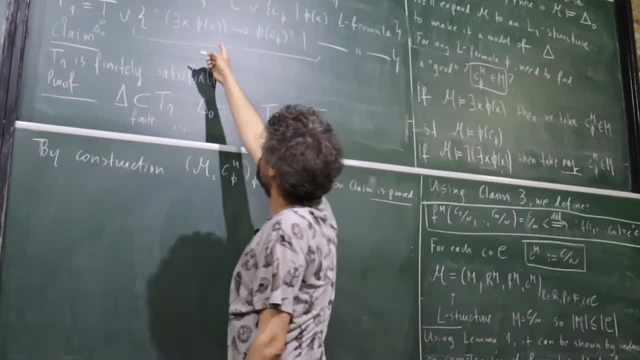 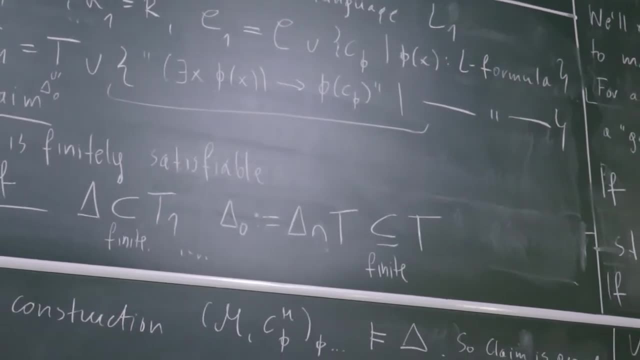 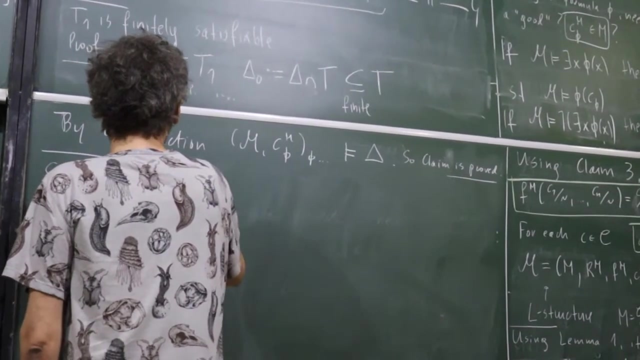 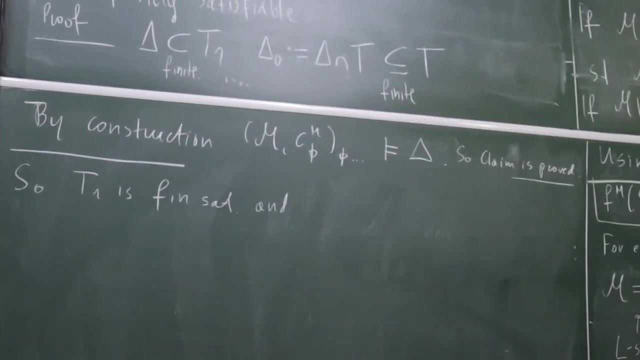 actual witnesses of this part here. okay, so we have a claim, and now we continue. so we have a claim, and now we continue. so we have a claim and now we continue. so t1 is finitely satisfiable but, as i said, it does not have the full witness property. it has witness property with respect. 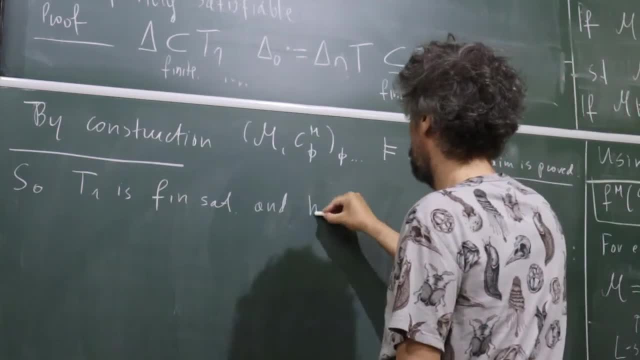 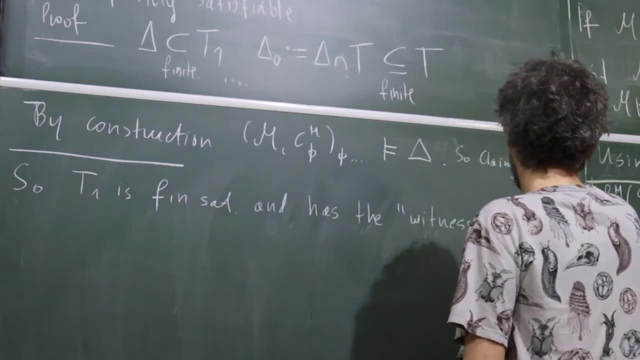 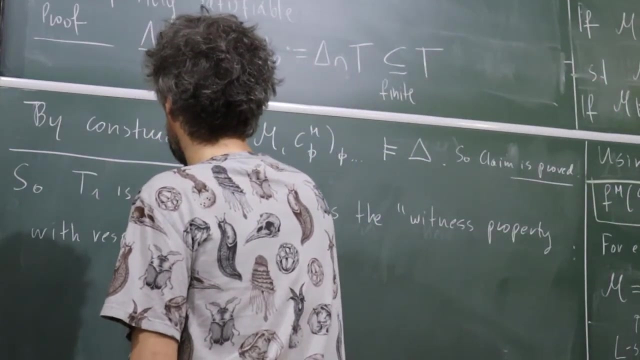 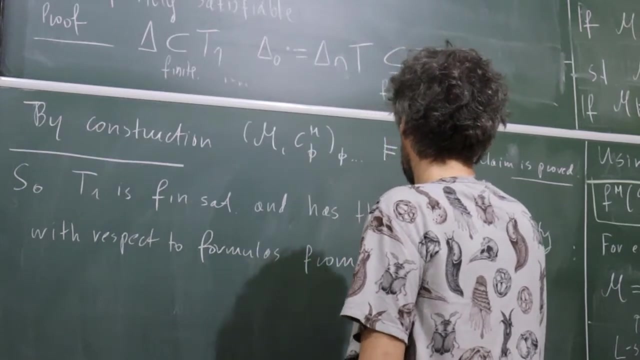 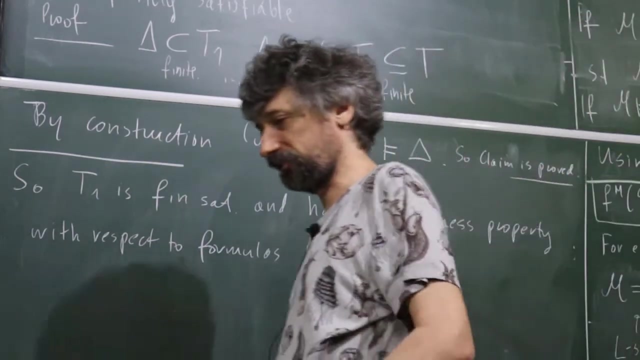 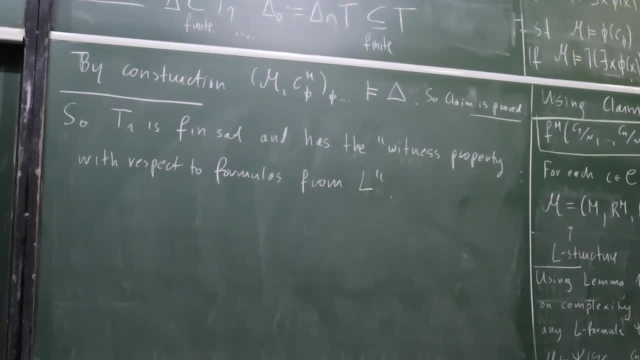 we got some bigger field which has all the solutions of polynomials. of the smaller field we repeat the construction and then do with aleph 0 term. we get the solids n parameters of the basis fields, but we don't know yet yet. the Theirar estaqty is a- yeah, it is an- arbitrary. 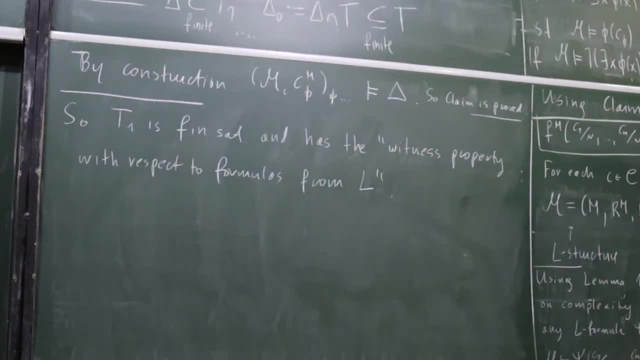 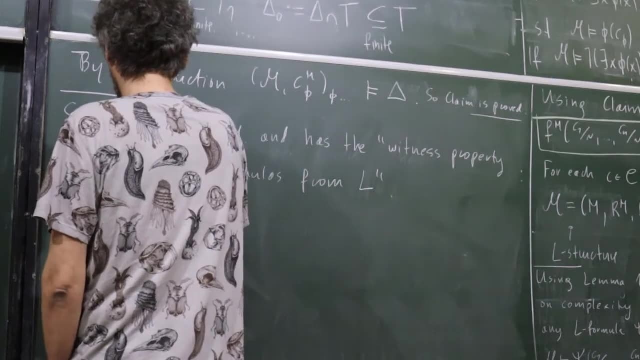 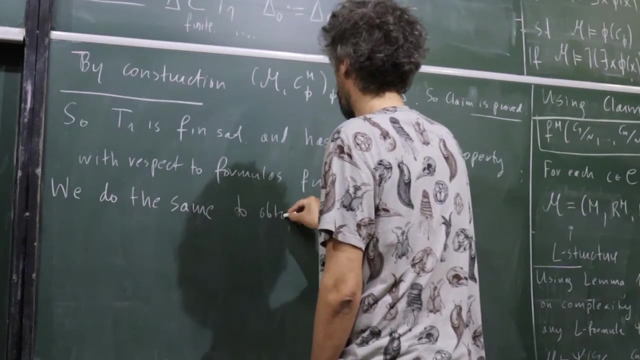 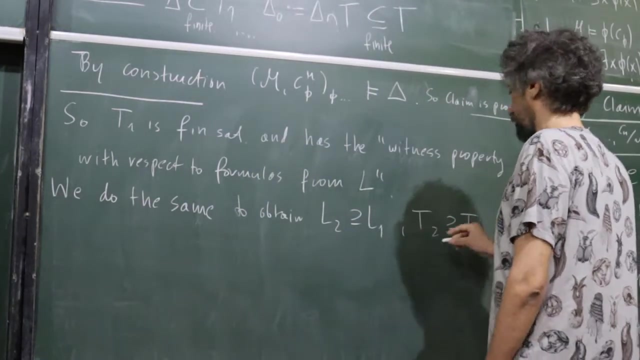 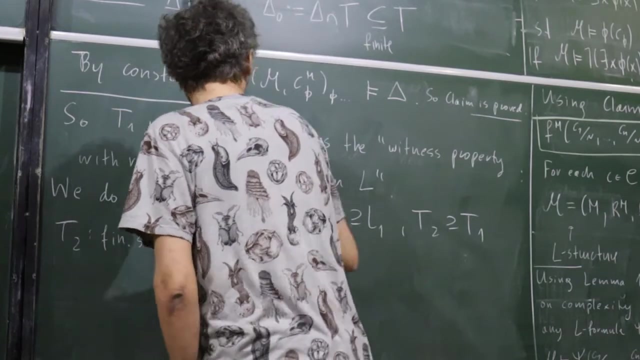 do it aleph 0 times and at the end we can algebraic the closed field and here it's the same. so now we do the same to obtain language l2 and t21, such that t2 and has the same. so, so, so, so so. 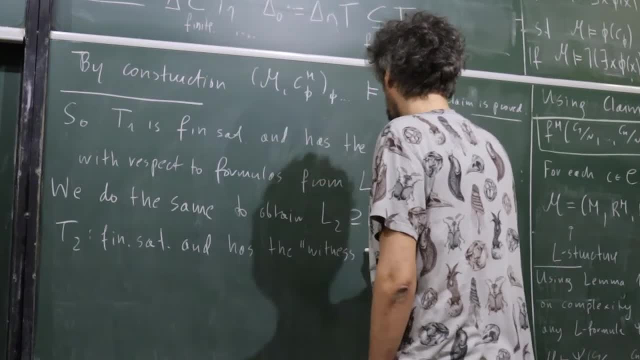 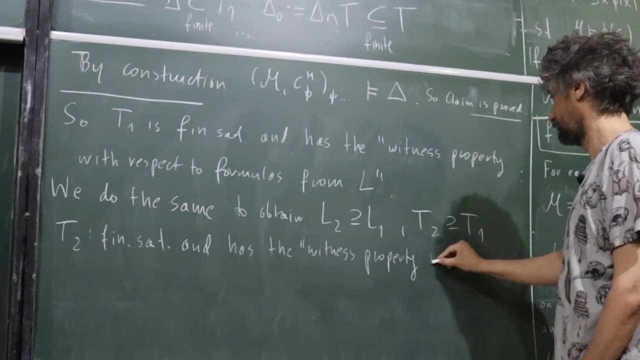 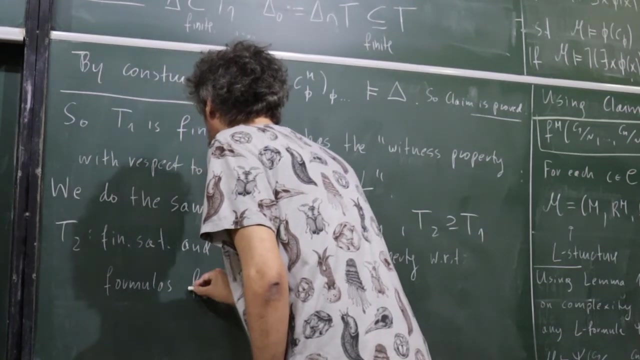 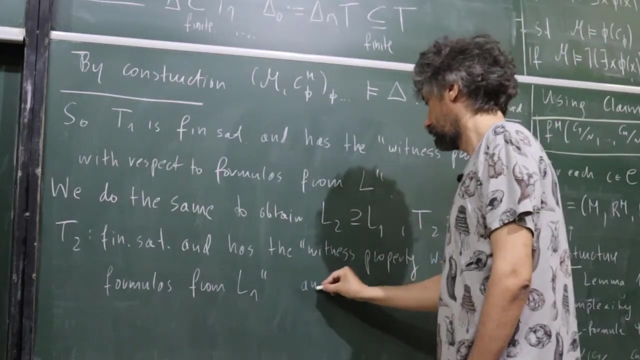 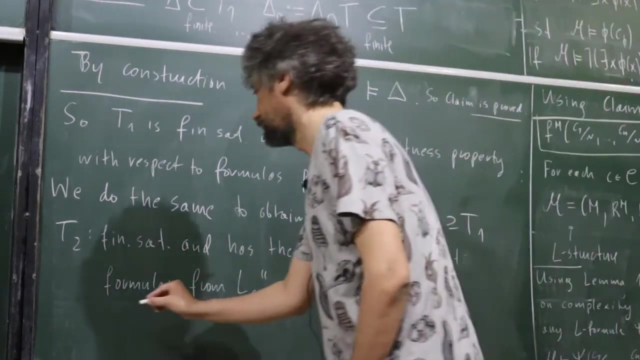 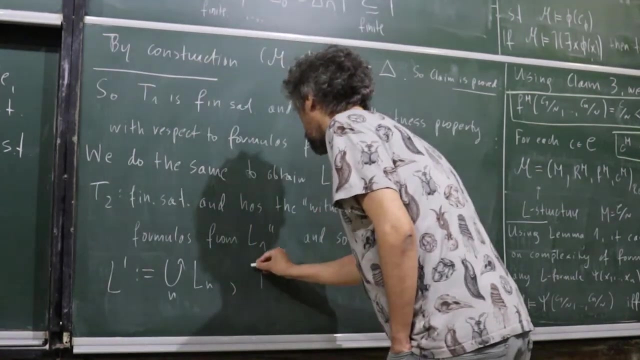 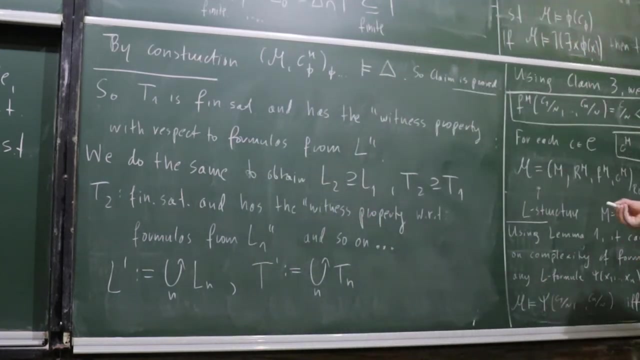 so witness property with respect to formulas from l1. so of course we continue. so at the end we can. our l prime is the increasing union and t prime is the increasing union of tn's and they all were finally satisfiable. it witnessed on the finite part. so this is finally. 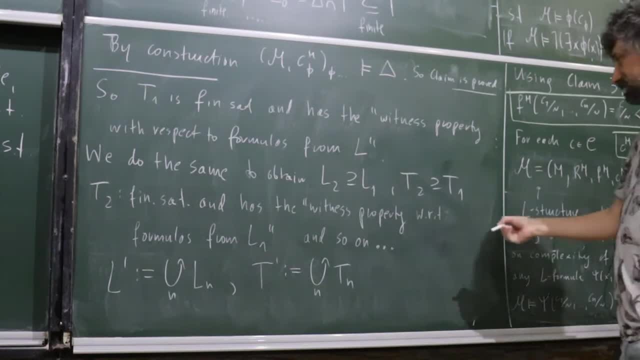 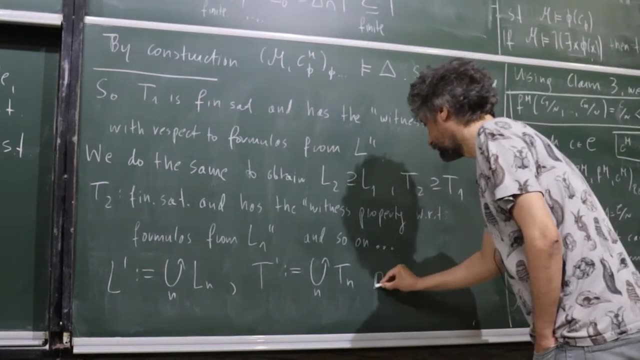 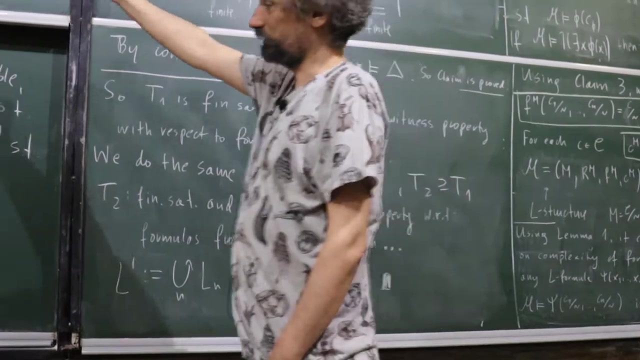 satisfiable and then, by the construction it has witnessed, property with respect to the good language. so this is, this is okay, okay, repeating this process and repeating. and so it was not enough to add all this constant once, we had to add them again, and again, and again. 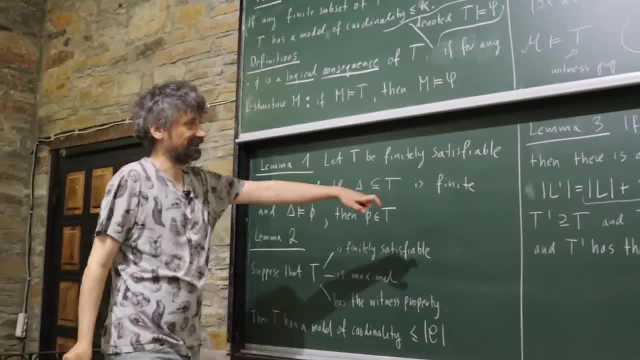 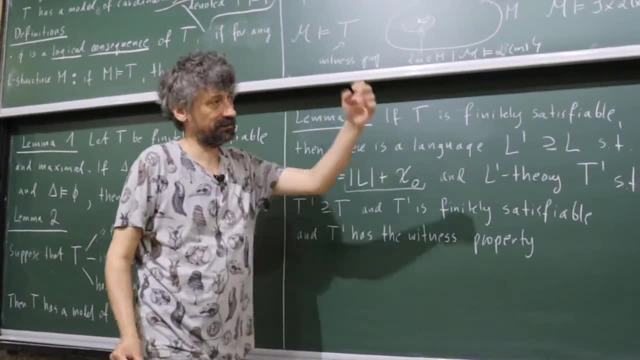 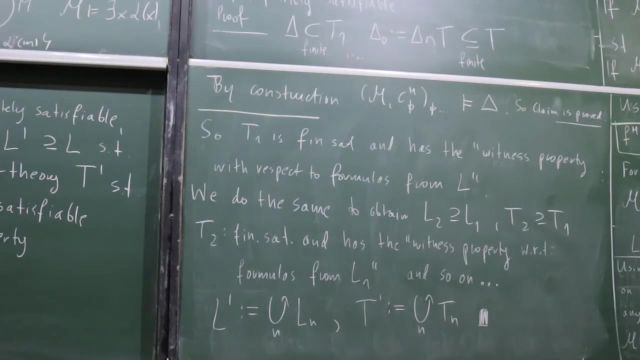 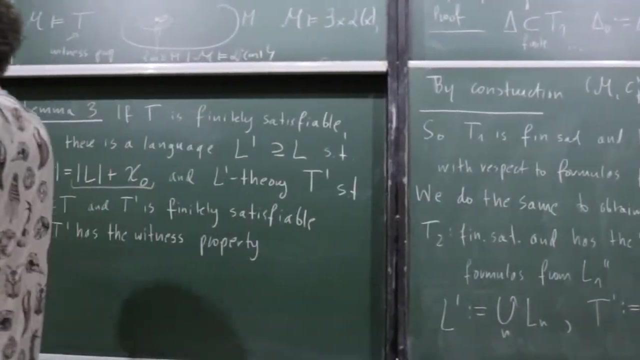 but it was happened cantably many times, so the cardinality did not grow over this. because this is number of formulas and we repeat the process cantably many times, will i finish today? so now the last lemma. this was about getting witness property. now we have to get maximality. 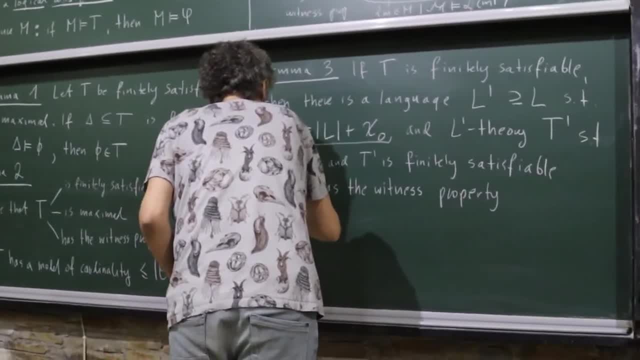 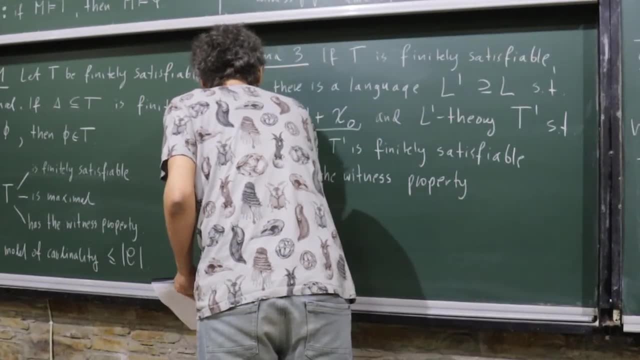 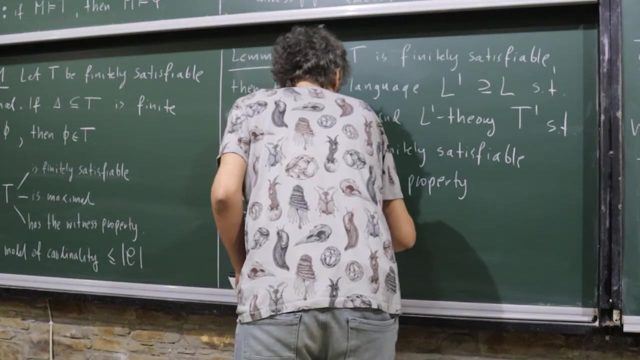 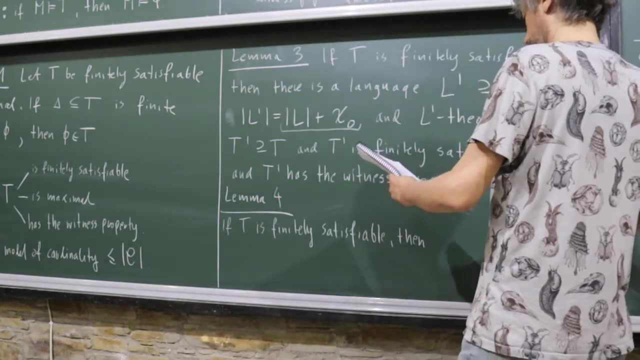 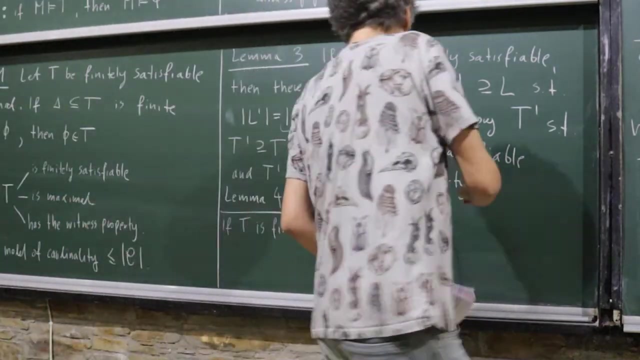 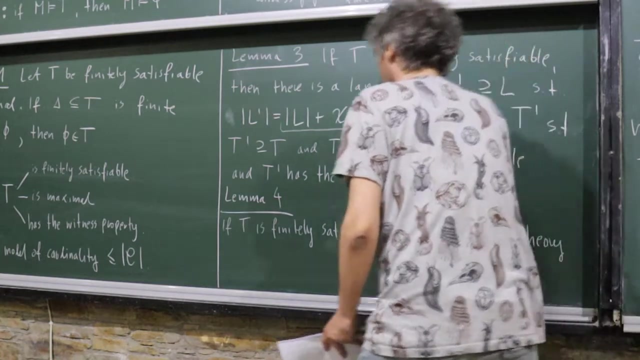 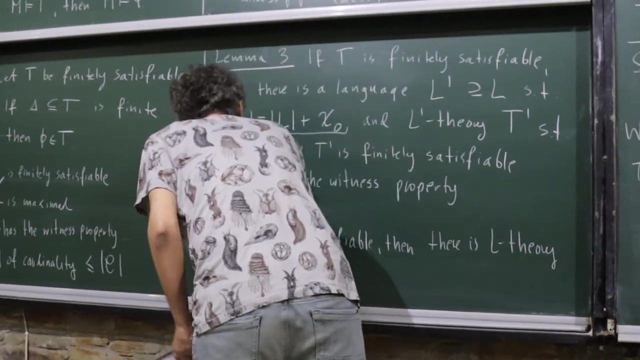 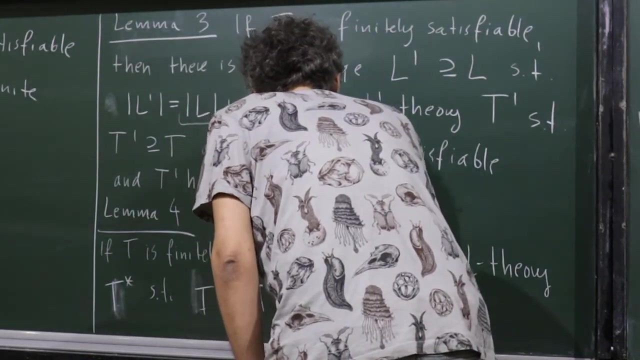 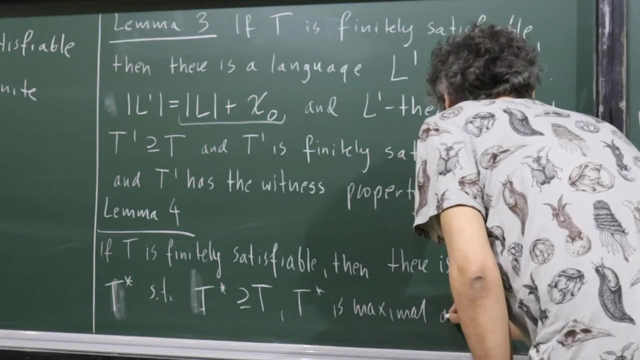 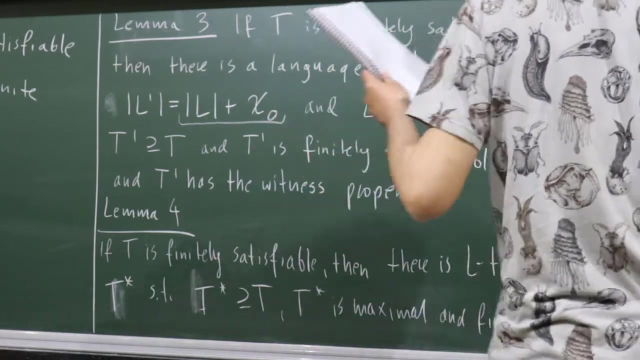 so this is lemma 4. now we don't have to change the language. so if t is finitely so, so, so, so then in this way: uh, silver, when very, very, very contains T, T star is maximal now and finitely satisfiable still. and after this I will be: 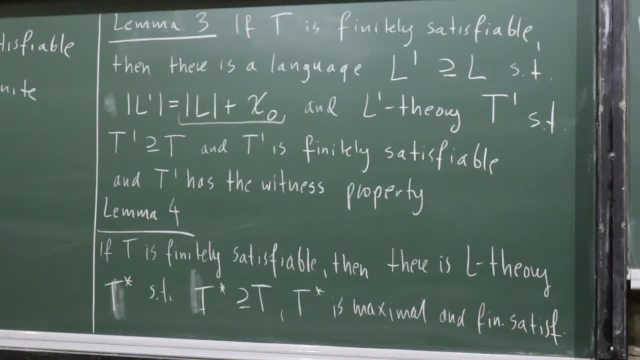 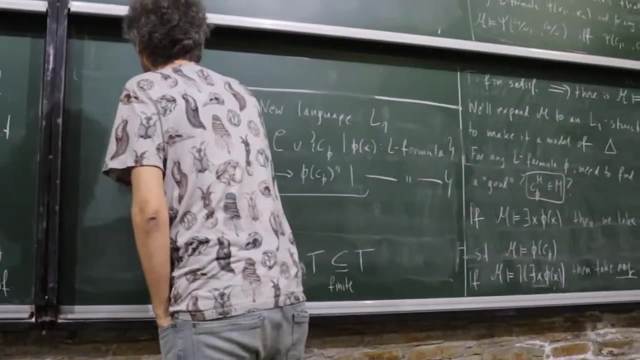 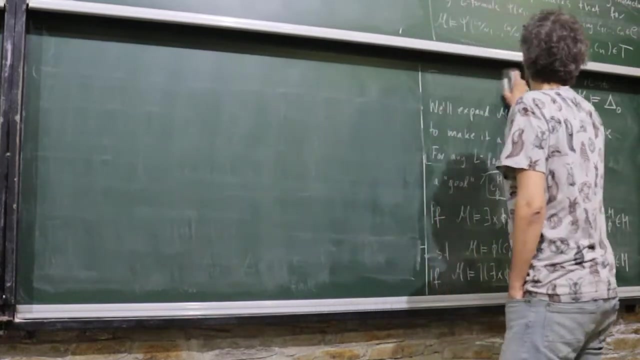 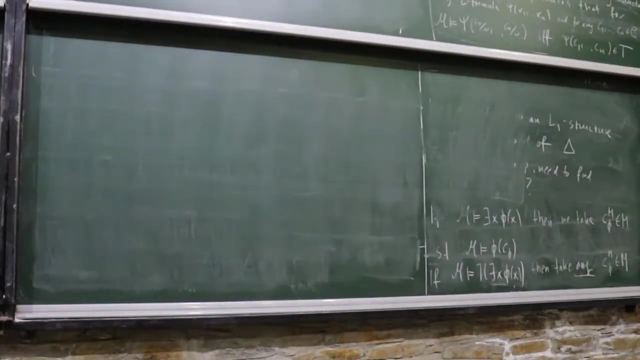 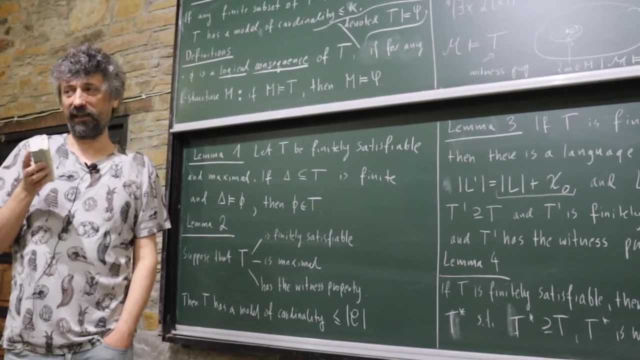 able to prove compactness theorem. but I will have no time. but this is the moment. okay, this is slightly interesting moment. so far, I think there was, there, was, was there an axiom of choice used? yes, okay, maybe a bit with these witnesses, but now it will be strong here it will be kind. 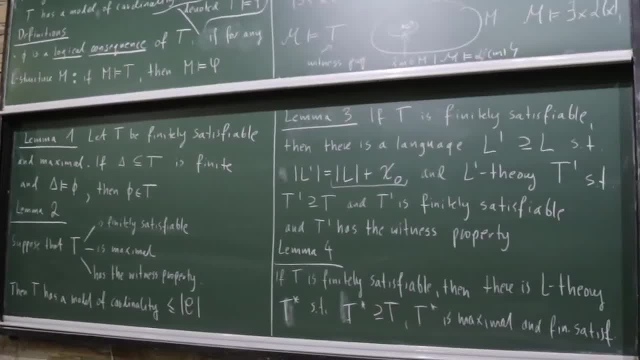 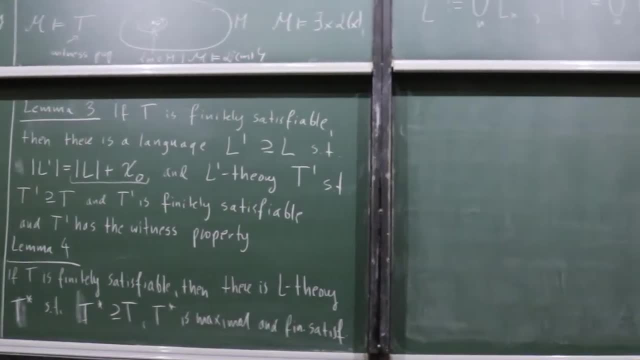 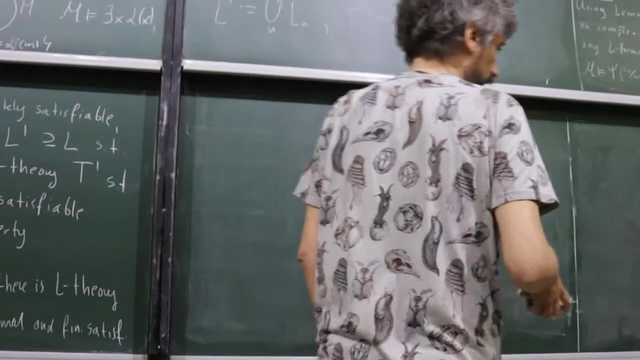 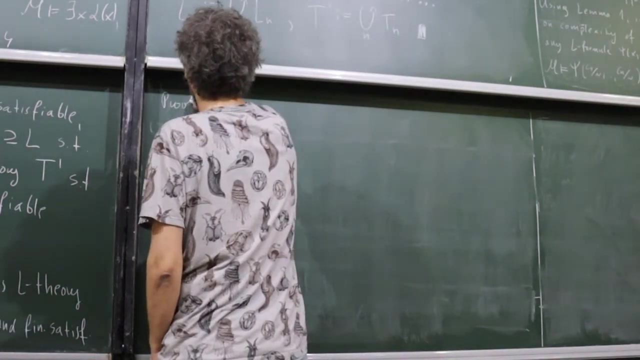 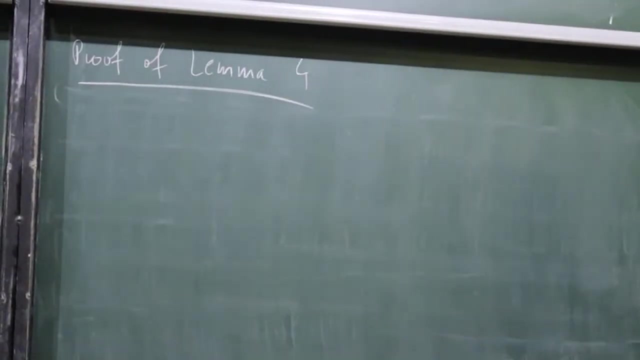 of strong usage of axiom of choice to find this maximal one. so this, this will is kind of non-constructive moment of the proof. this lemma 4: okay, as usual. yes, as, for example, if you want to find maximal ideal, it's axiom of choice. so 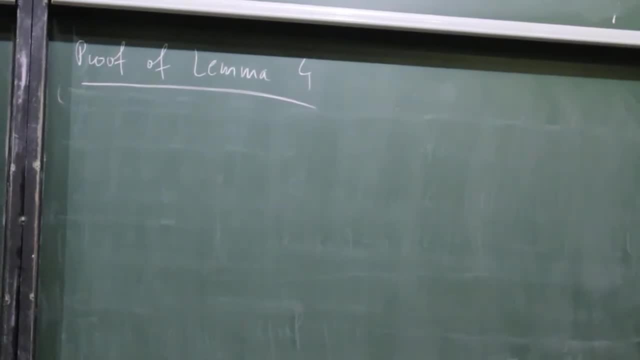 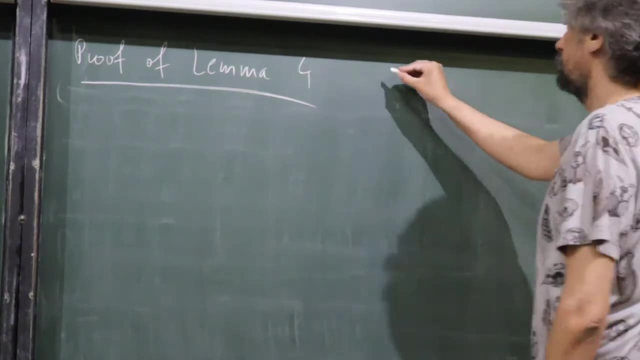 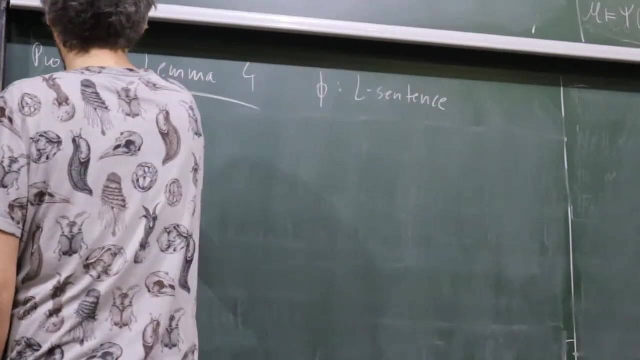 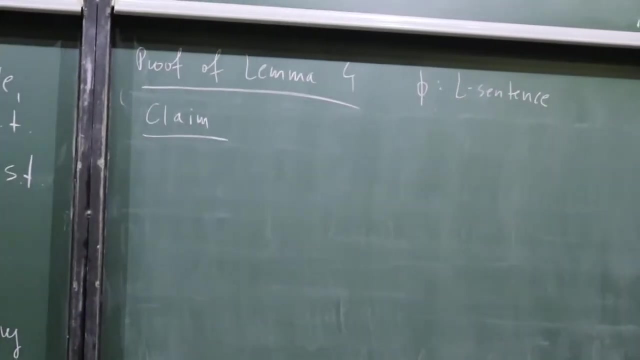 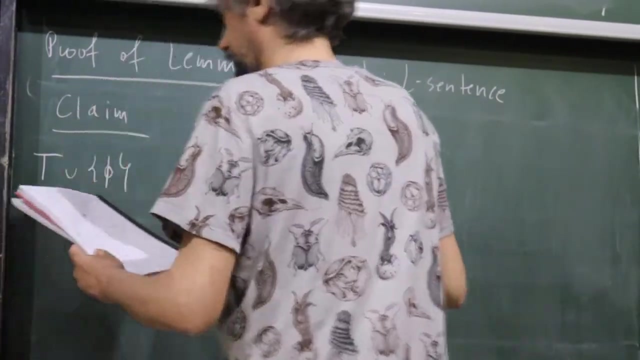 it's similar thing here. okay, so it will be kind of: let us have an L sentence, so now claim: have an L sentence. so now claim our T is finitely satisfiable. so I'm saying that like something which is needed to apply Zorn lemma either. this is finitely satisfiable. 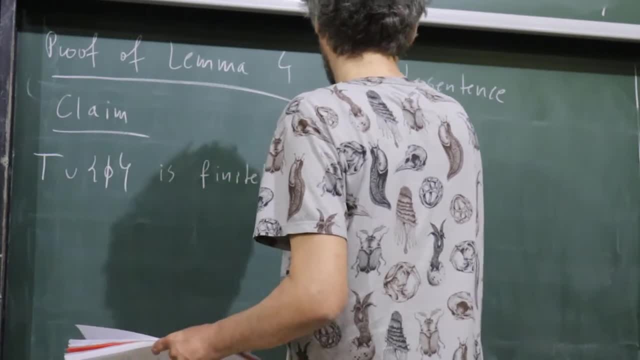 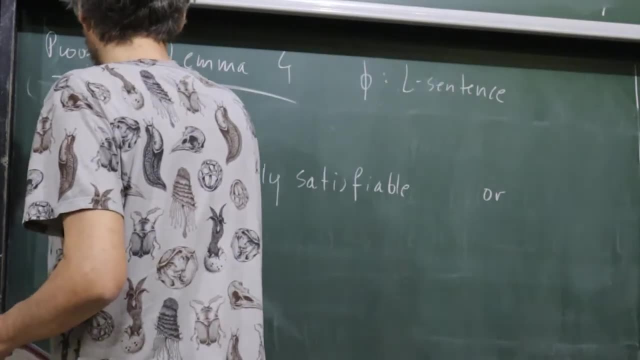 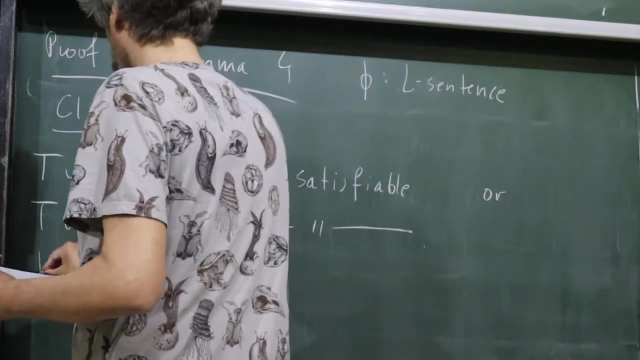 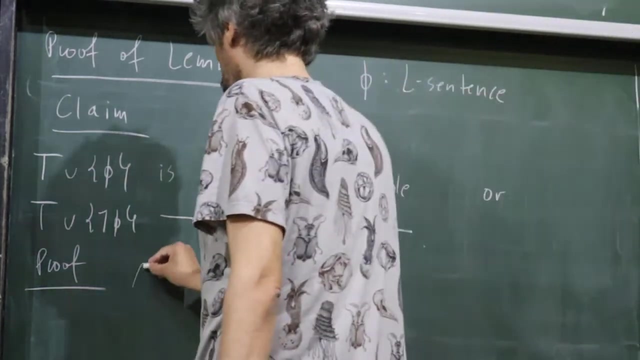 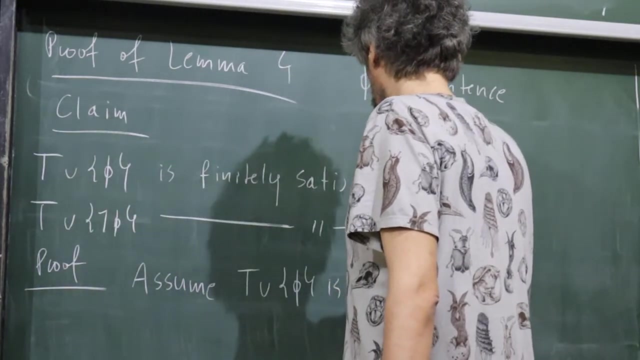 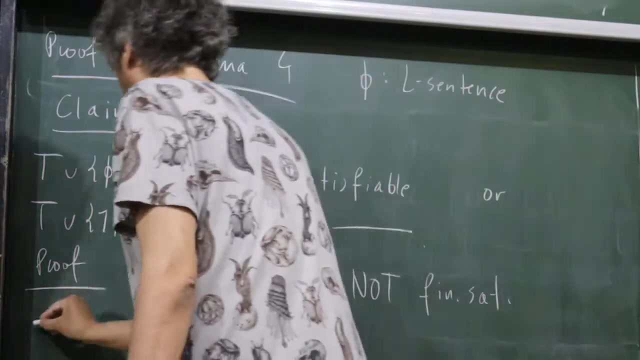 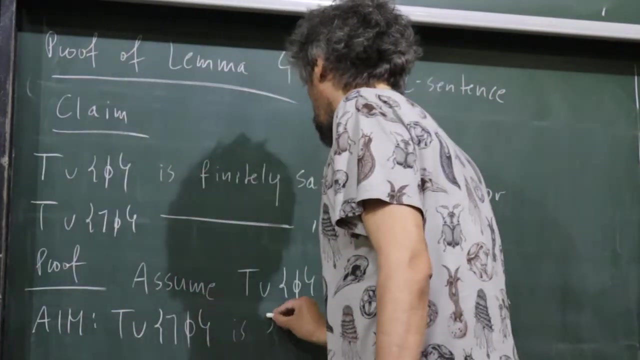 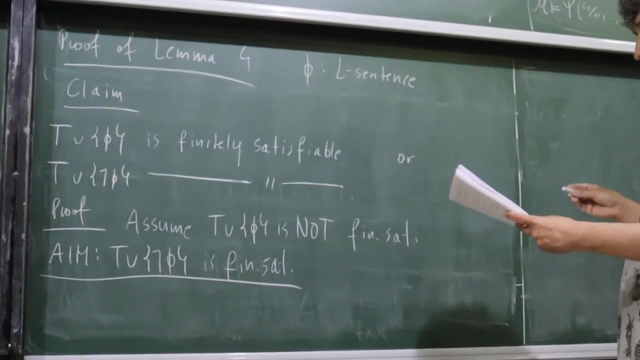 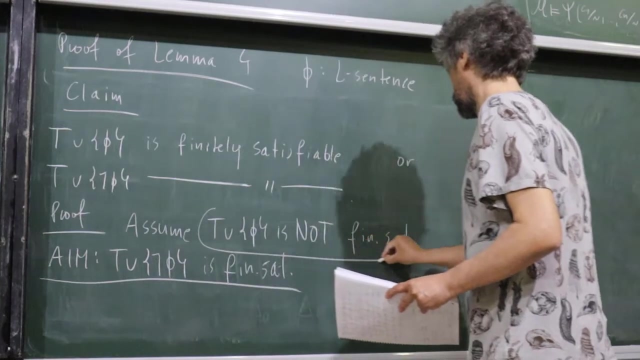 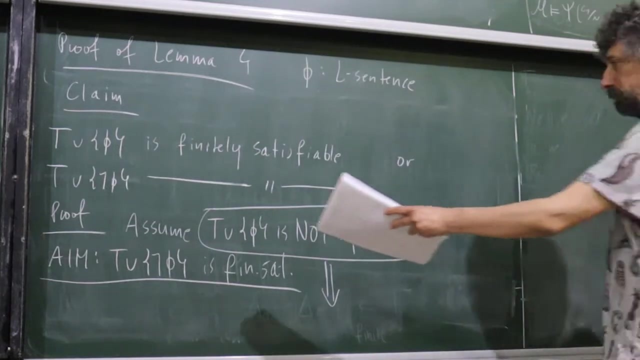 or this is: this is: this is proof of claim. so assume the first one is not finitely satisfiable. of course we want to show that the other one is is not finitely satisfiable. okay, so since this is not finitely satisfiable and there is some finite, 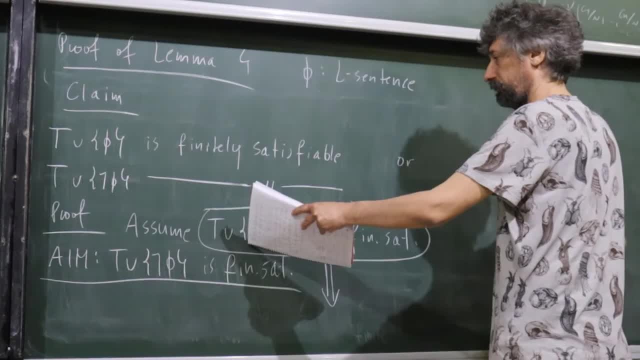 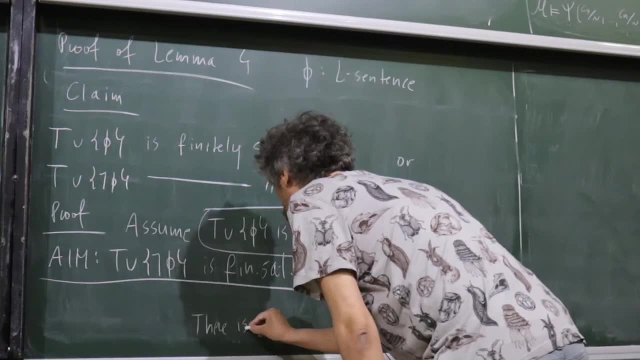 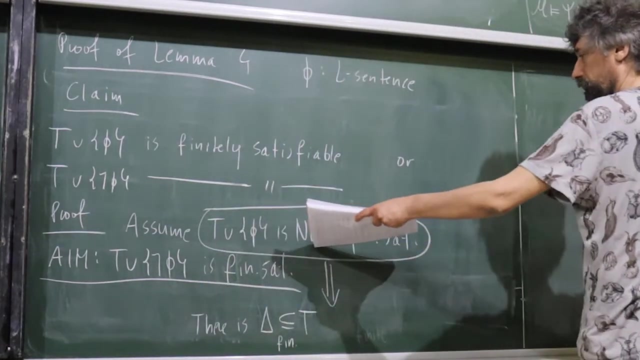 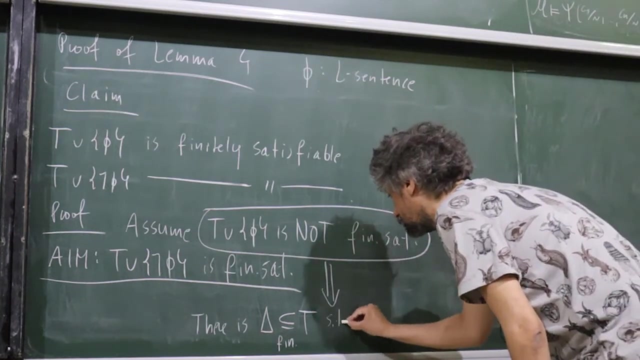 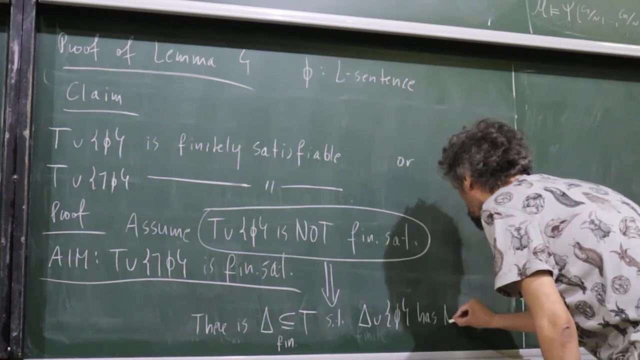 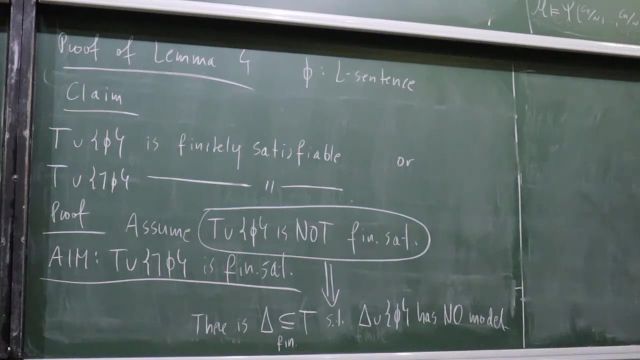 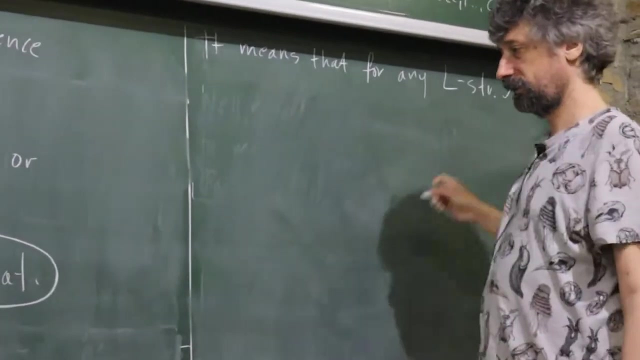 part of T, such that this finite part of T with phi has no model. yes, because the whole thing is not finitely satisfiable by assumption, such that novel structure is a model. okay, so what does it mean? it means that for any structure M if it satisfies this part. 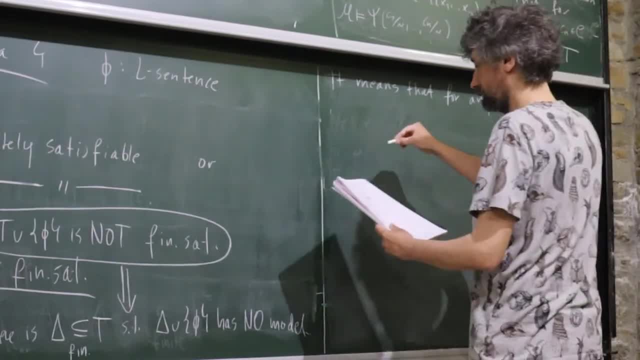 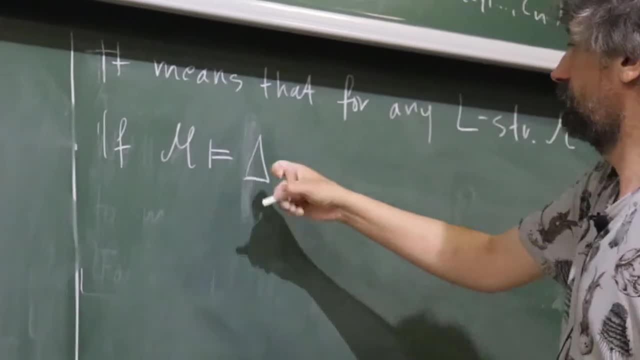 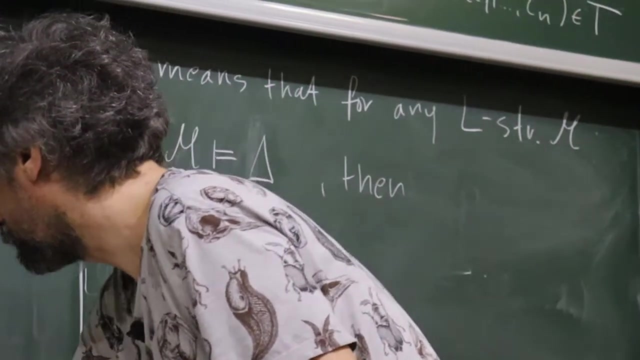 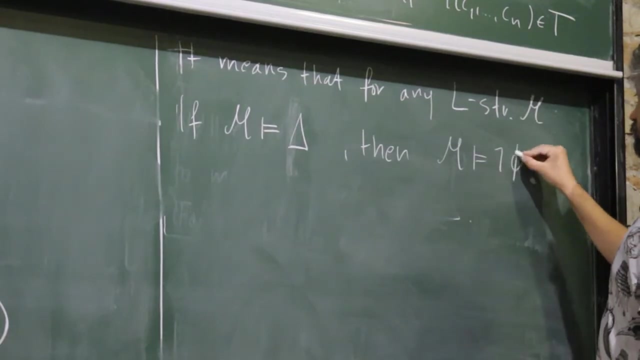 then it cannot satisfy this part. so if, if, if M satisfies, if this is a model of Delta, then it is not true that M satisfies phi. so M satisfies not phi. yes, because always one of them is true, but then. okay, now I forgot what's going on. 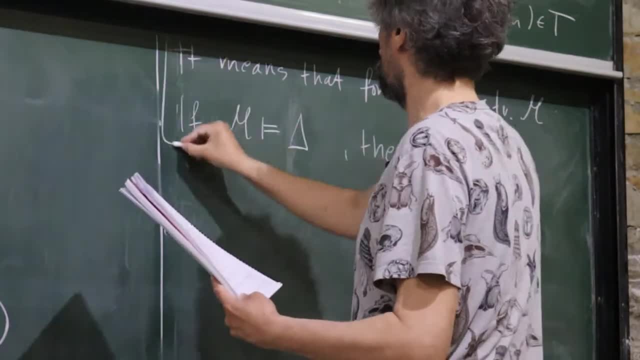 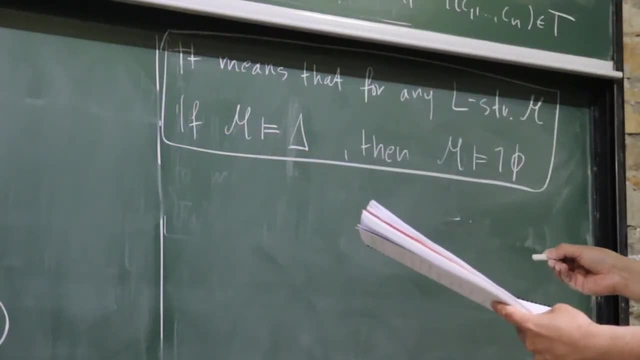 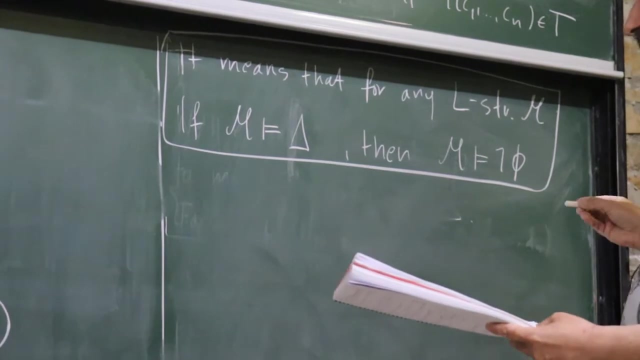 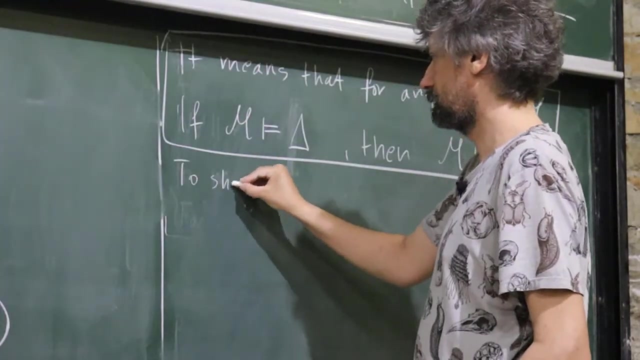 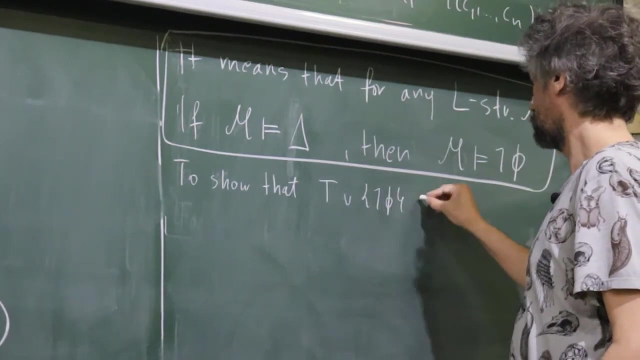 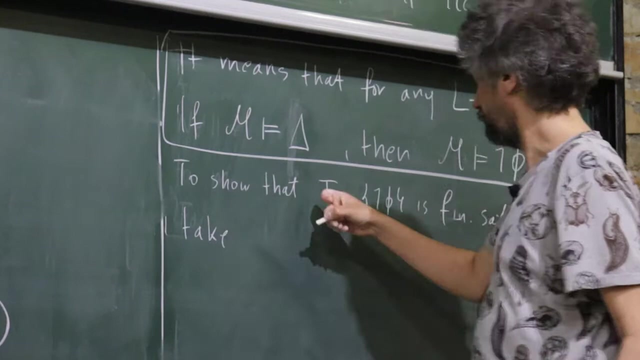 okay, so this is something which is true. okay, so this is something which is true. and so now we want to show that this is finitely satisfiable, and, and, and, and, and, and. we take a finite subset here, so a finite subset here and this negation of V, let's say: 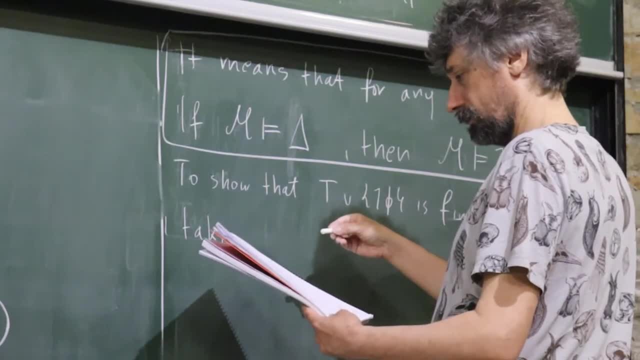 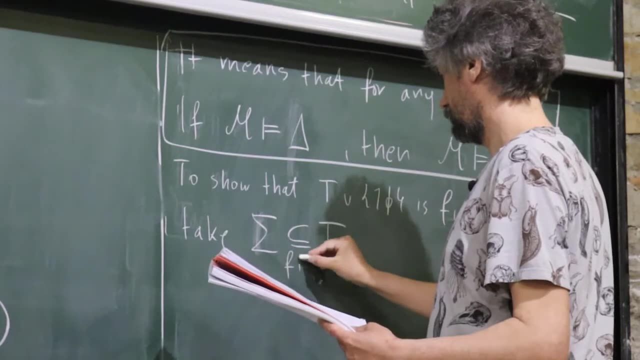 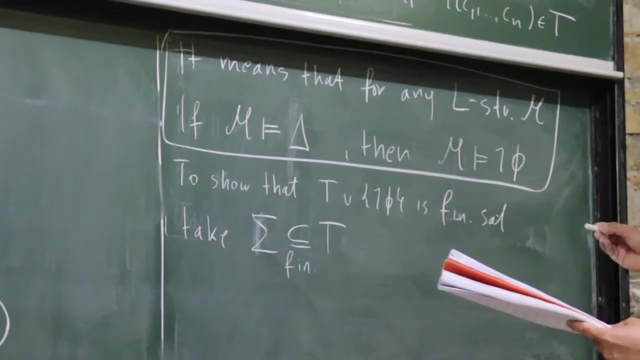 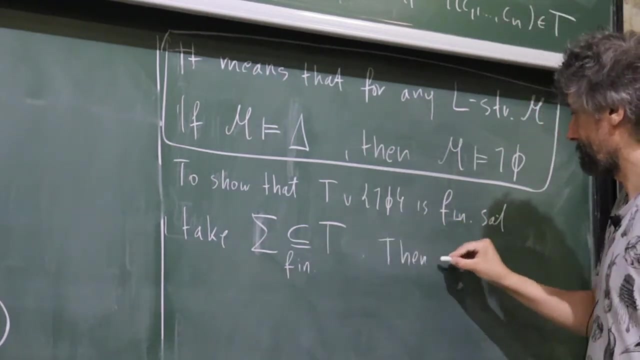 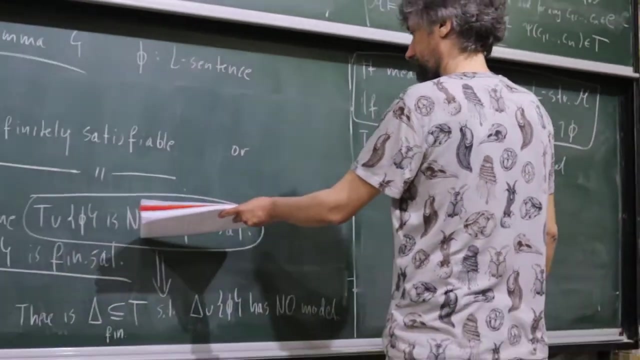 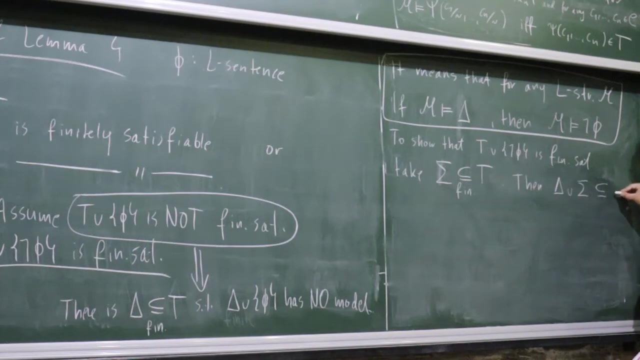 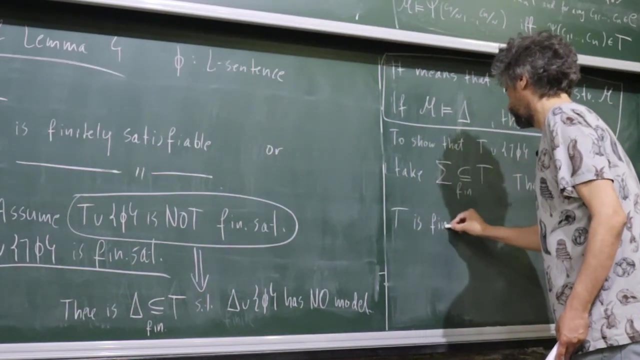 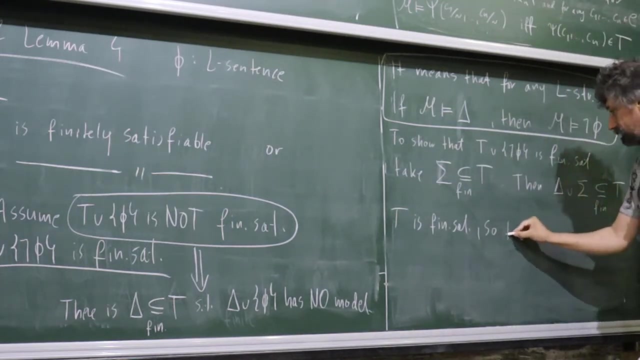 okay, but then now everything will be combined. this is finite and this is finite, okay. so then this previous one showing that this is not finitely satisfiable, together with this sigma, is finite. here t is finitely satisfiable, so there is a model of this part. 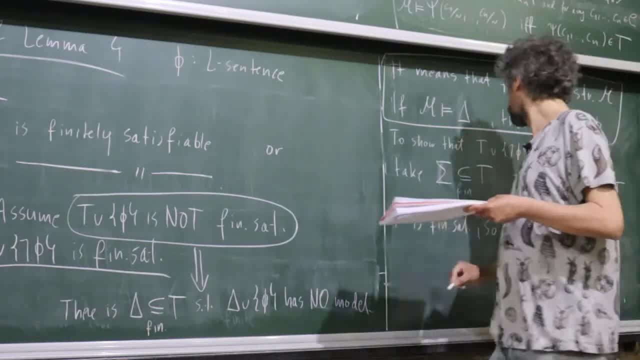 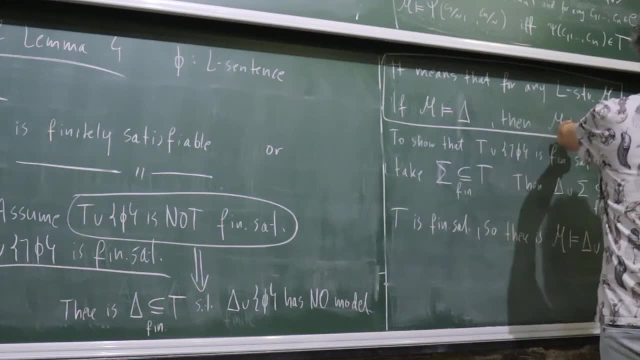 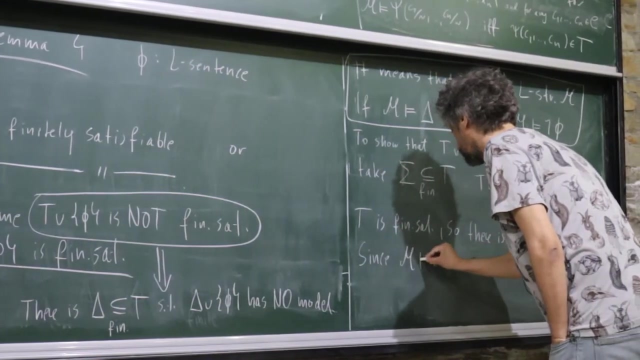 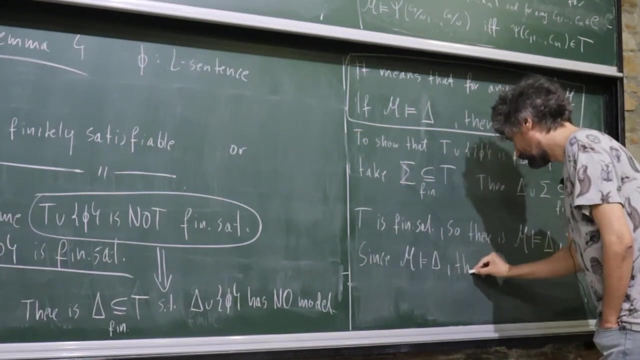 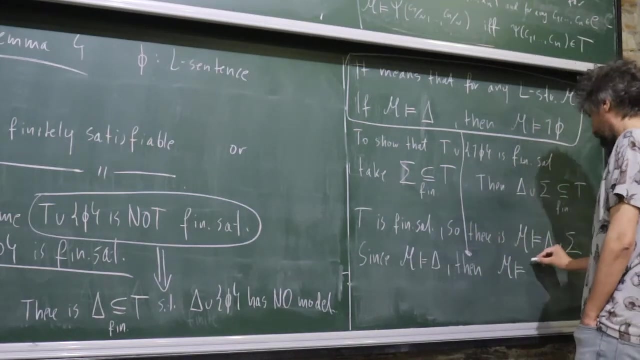 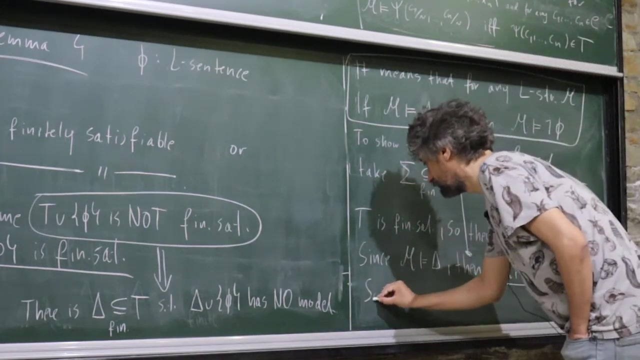 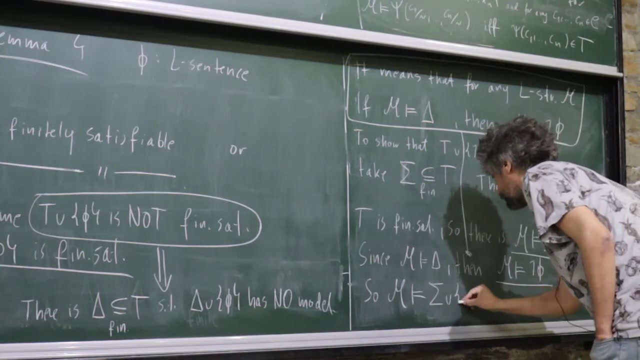 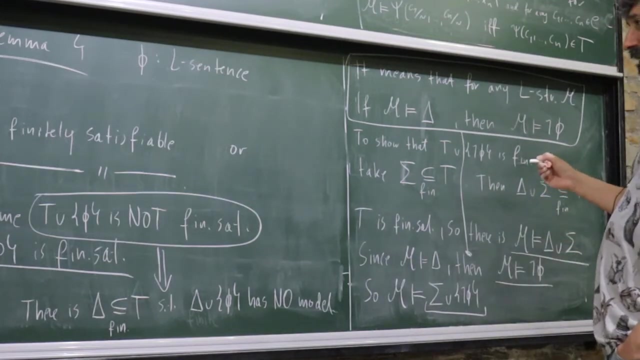 okay, but since m, in particular, is model of delta, m satisfies not phi, okay, okay. and then it satisfies this and this, so that by this part, so we have this, we have this, so m satisfies this, and this is arbitrarily finite subset of this theory, so it is finitely. 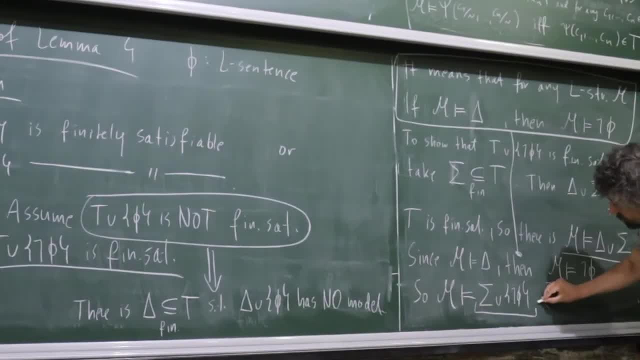 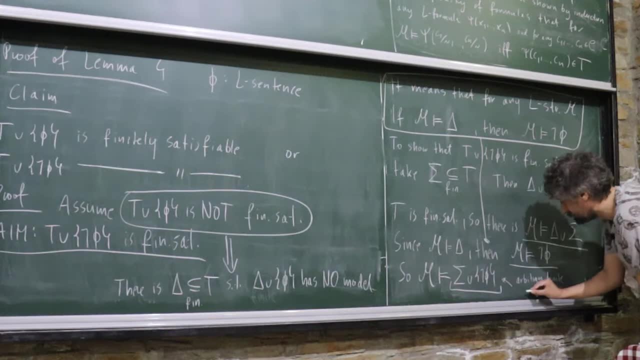 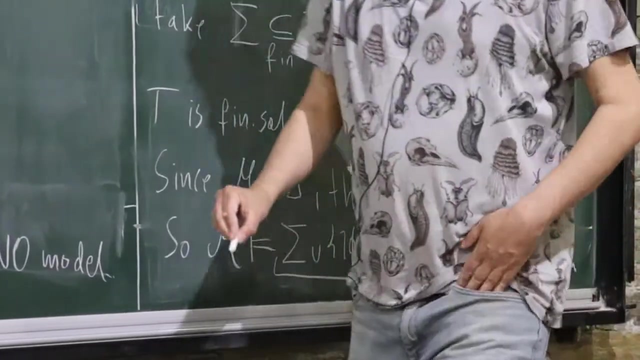 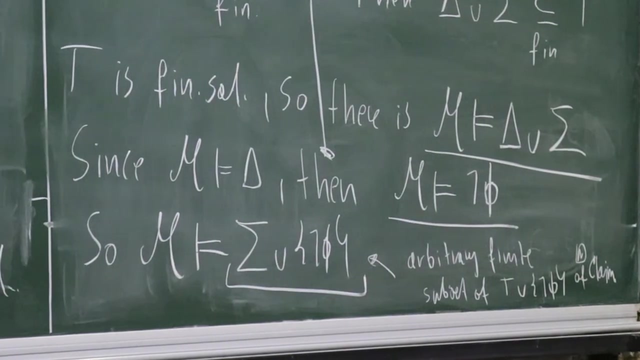 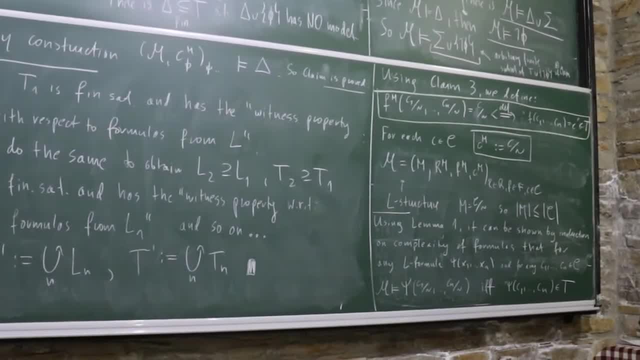 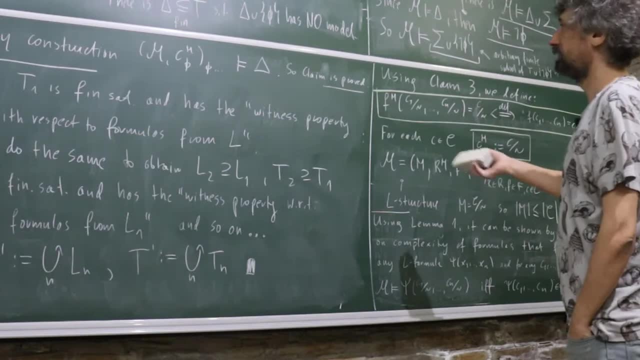 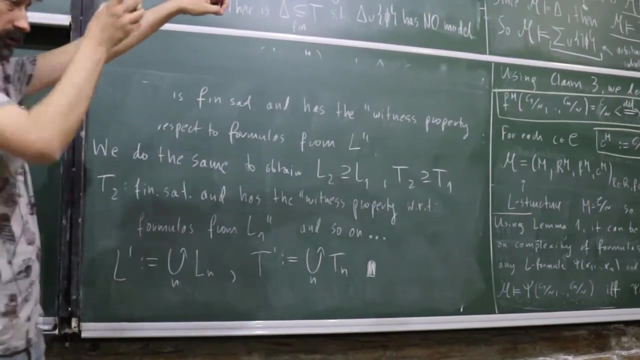 and now I am leaving you as an exercise to finish the project and I hope that you liked it. Thank you very much. and now I am leaving you as an exercise to finish the project and I hope that you liked it. Thank you very much. 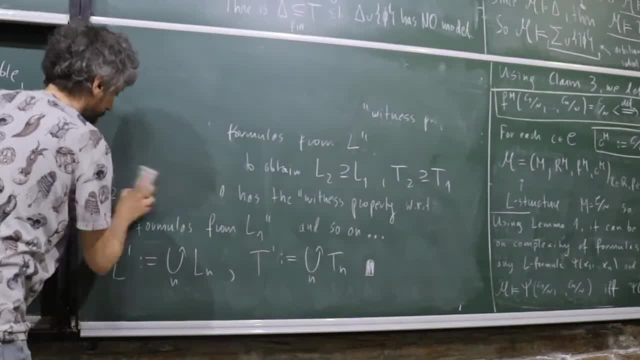 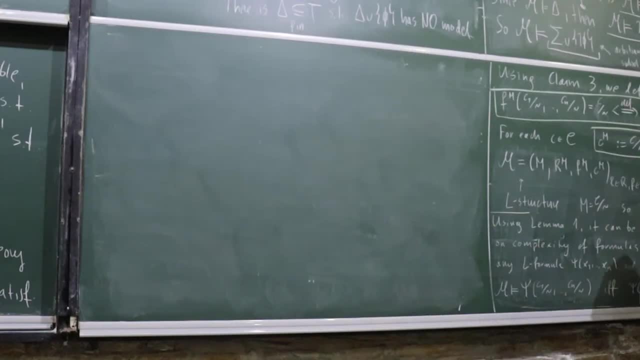 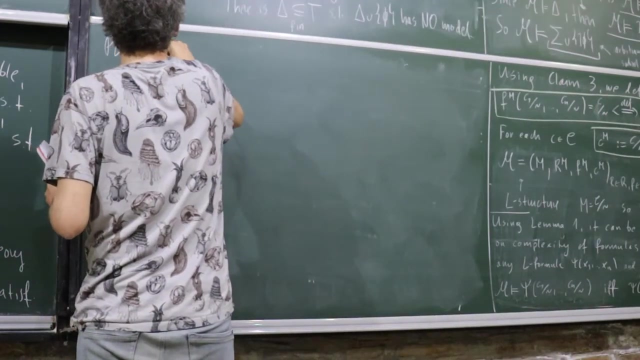 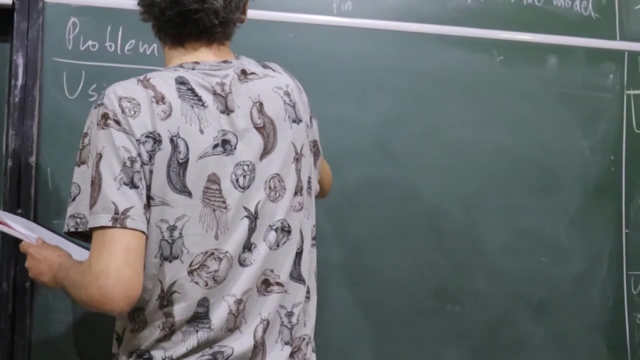 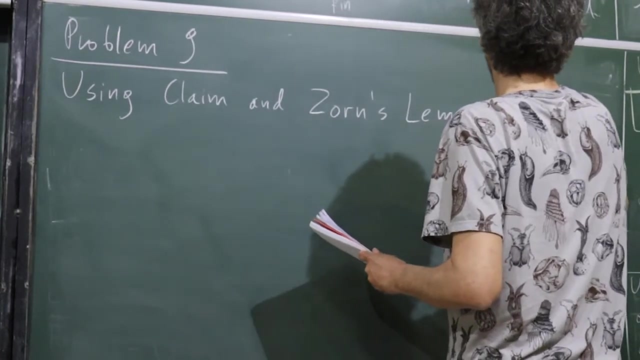 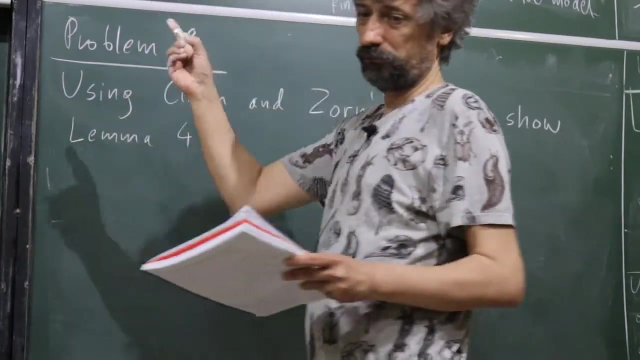 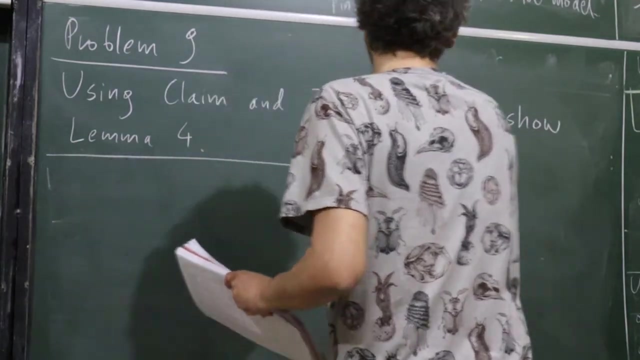 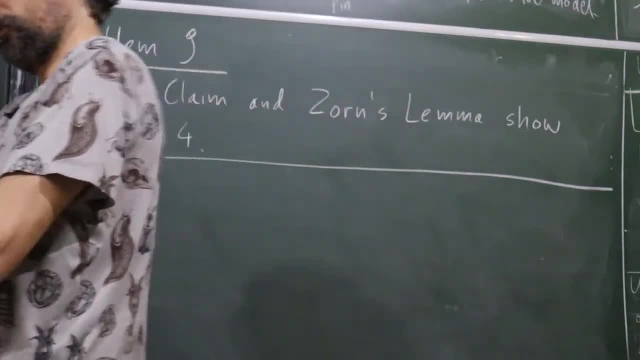 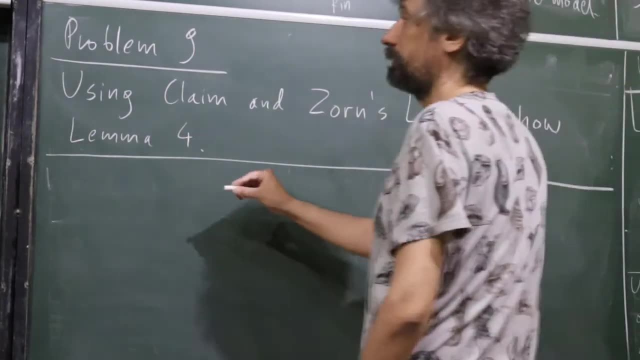 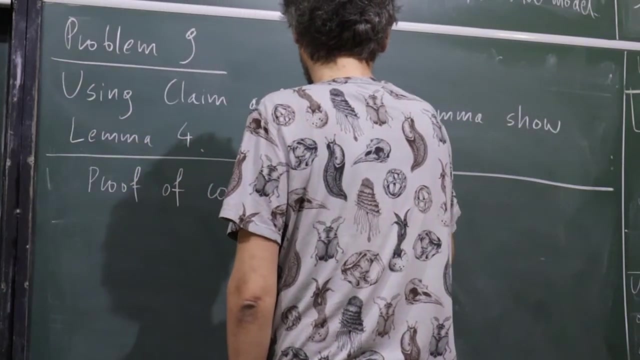 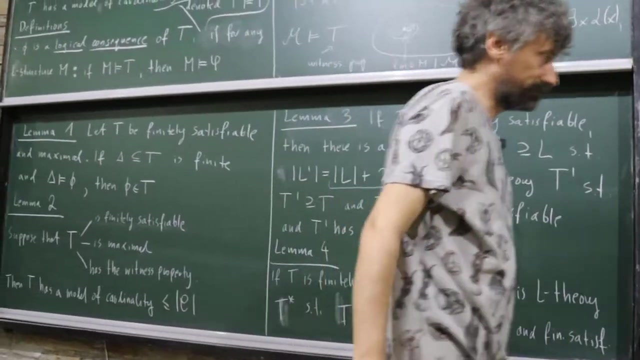 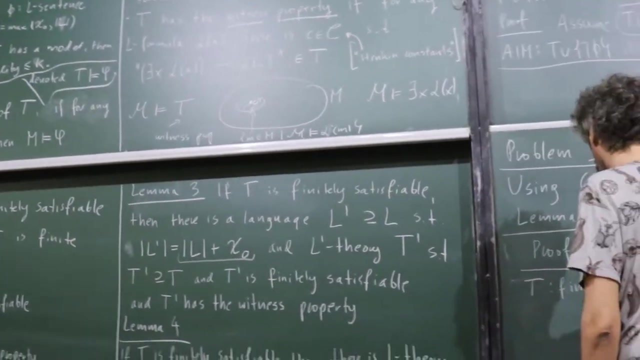 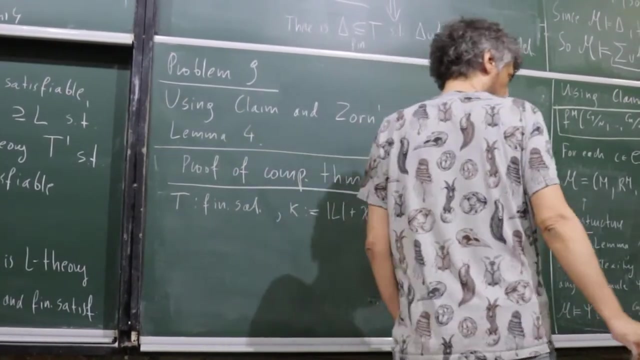 which is highly non-constructive. this maximality, okay, I guess I can finish compactness theorem, surprisingly so. proof of compactness theorem. so we start from the assumptions. T is finitely satisfiable, it's kappa and we want to find model. yes, we want to find model. 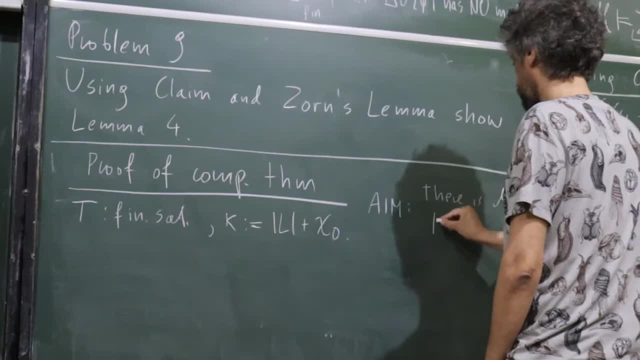 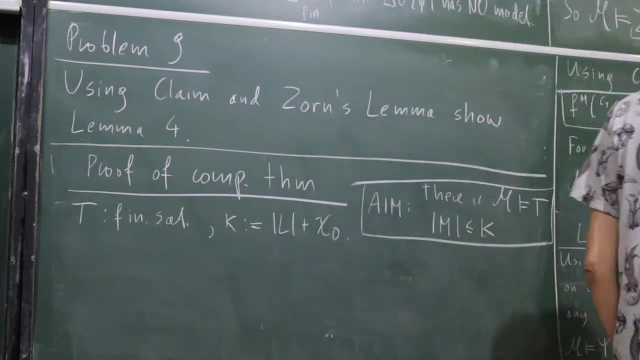 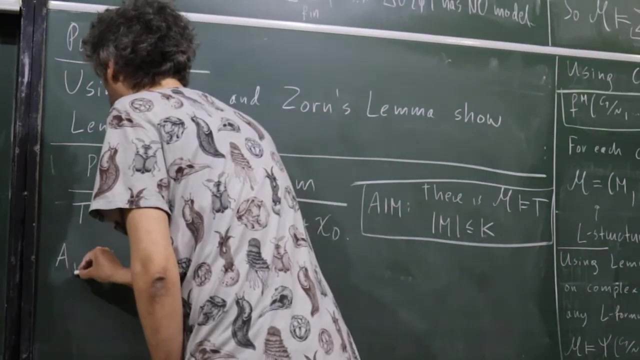 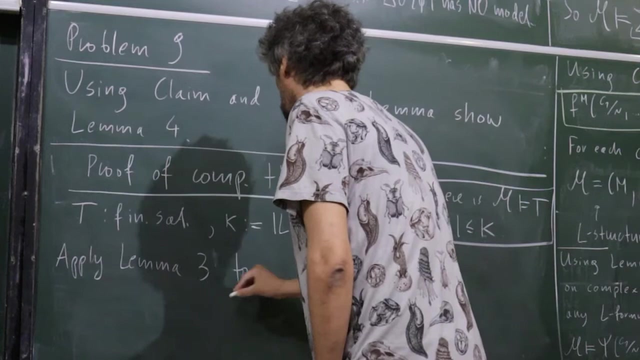 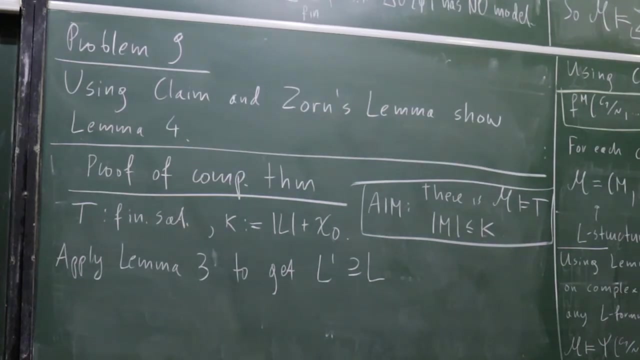 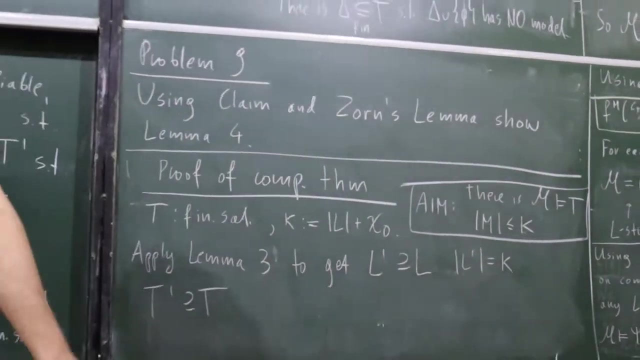 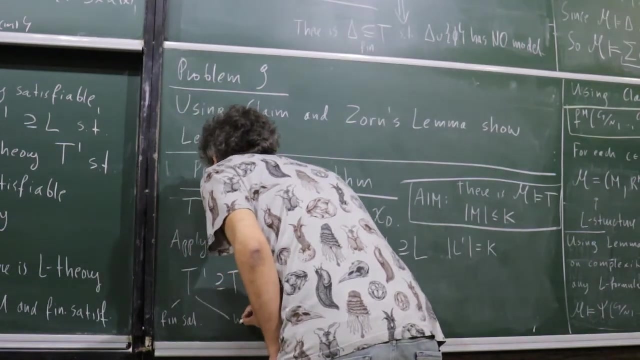 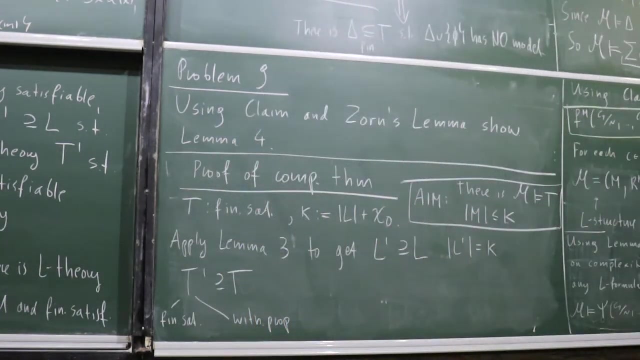 there is model of T of cardinality, at most kappa, so by lemma 3 at yes, as in lemma 3, bigger language, but still okay, l prime actually is kappa and t prime containing T finitely satisfiable with witness property, and to this one we apply lemma 4. so now 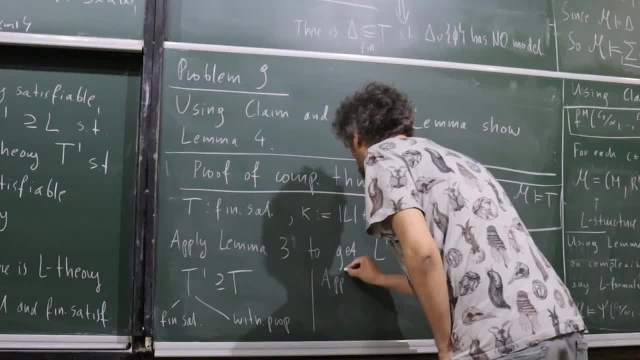 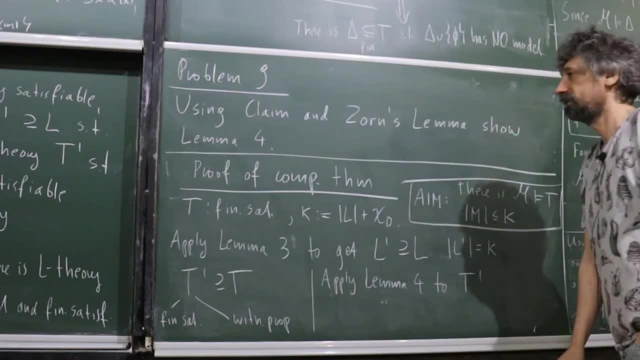 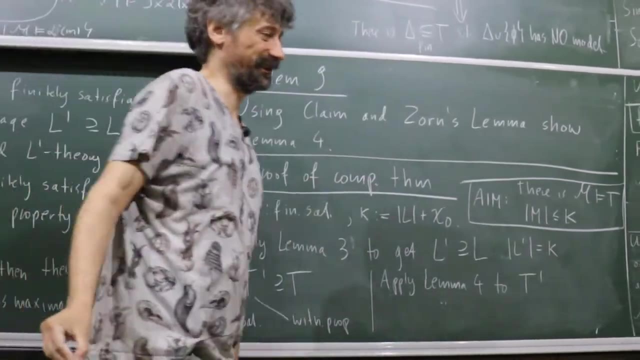 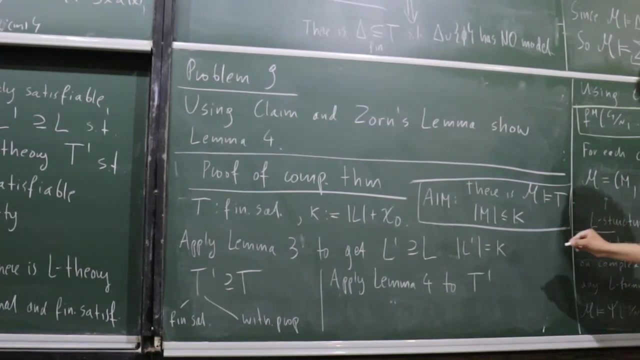 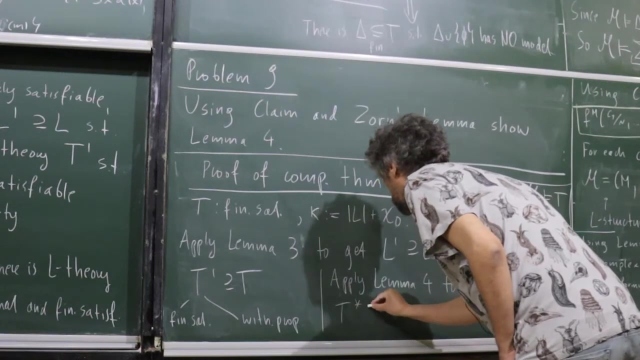 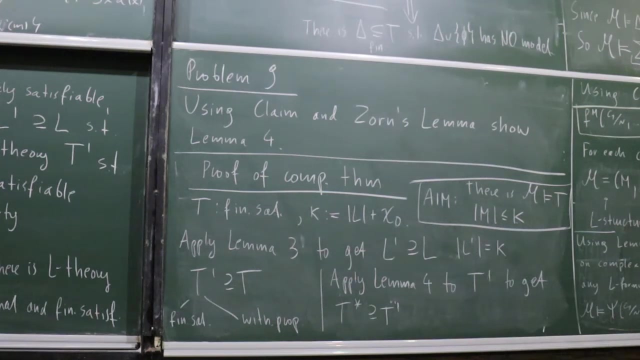 apply lemma 4 to T prime. okay, so in lemma 4 there was no witness property. but witness property cannot be lost in bigger theory. you can notice easily. soon lemma 4 to T prime to get to get, then I think you would lose maximality. okay, I guess you could continue and make some infinite process. 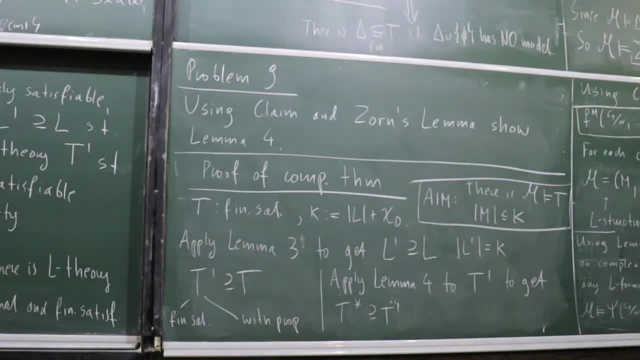 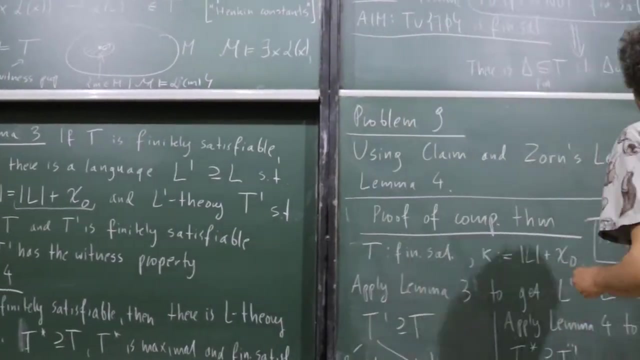 but this is just faster process. I'm not sure, but I think you're using one lemma. I mean, isn't it enough to all this? definitely, if you add all, yes, if you use lemma 3 at this witness property, you lose maximality for sure. okay, because you are looking maximum for l prime. 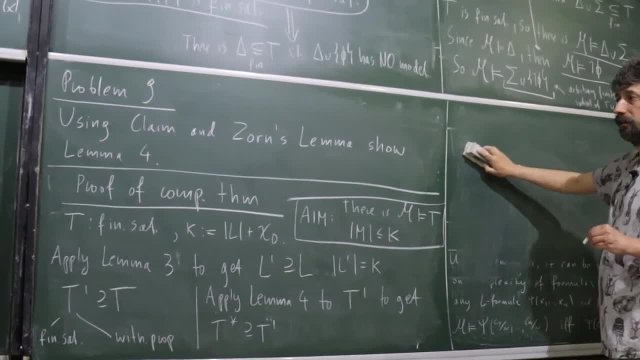 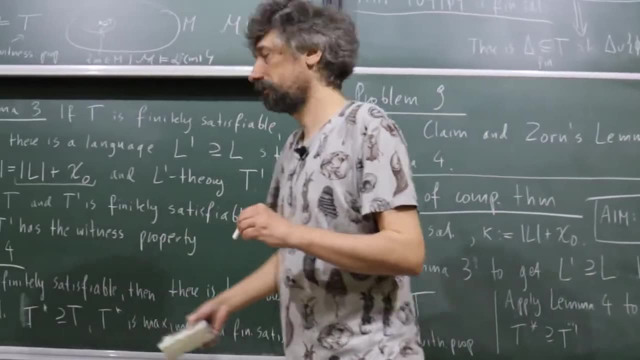 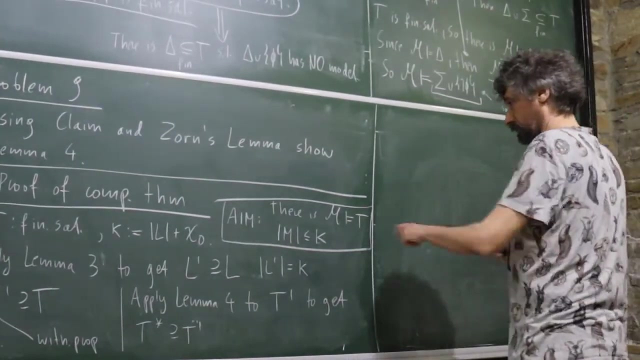 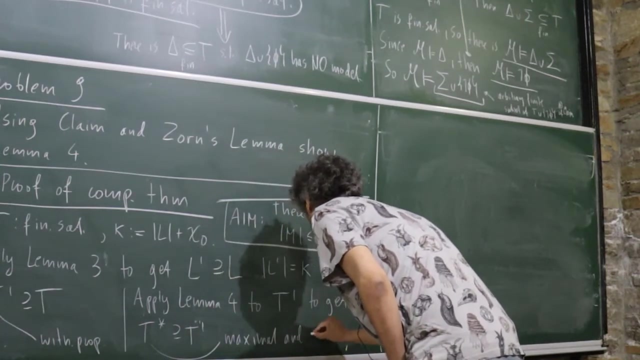 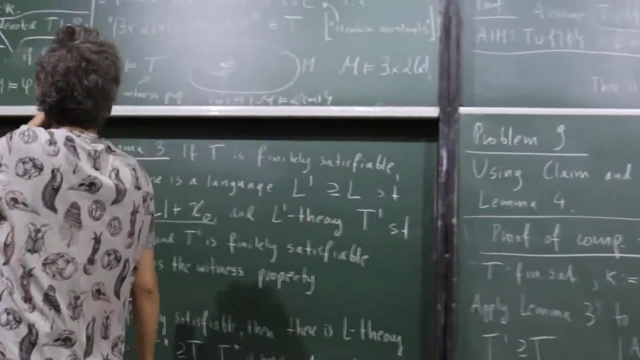 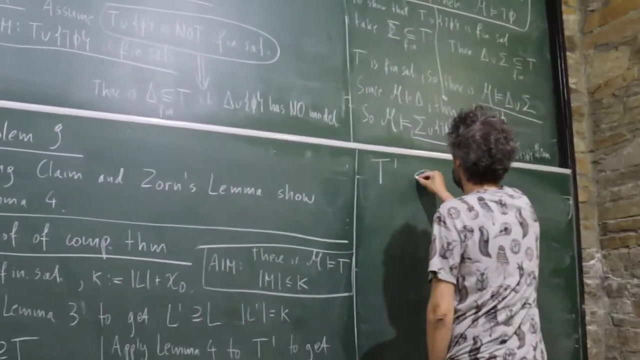 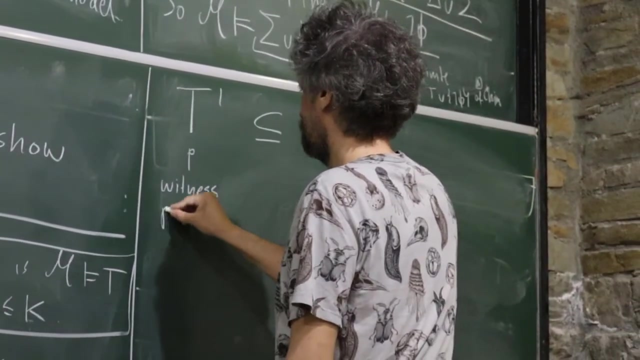 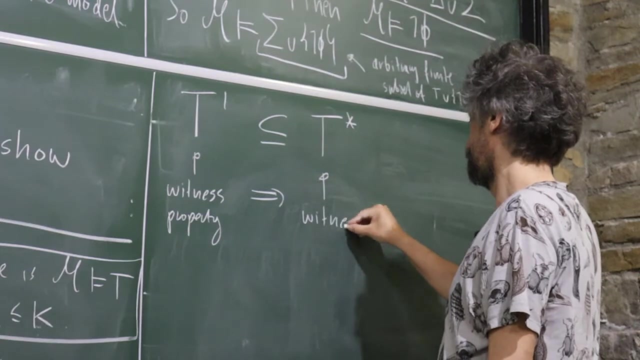 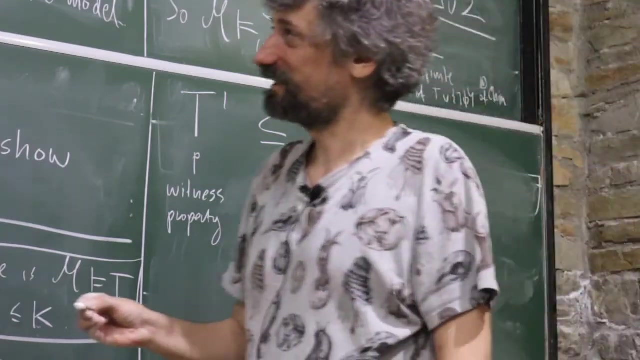 huh, you are looking for maximum for l prime. basically, yes, yes, maximum for l prime, yes, in max. in this part, lemma 4, we don't change language. so which is maximal and finite? okay, but this already. so t prime, this has witness property, so so it's okay. maybe it's late, but this is totally obvious. already all the sentences were in t. 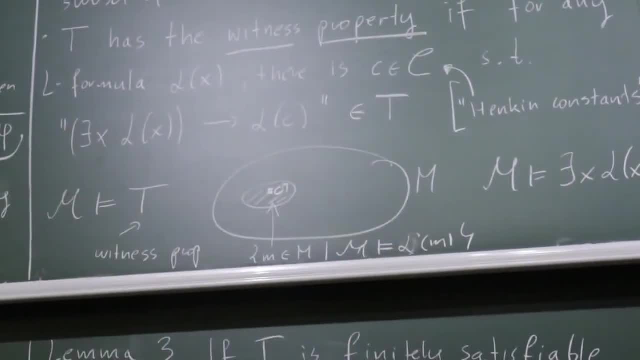 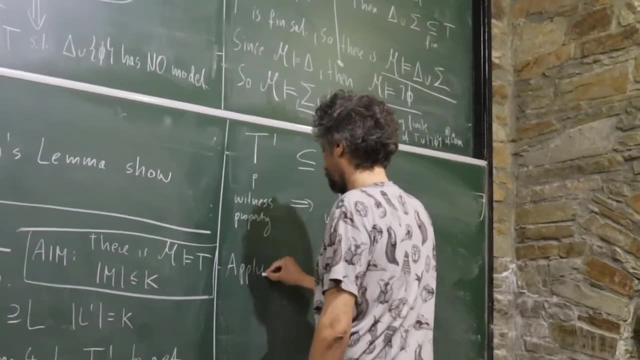 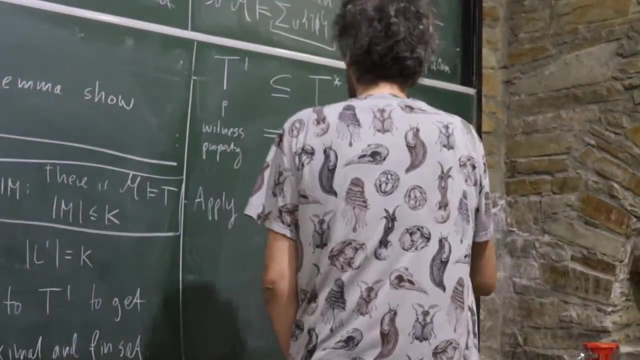 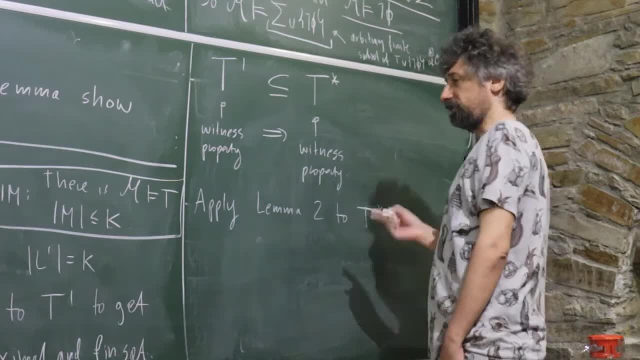 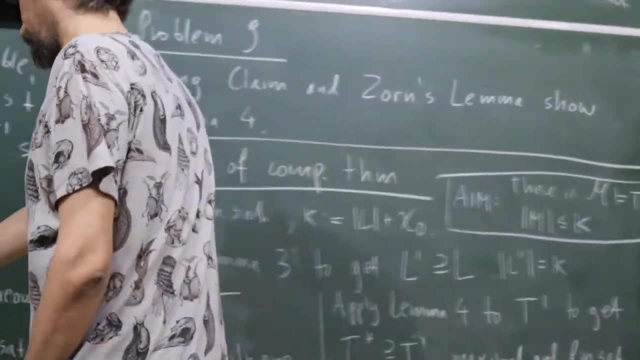 yes, so this t star has all the properties from lemma 2.. okay, as you can see, this kappa was also not lost in this t star process. i didn't put it okay here, but the cardinality also didn't change. i should have said and get. 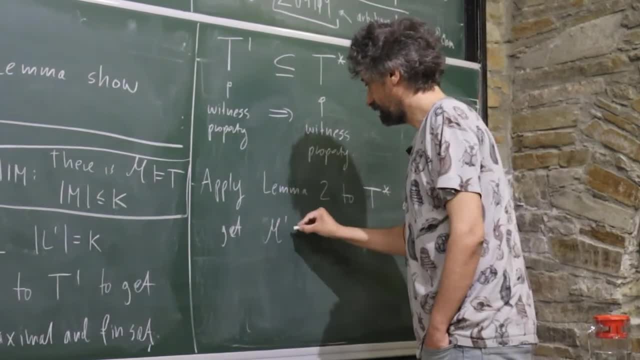 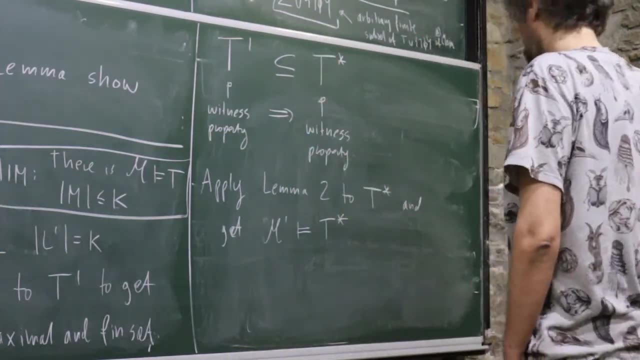 okay, let's say m prime, so it has some more structure. but now, so it has some more structure, but now. so how this m prime looks like so how this m prime looks like so how this m prime looks like it has some universe. it has some universe. 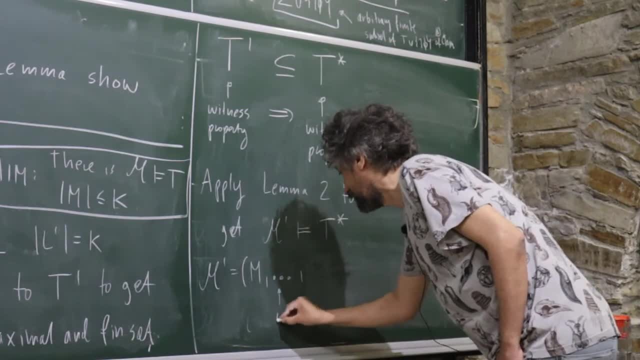 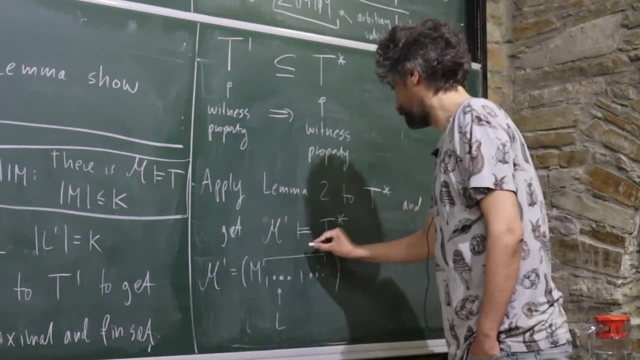 it has some universe. very informally, i say very informally, i say very informally, i say this is in the language l, and then there is the rest, and then there is the rest, and then there is the rest which is in the language l, prime, l prime. 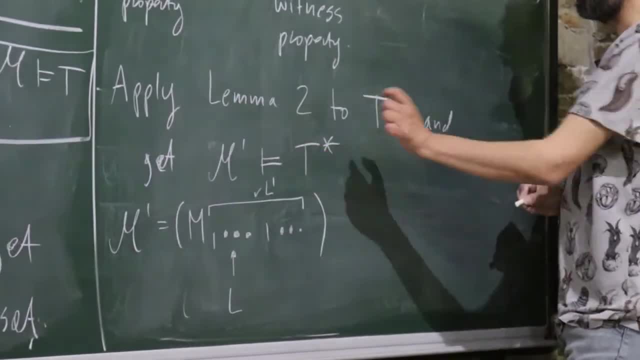 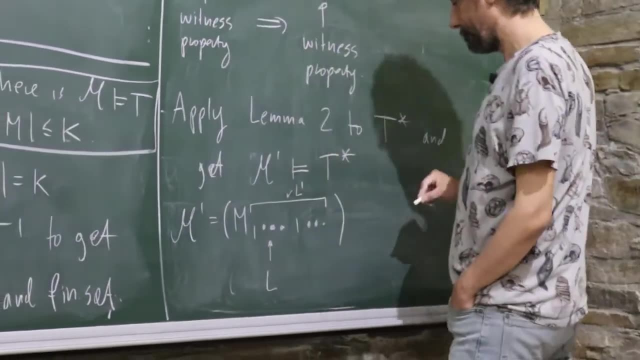 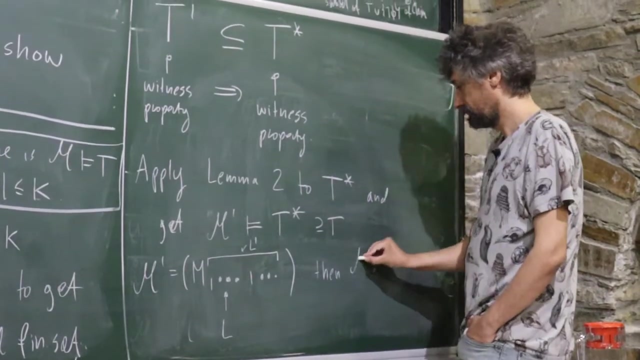 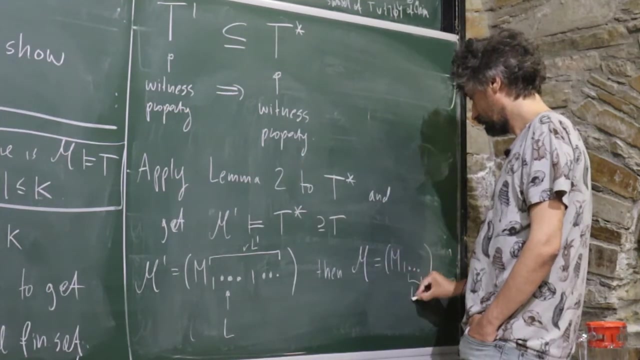 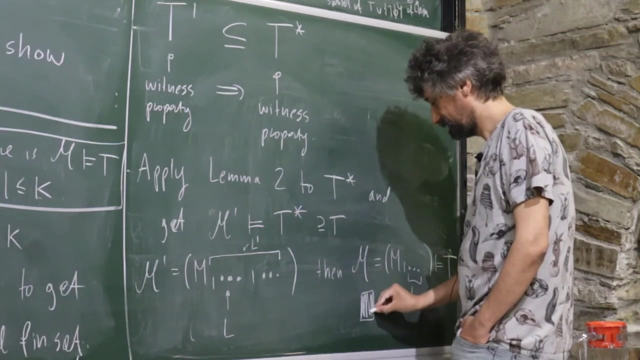 l prime. so if i reduce to this part, so if i reduce to this part, so if i reduce to this part, it would have to be model of t, because it was, because it was, because it was contained there. so that's the end of the whole proof. the last thing. 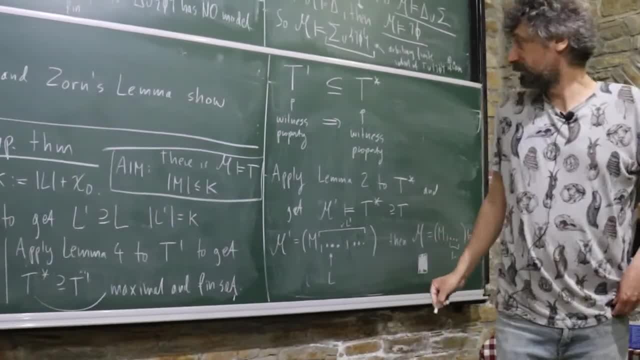 of the whole proof, the last thing of the whole proof, the last thing i may. i may. i may discuss, discuss a bit, okay, maybe still a bit okay, maybe still a bit okay, maybe still so. did you get what i meant at the end i so. did you get what i meant at the end i? 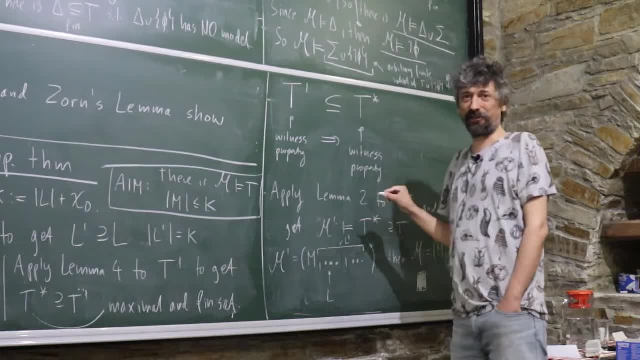 so did you get what i meant? at the end, i got a model, got a model, got a model, but of bigger theory in a bigger language, but of bigger theory in a bigger language, but of bigger theory in a bigger language. so i'm saying, so i'm saying: 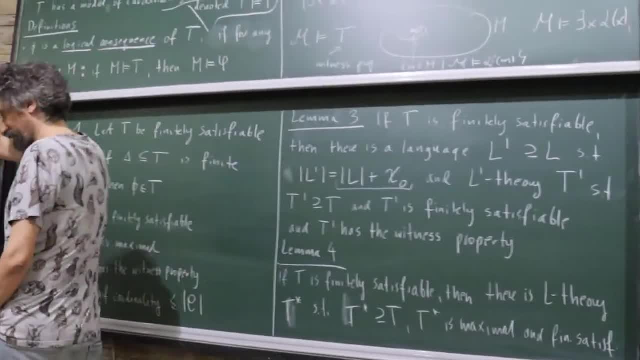 so i'm saying, if i forget about this bigger language, if i forget about this bigger language, if i forget about this bigger language part, i just think in the old language part, i just think in the old language part, i just think in the old language. this is the model of original theory. 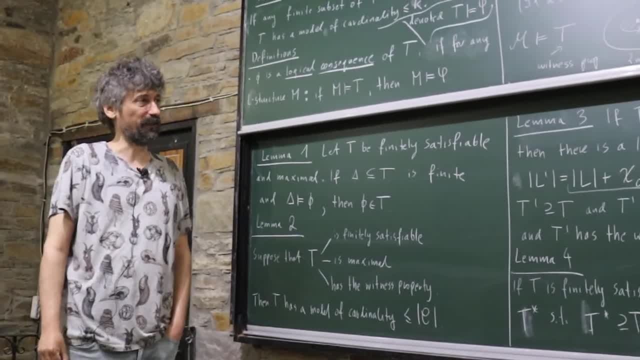 this is the model of original theory. this is the model of original theory, which is, which is? which is kind of obvious if you think about it, so kind of obvious, if you think about it, so kind of obvious, if you think about it, so maybe i will give an example. 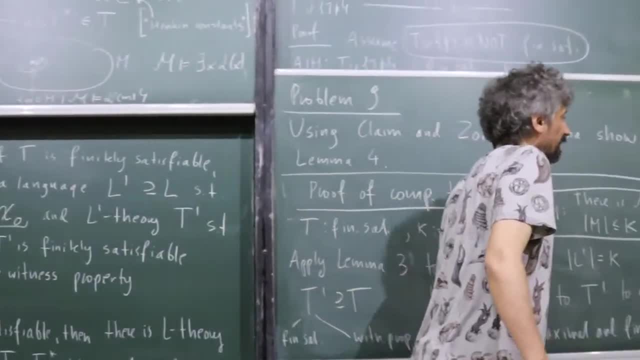 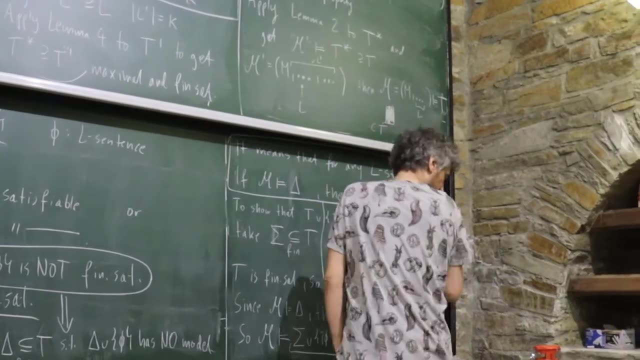 maybe i will give an example. maybe i will give an example for this last moment. so this was end of the proof of. so this was end of the proof of. so this was end of the proof of compactness theorem. so what is the meaning of this last part? 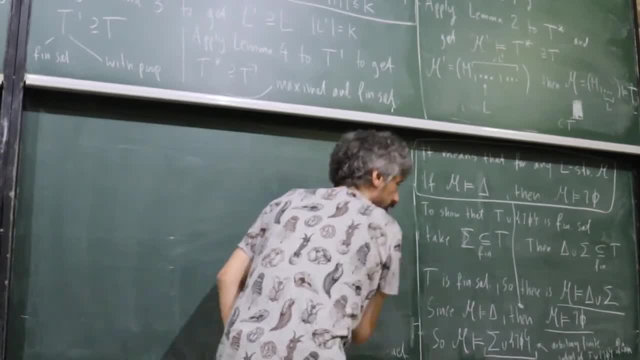 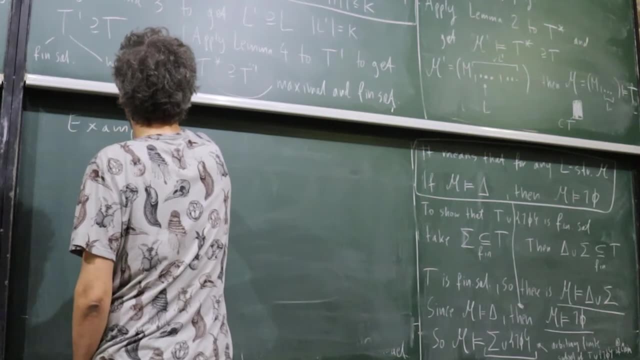 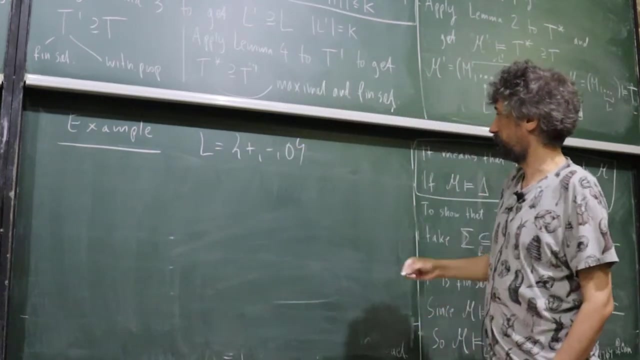 so what is the meaning of this last part? so what is the meaning of this last part? maybe by example, maybe by example. so if l let's say: is this so? if l let's say: is this so, if l let's say: is this language of abelian groups? 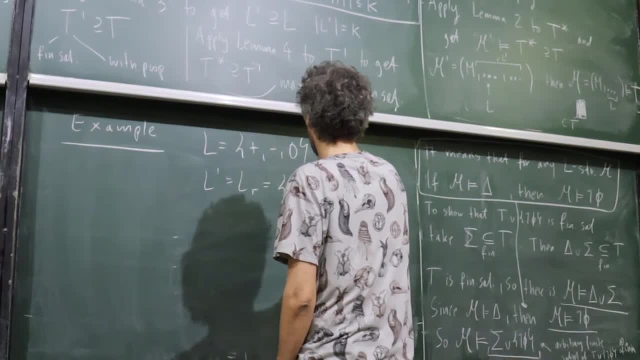 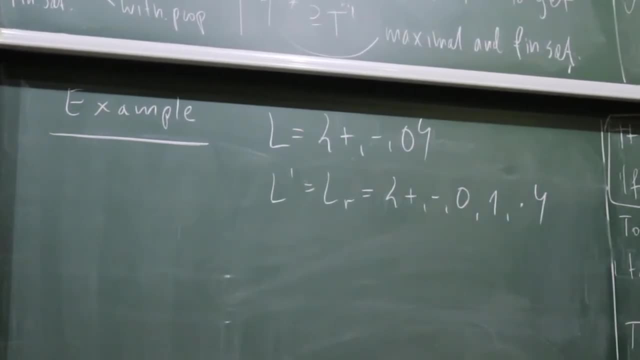 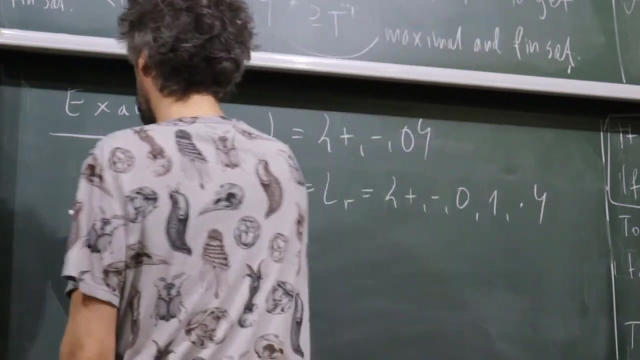 language of abelian groups, language of abelian groups and l prime is the speaker language, then is the speaker language, then is the speaker language. then, okay, if, if i have any sentence, if i have any sentence, if i have any sentence, so let's say i have z.